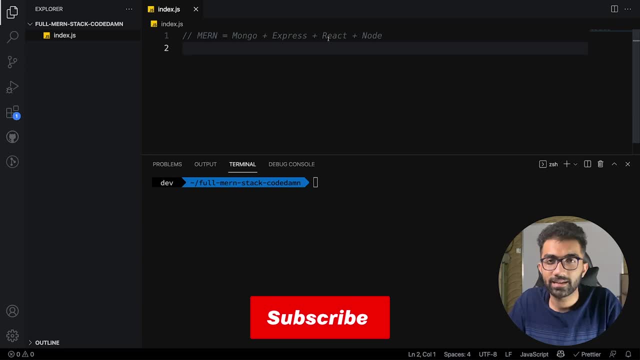 redundant, but it's okay. We'll start with setting up a simple react app, because that can also run standalone. But what you have to remember is when development inside development, you would have a nodejs server plus a react server running right, but when you're 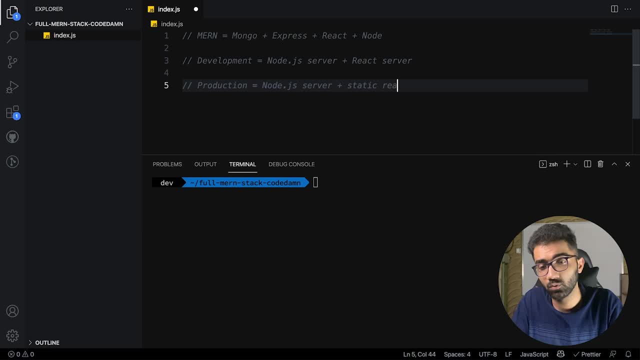 running this in production. you will have a nodejs server, but you will have static react files. that is the difference between development and the production thing, and we will see how we can combine them in the production video and in when we are deploying this on the cloud. but for the development part, let's 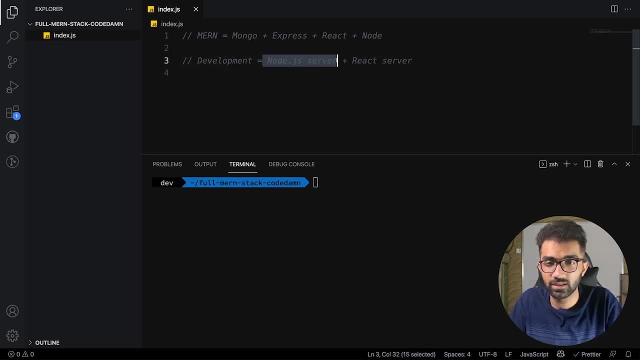 just stick with this setup right here. this means clearly we need two things. the first thing is nodejs server and the second thing is react server or the react project. so what I'm gonna do is I'm gonna go ahead and create a directory here called server, and this will just contain our server stuff and 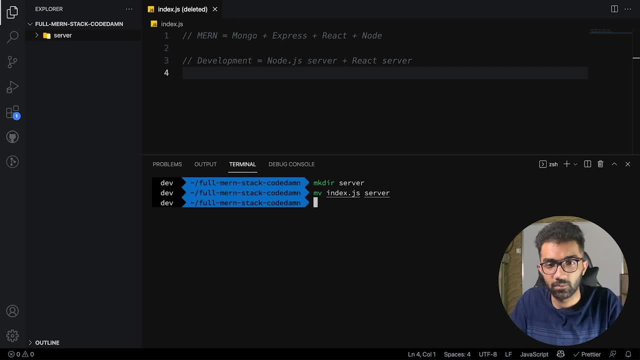 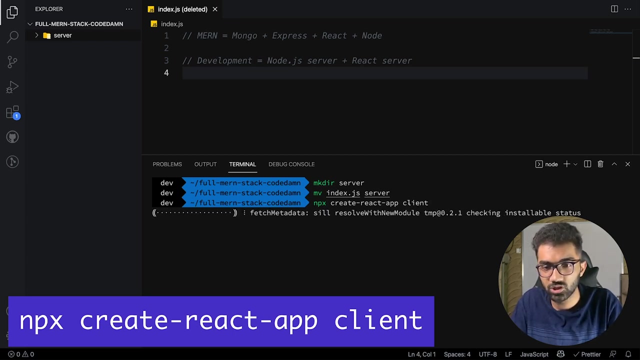 I'm also gonna move this index to server right. I'm gonna create another directory called app or client or whatever you want to name. but we want this to be a react project. so I'm gonna initialize this with npx: create react app and this would be just client right. so this just initializes it with the default react. 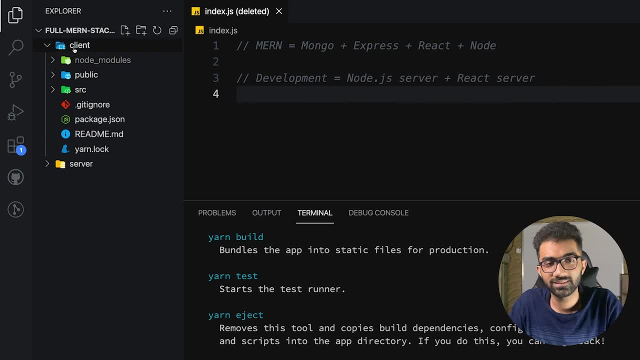 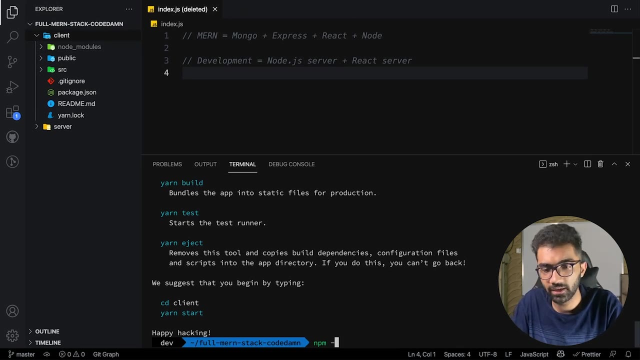 bundle and installing packages and stuff. alright, so let's get started. alright, so you can see, now inside our client folder we have packagejsonyarnlog file, which means we are running yarn as the package manager. if you see a package dash lockjson file, it's completely fine. that means you're using npm. if you write: 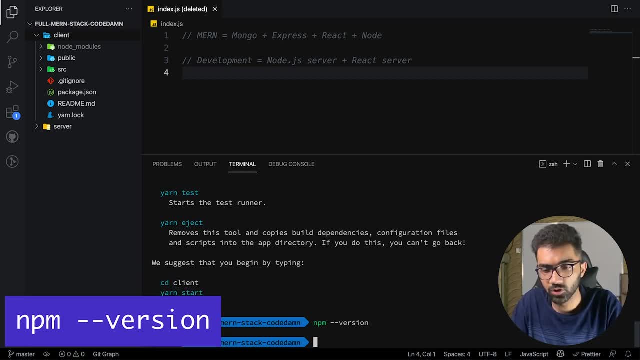 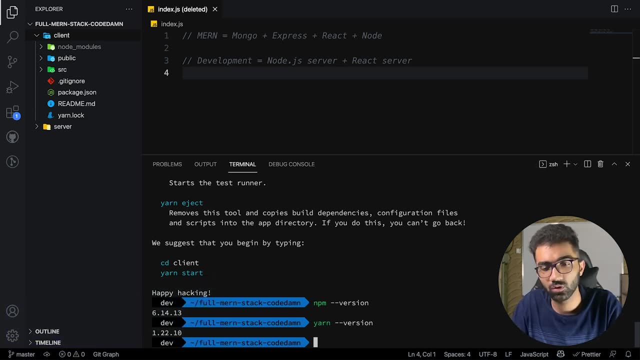 npm. like this in your terminal and do an npm version. if this happens, this appears as six or seven or whatever version you have at the moment. that's fine. if you're using yarn, that is also fine. these are both package managers and at least yarn version one. 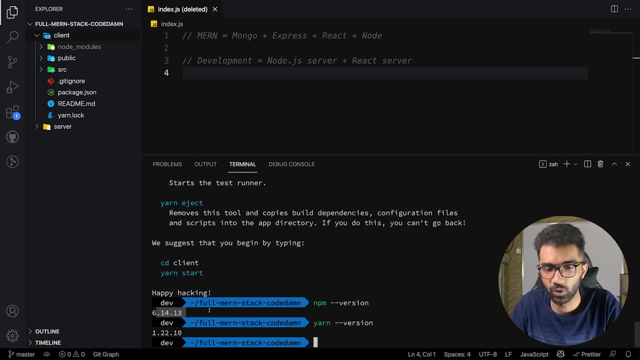 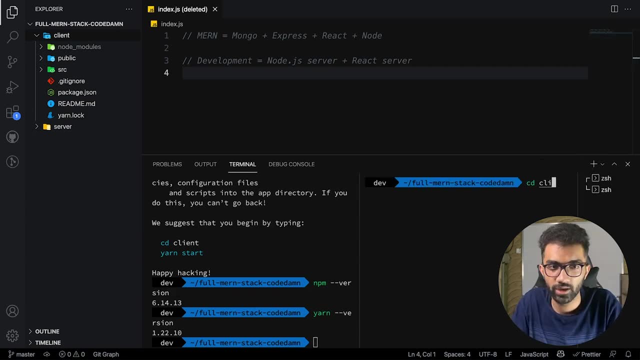 is basically the similar thing as npm version. whatever you're running, six, seven, eight, so we have this client set up. now what I want to do is split my terminal here real quick and I want to go ahead and start this project by saying, yarn, start. because this is gonna start our client project on port number 3000 by 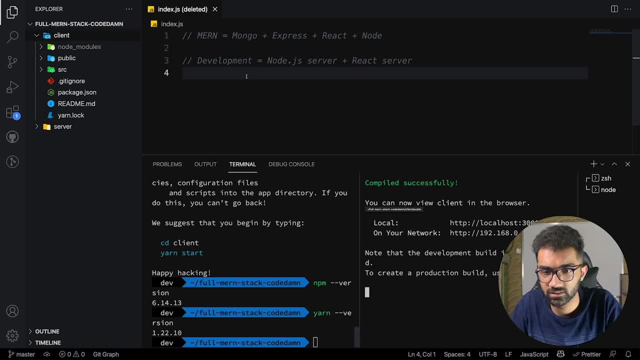 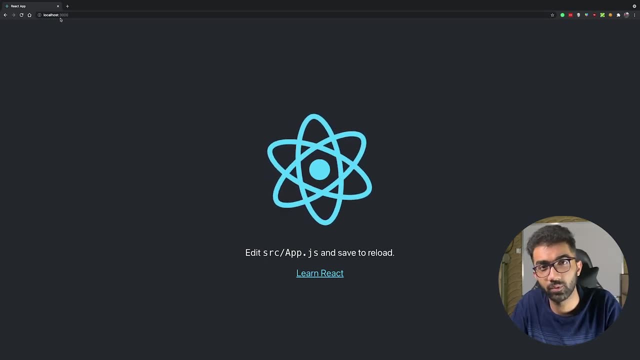 default right. so it opens it up in the browser. it will just compile the stuff, like you know. like I said, this is the react server which I was talking about. when you're doing this on production, when you're deploying this on a real website, you will obviously not have a react server running, because react is. 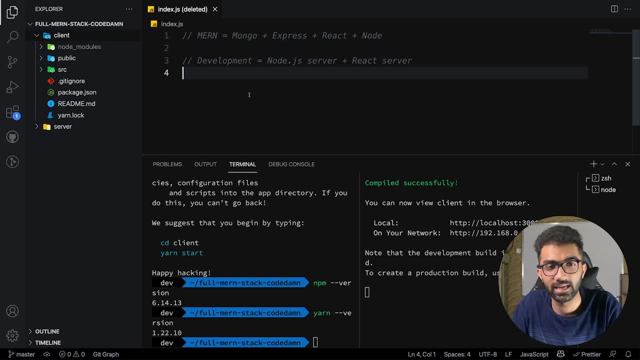 just HTML, CSS and JavaScript. right at the end of the day, react is just JavaScript and the reason you need this server is because react needs a transpilation step. the JSX which you write, the modern JavaScript syntax which you write, that needs a transpilation step. so, babel, webpack, all this stuff is 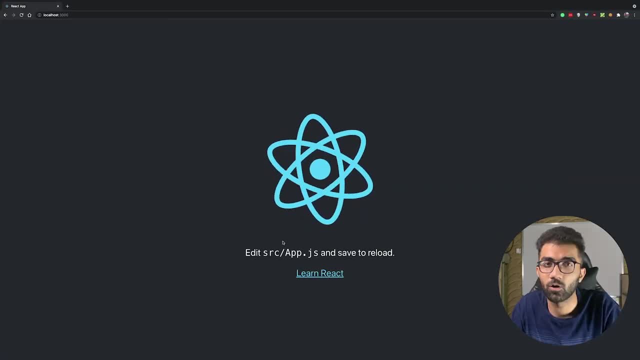 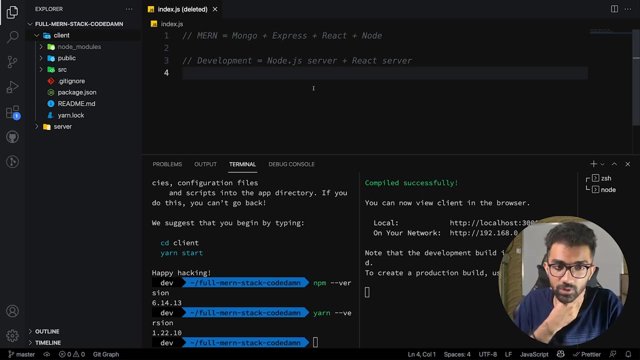 sitting in the server and doing that as you type, like the hot reloading stuff, and without actually refreshing anything, all that stuff happens. but the moment that happens you can see that on the screen and it refreshes and all that things. but you don't necessarily need that on a production server. so anyway, let's just 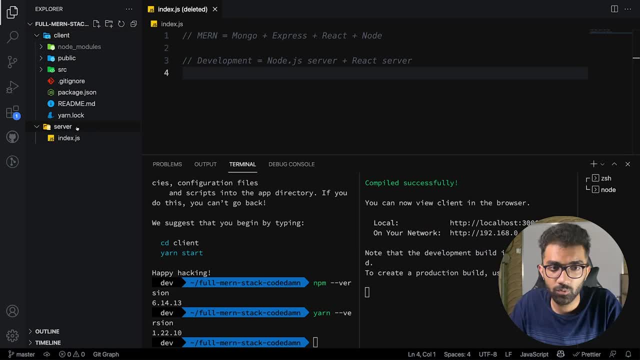 keep going. so we have our react app up and ready. what we want to do next is also have our server- some sort of you know- in place. so of the mon stack, we have already covered the R part, so it's the main type, and so let's just go ahead and 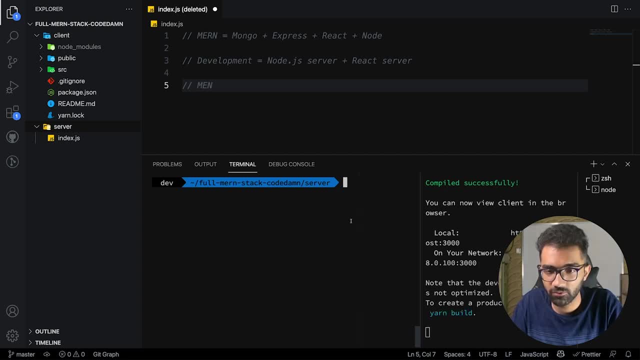 start with our main time, which is basically gonna be very simple. first of all, we need to initialize the project, because this is a node project, so we can just say yarn init. if you are using npm, you can say npm init. I'm just gonna keep the default options. you can also specify a dash Y here, but anyway, now you 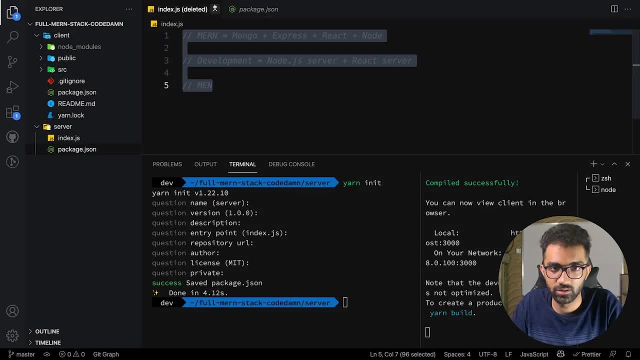 can see, we also have a packagejson file here, and let me just actually copy this whole thing and save it inside here. alright, so you can see, we basically have node installed on our system. right, I did not talk about that because I was assuming that everyone has node installed, but if you don't have it, I 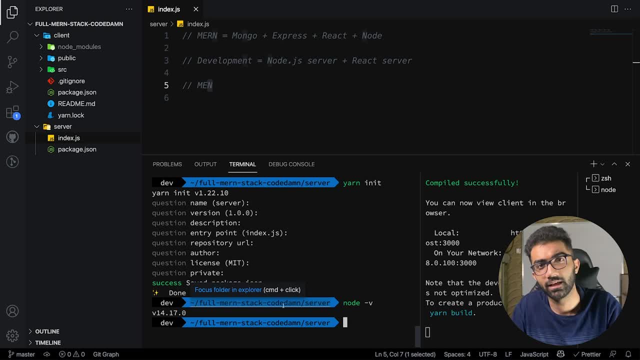 have a bunch of videos- probably I will link it somewhere here in the cards at the top right or left- showing you how you can install nodejs. but once we have done that, you will be able to see that it's very easy to set up a project. 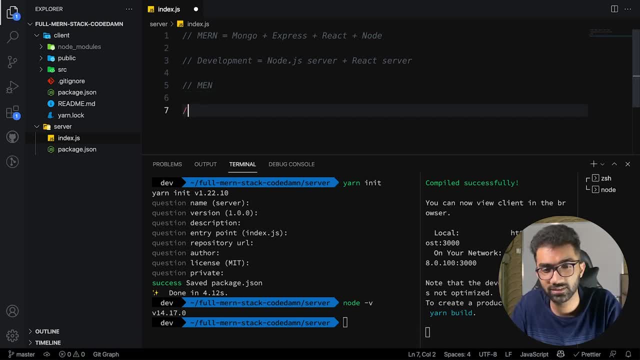 now the next thing you need to do is install Express. now, Express is a framework- E stands for Express and Express is just a nodejs framework which allows your application, the server application, to have easier looking syntax, and you can see that it's very easy to set up a project and it's very easy to 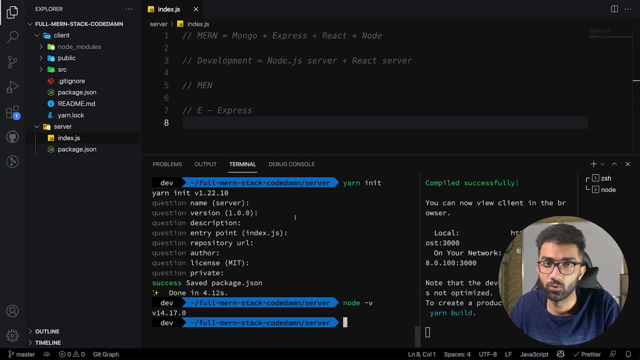 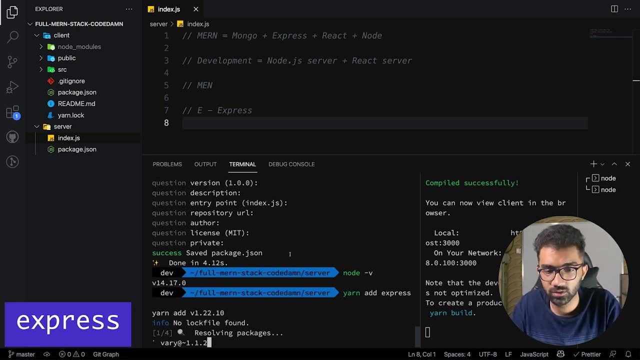 I mean, you can technically still do all of the stuff we do in Express in node, but it's just easy on ice, right? it's easy to do. so let's just start with yarn again yarn add Express, and what this will do is this will install the Expressjs. 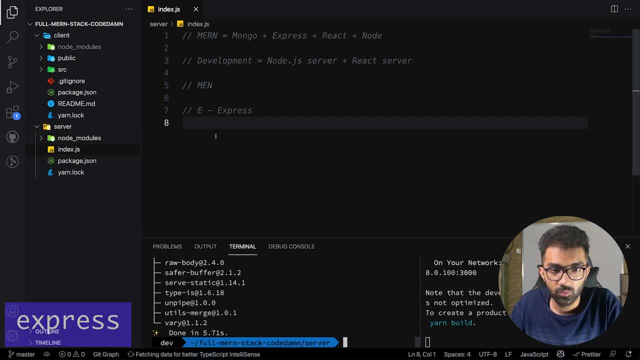 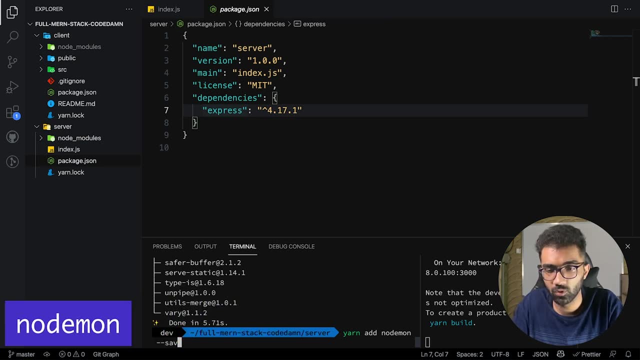 package inside of our server folder. okay, so the moment we do that, you're gonna be seeing that inside packagejson we have this, but we're gonna be adding another server called yarn, add nodemod. so just like you can see that, we have react server running which will reflect, let's say, if I go to this, 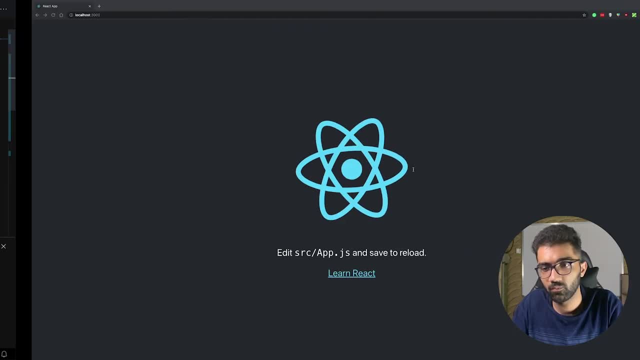 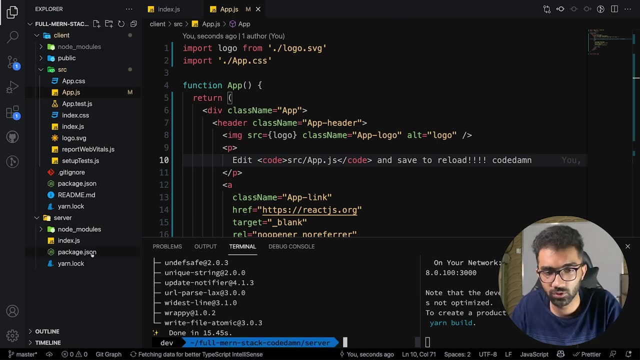 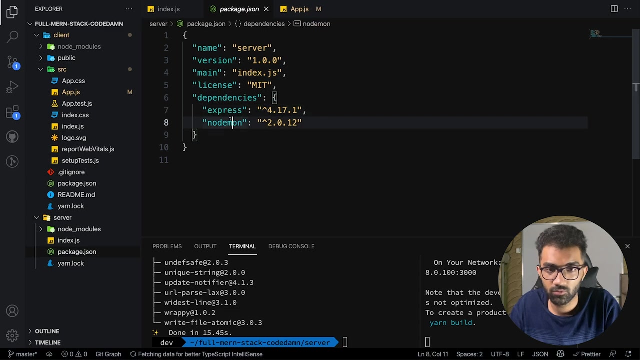 appjsx and say: go damn right here and take a look, you can see, it updates automatically, right? similarly, we can do a similar thing with servers using nodemon, where nodemon would just restart the nodejs process if there is any change. okay, so now you can see. we also have nodemon installed and what I'm 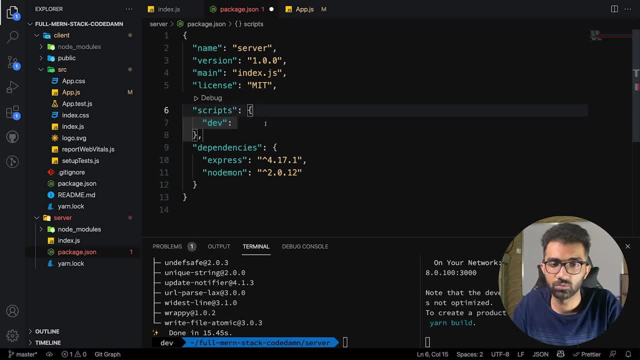 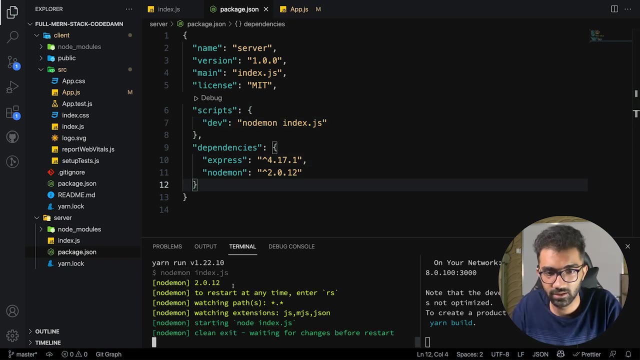 gonna do more is I'm gonna add a script here called dev. so this script just means that whenever I write yarn dev or npx dev or npm run dev. this should happen. what is that? that is nodemon indexjs, right. write yarn dev and you can see it runs. nodemon indexjs, clean exit. waiting for changes. 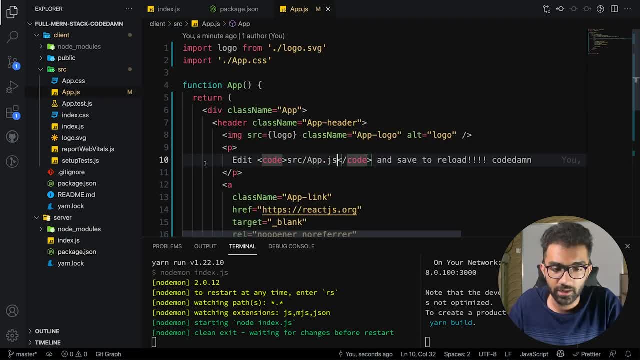 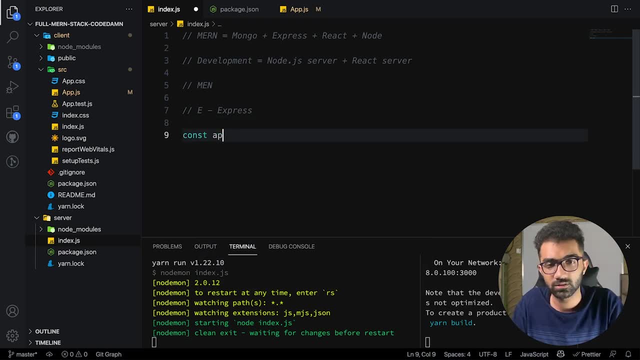 before restart, because obviously there is no change yet. let's just go ahead now and take a look at how we can write our Express server real quick. I'm gonna go ahead and say const app or const Express. this will require Express and once you have Express you need to call this as a function to actually initialize a new. 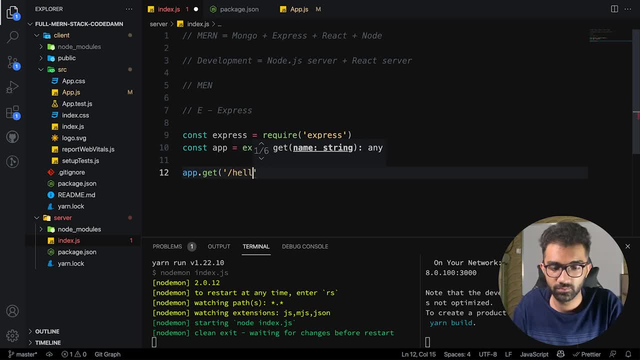 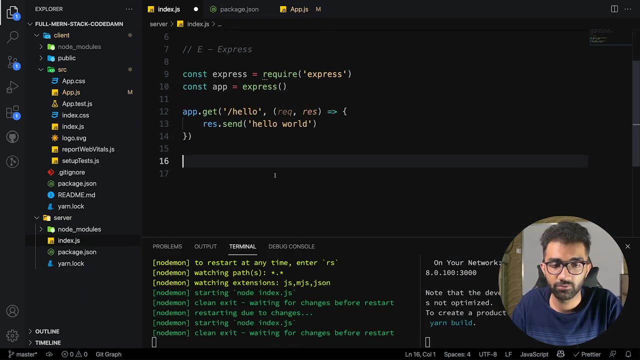 application. then you can specify some routes, like hello, for example, and this accepts a request and a response object which can be used to determine what headers the client has passed or what you want to say to client. in this case, I'm just gonna say hello, world, like this, right. and the final thing you need to do, 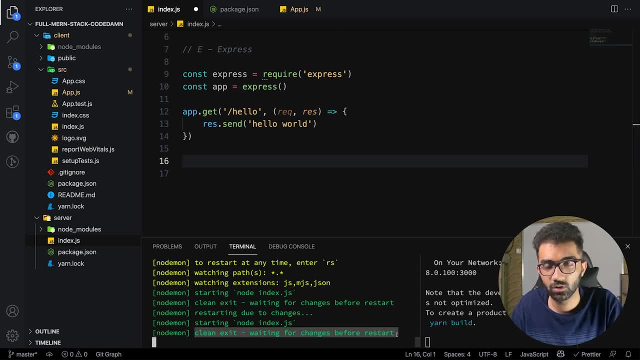 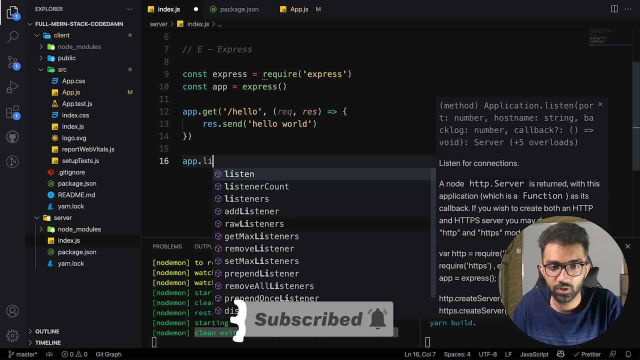 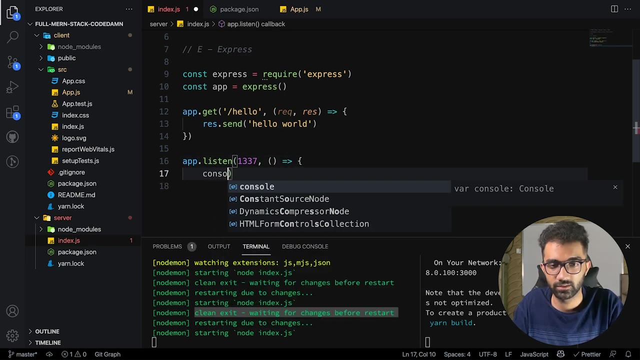 is also start a server, because right now you can see nodemon just runs your node file and exits because there is no long running process and servers are long running process. so what do you want to do is say applisten. and let's say: I want to listen to port number 1, 2, 3, 7, right. and we can also say something like: 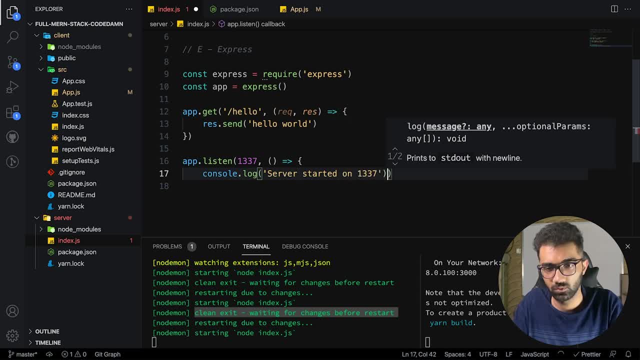 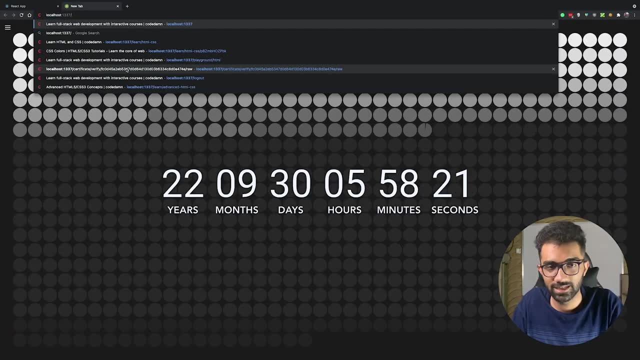 consolelog server started on 1, 2, 3, 7 right. just just a quick notice which you can see in the console now. what you can see is if you go to localhost- 1, 3, 3, 7, slash, let's say hello, which which is our defined route, you can see we get hello world now. 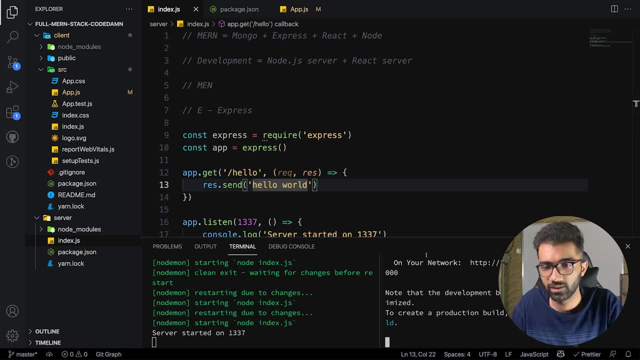 remember, we have two servers running at the moment. the first one is the react server, which is a fake server because we don't need this in production, and the second one is the node server, which we will need in the production right, but for now we will develop it as if we are having two different servers. 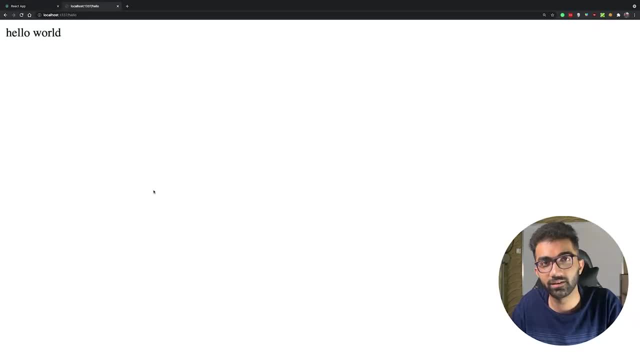 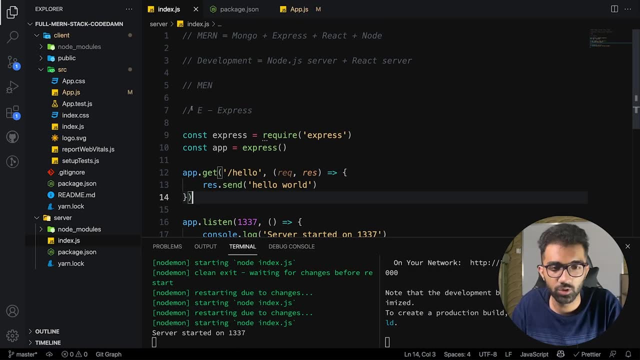 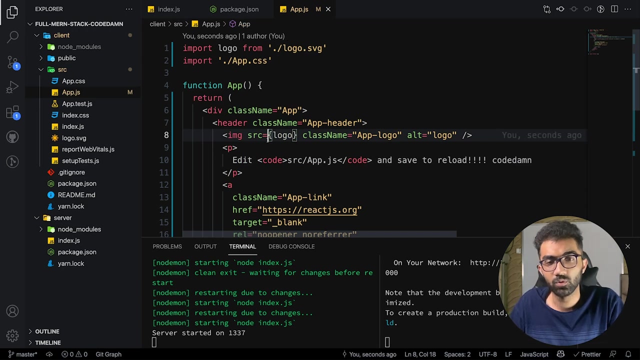 right in production. probably this page would be served right here automatically. right? you can do that still, even in this phase, but it will require a lot of patching and you will lose a bunch of features like hot reloading and stuff like that. all right, let's just go ahead and create a very simple app which has 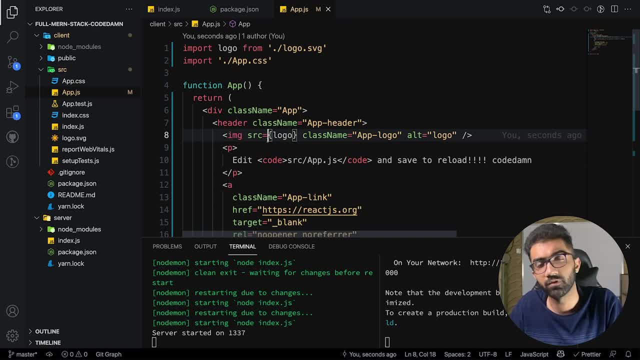 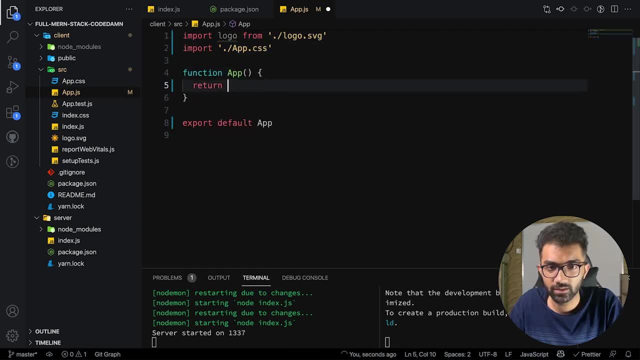 handles login, registration and setting up a favorite code inside the dashboard. right that? that's all that will be. so what we want to do first things first is we want to go ahead and clean up this mess right here and let's say: this is just registration area for us, right? so? 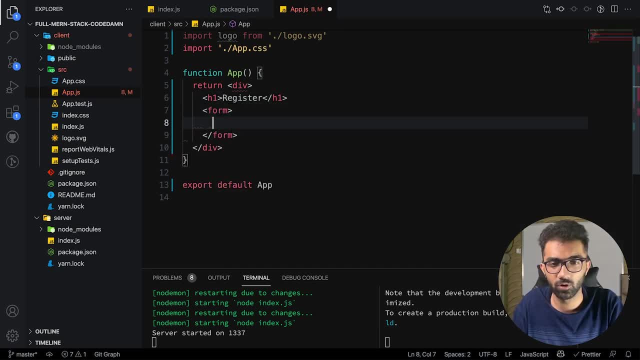 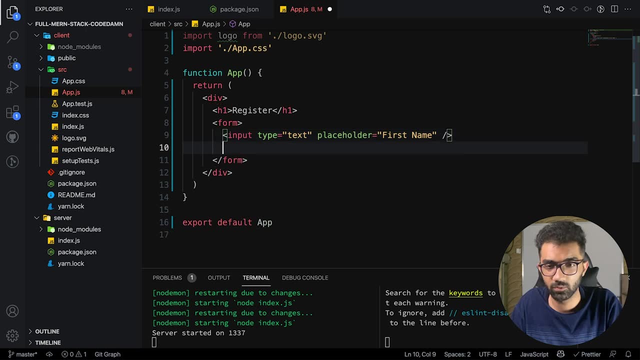 I'm gonna say h1 register and I'm not gonna focus at all on the layout or the CSS part, because the monstag actually we just want to cover how the code functionality works and you know, GitHub copilot can be really, really helpful here. let's see if it can help. first name: no, I don't want a lot of. 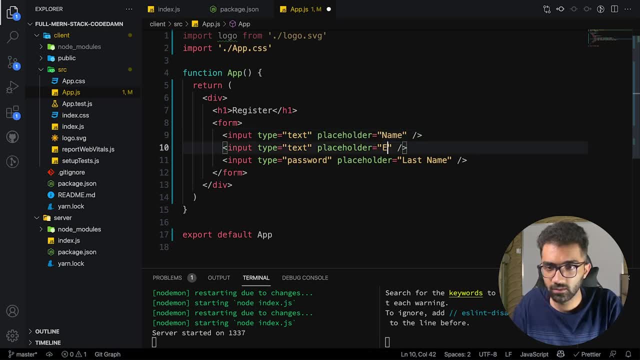 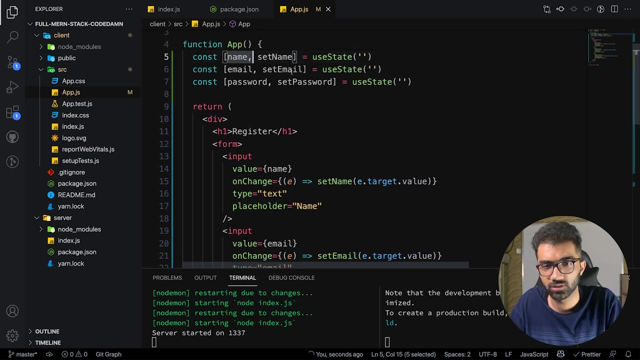 stuff. so we can just stick to maybe name, email and password, right, and what you want to do is really create them as state variables, all right. so now you can see I imported use state from here and set up the basic boilerplate template, which is just having these variables as the state. 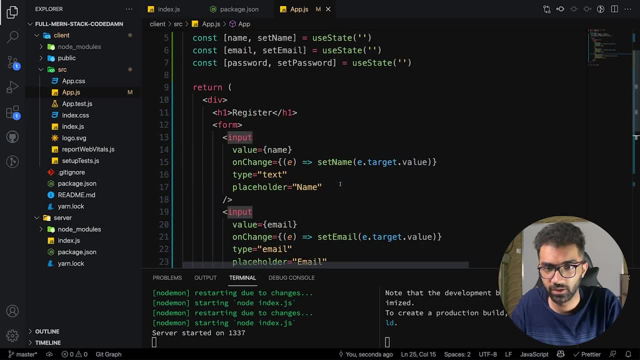 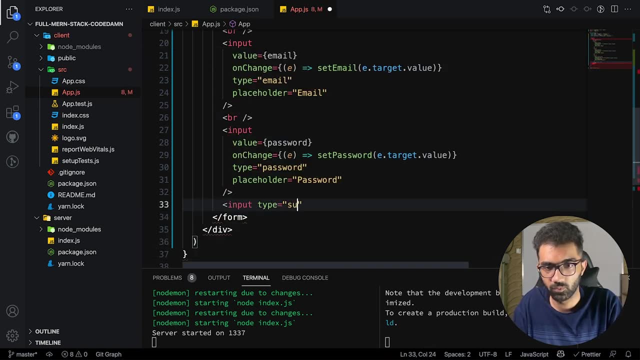 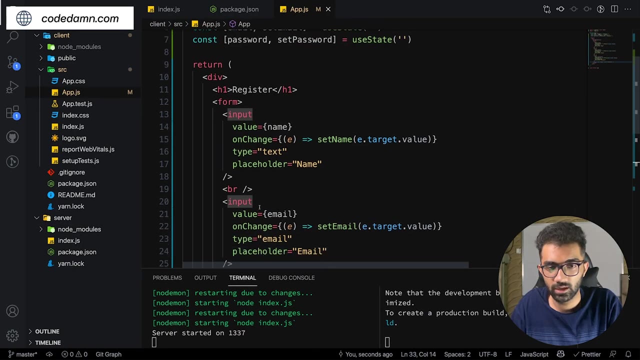 thing as these things, and you can see now this works absolutely fine, right, we have a pretty much working form and you can just inject a bunch of HTML here if you would like, and a final button so you can say input type, Summit, and then value register, and that's it. now you can see that we. 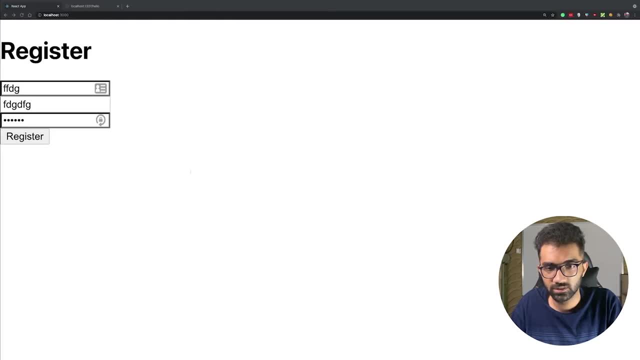 have. let's just go ahead and also get this a VR. but you can see that we have this as a form. so whenever I summit this, I mean after having the right data, you can see it redirects me to a page. so in order to change that behavior, we'll have a method of. we don't exactly need a. 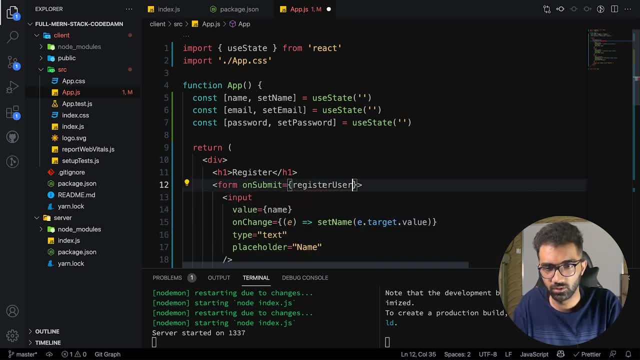 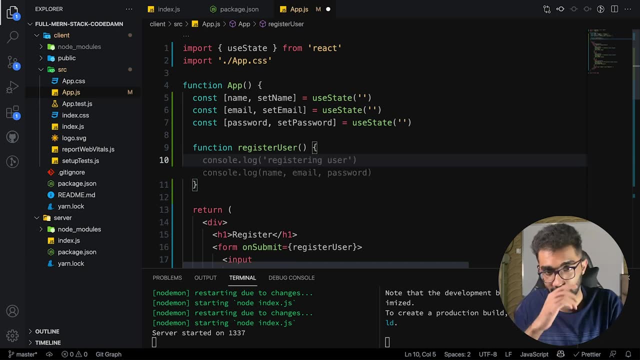 method. we can just say on Summit, and we can specify register user now, right here. this is the very first point when our front end is going to communicate with the back end, right, and we can make this an asynchronous function, and what we want to do is we want to say that hey, go ahead. 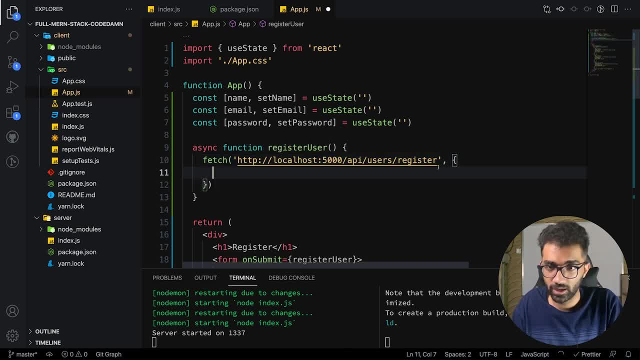 and fetch something like this, which called your dub copilot, is helping me already with. so this is localhost 1337, remember, because we are running this on port number 1337 and we're going to have an API register route. let's see where what we're. 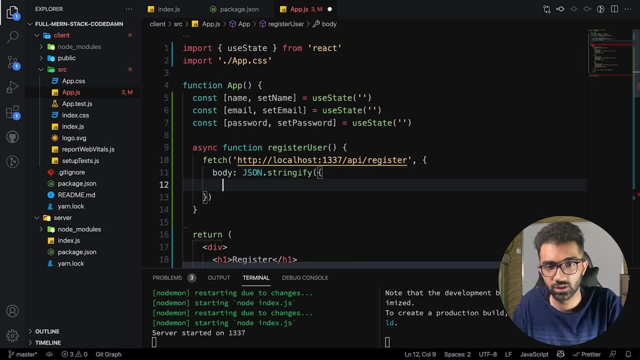 going to do is pass the body as the following: object: jsonstringify name, email and password- right, so once we do that, you're going to be seeing that we just send this to the back end. but we also need to tell the back end that, hey, we are going to send this as a content type of. 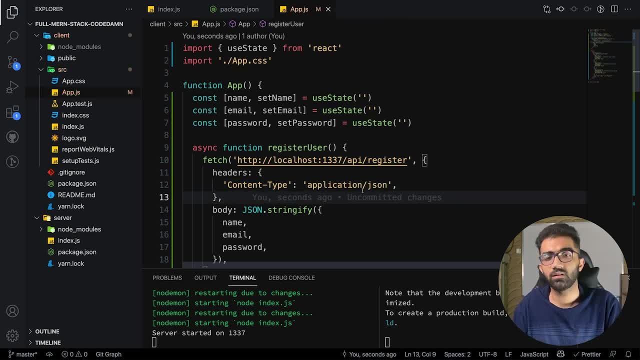 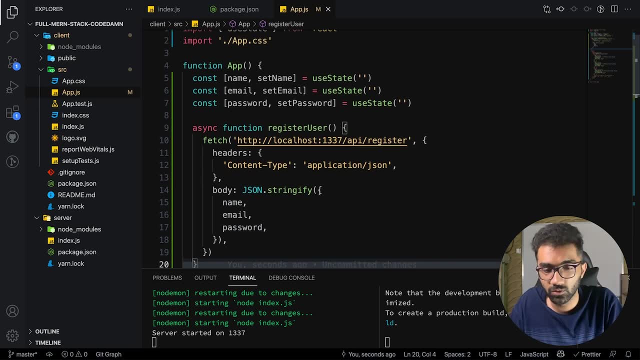 application json and why that is necessary. that is necessary because there are a lot of content types and we can send this in a bunch of ways. you can send this as a binary data, you can send this as URL encoded and stuff like this, but the simplest is for text-based data. at least is json okay. so 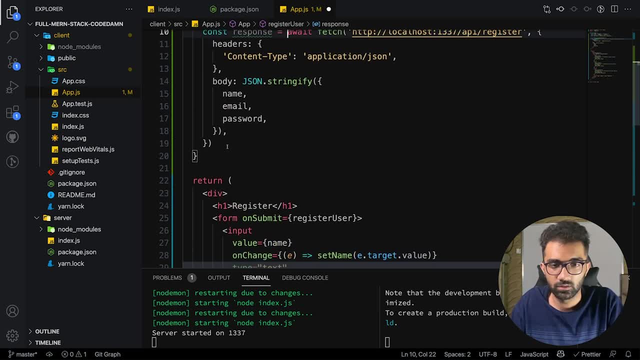 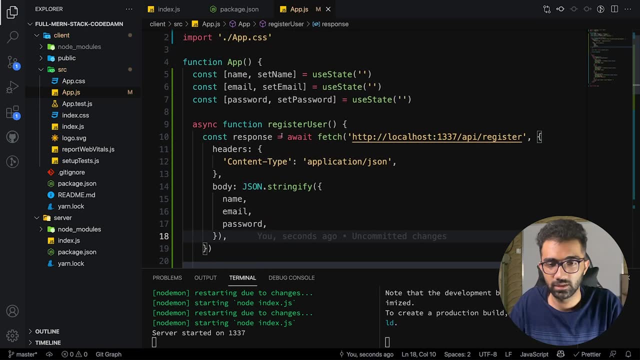 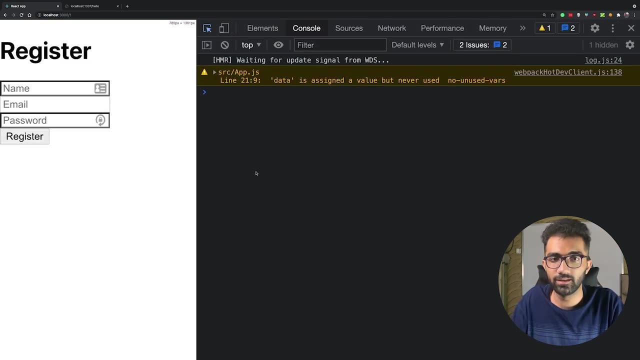 I'm going to go ahead and wait for the response, and then we are also going to try to convert it into json like this, and I'm just going to console log this data right here, right? so this actually ends our first part, in which we just have to go ahead and create a link between: 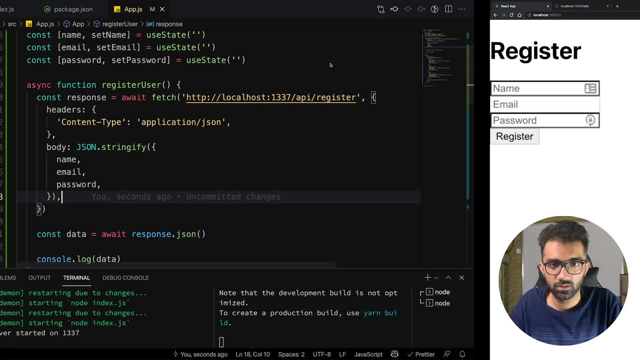 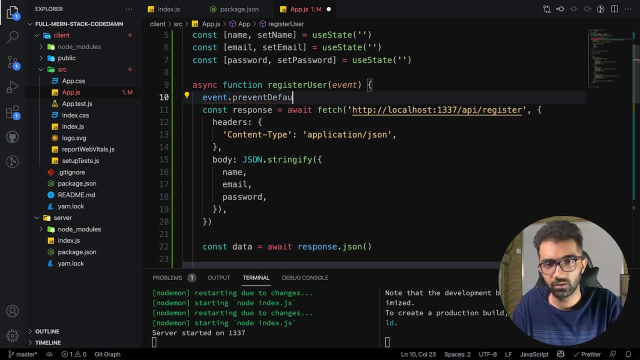 the front end and the back end. so now, if I have something like this register- and of course we need to do one more thing- is the event which we get here. we need to set eventrevent default. why do we need to do this? because right here you can see forms have a default behavior of refreshing. 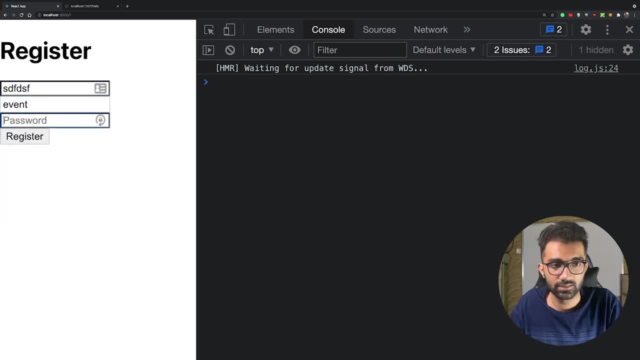 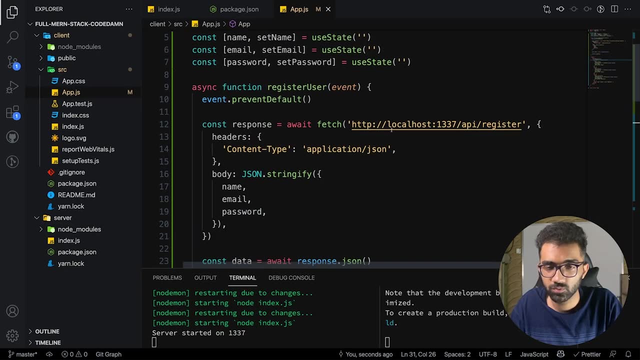 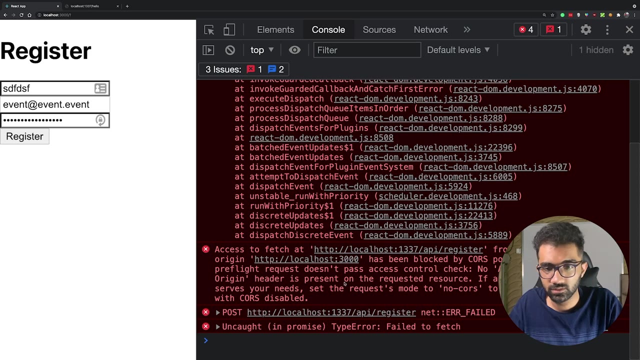 or redirecting to that particular page which you have specified as an action. let's say, this is our email register and you can see that we get failed to fetch because again we are missing one thing, that we need a method here of post register again. and you can see now we get standard errors which 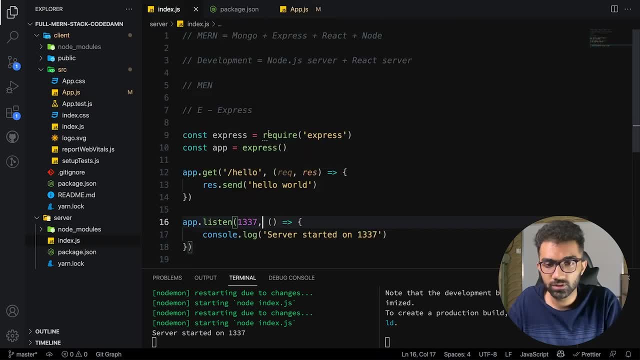 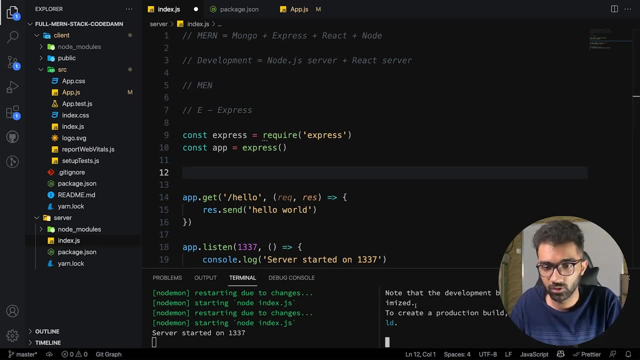 is fine, we'll fix this in server now. all right, so the first thing we need to do here is gonna be actually setting up our course policy for the local development part. I mean, you can do it for local itself, it's fine, but what you want to do is first of all terminate your server and install a. 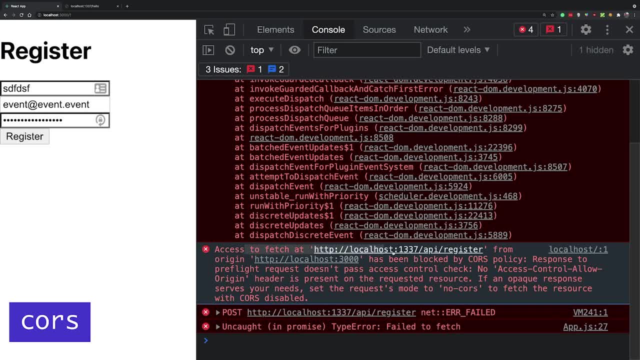 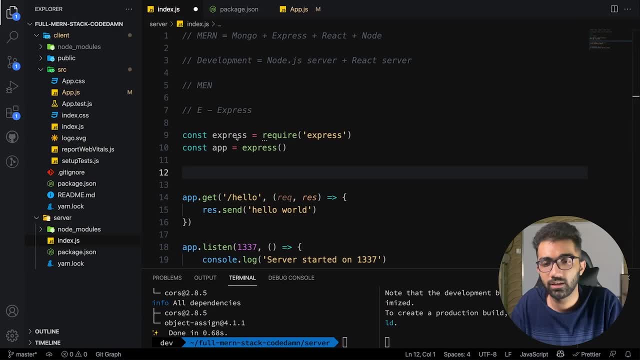 course and the reason you want to add course package is because you see this error. access to fetch at this from origin. this has been blocked by course policy, right? so you're gonna. you're gonna have this error anyway, even if you create your server, if you don't have the correct course. 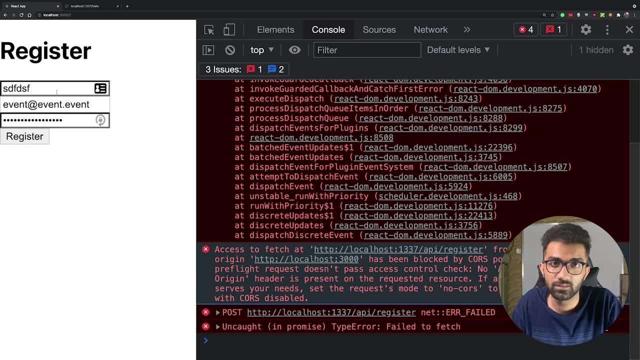 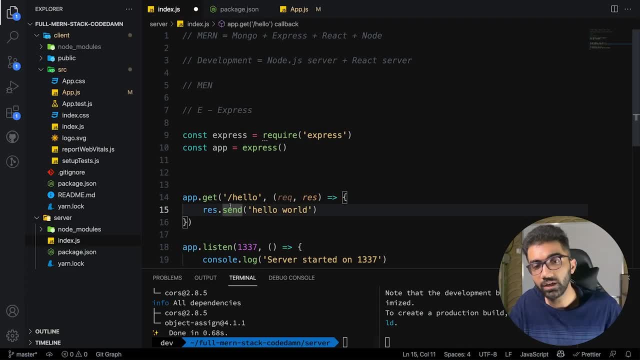 configuration. now, remember that this page, ideally, this react page ideally, would be served by the nodejs: same port itself, right, the same server, the same port itself. so you probably don't need course on production, but that is required when you're developing, at least because browser is not required to do that, because the browser is not required to do that, because browser. 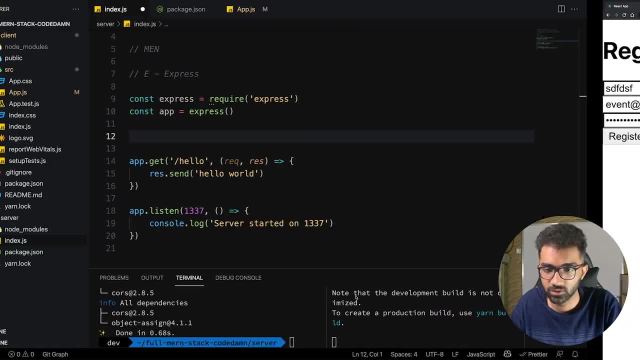 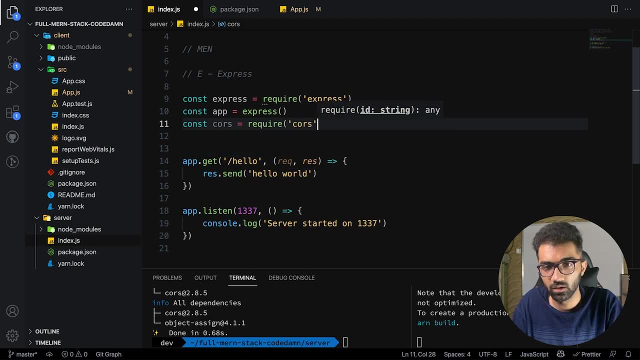 are weird and they require all sorts of security measures, and course is one of the security measures, right? so you need to do that. so once you have that, you just have to import it via require course and just say that this course is a middleware. now, middleware is just a function which manipulates. 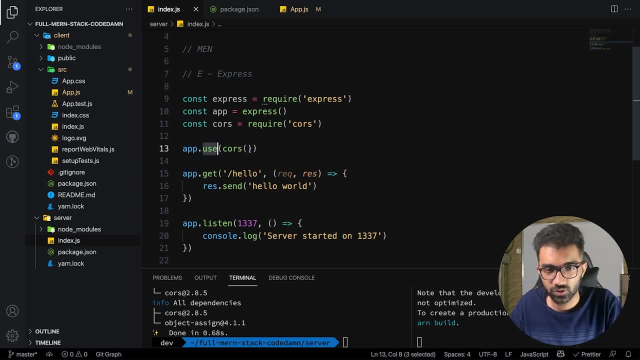 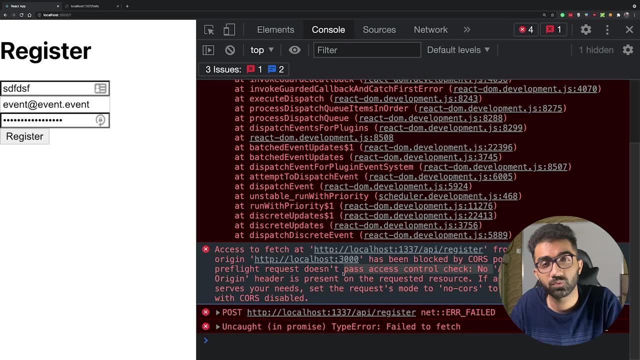 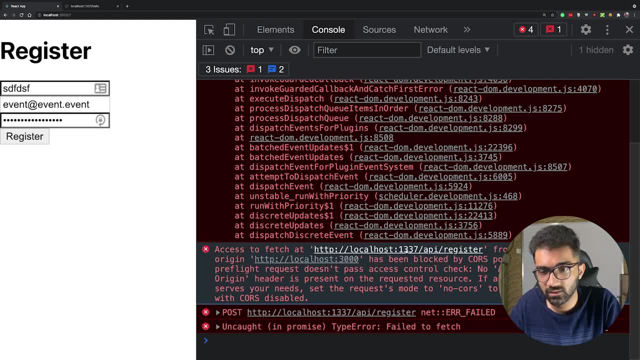 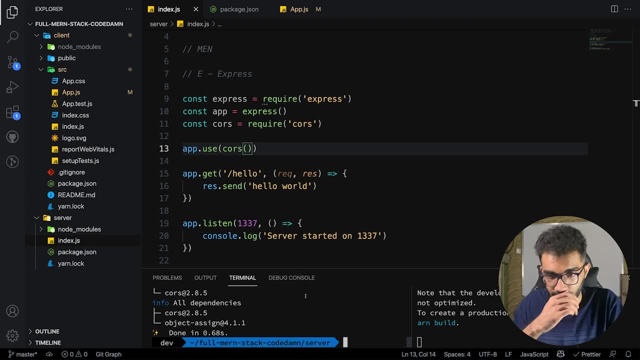 allows you to communicate with a cross origin, and why this is a cross origin? because of the different ports, right, if they were all the same ports- localhost 1337- then it will not be a cross origin. so that is fine. let's just start our server again by: let's say: nope, yarn dev, right. so once we 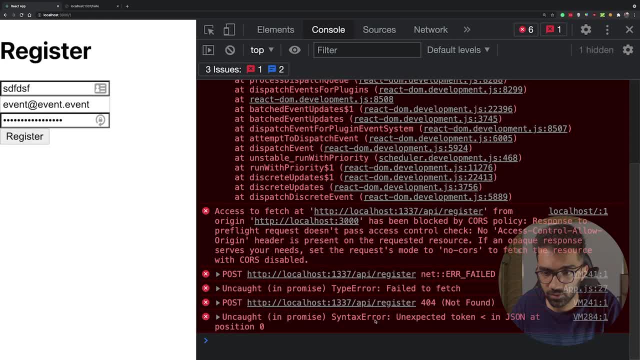 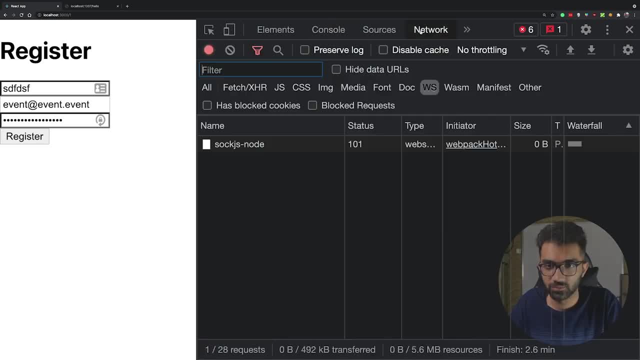 do that and refresh, or maybe even not even refresh. you can see right here we no longer get the course. but actually, uh, unexpected, greater than symbol or less than in json. that is because we are receiving just the wrong response at the moment. so if you go right here, you can see that we get the response all right. so now it's. 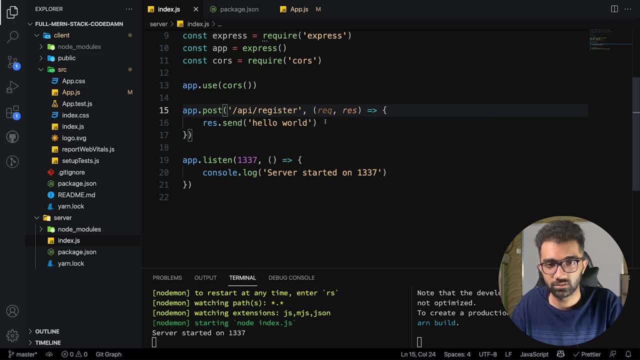 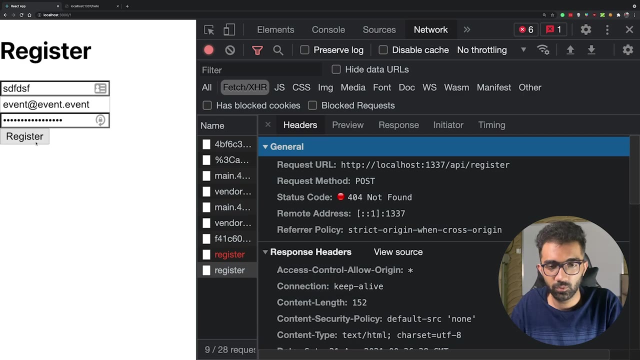 time to set up a handler called apppost api register. now the first thing we want to do is, of course, we can just say restjson status, okay, but how do we get the body here which the user is passing? because if you do something like consoleorg, requestbody, you're gonna see that. 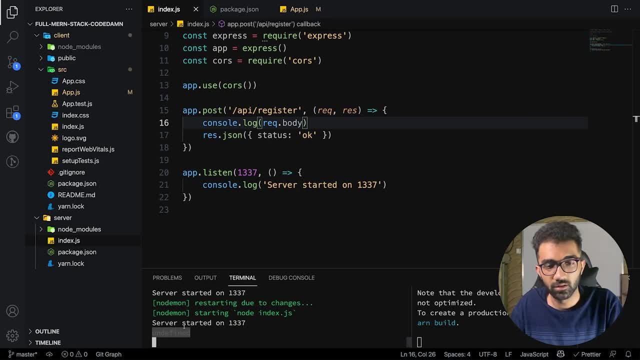 when i click on register we pretty much get undefined here in the console right. so that means we are not receiving the body yet we are, but that is not available, at least on the requestbody syntax right here. so the reason for this is because this route does not know that you are. 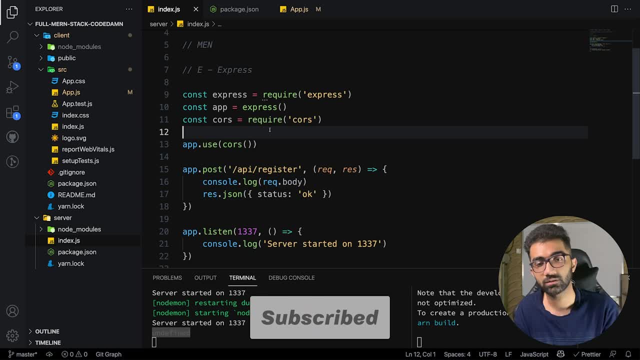 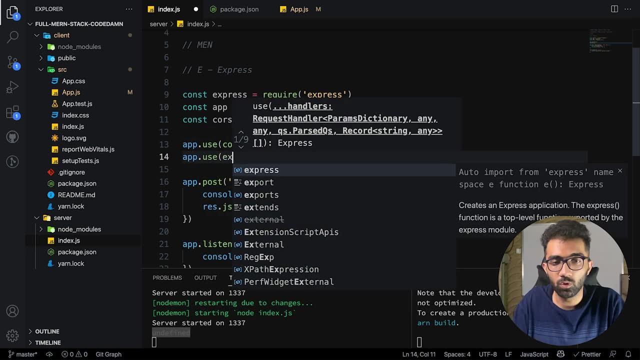 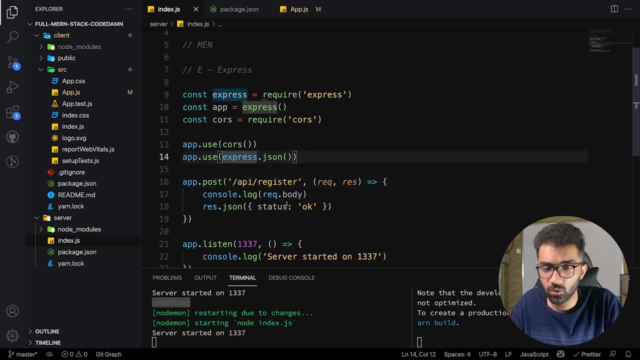 passing in json right and in order to let express know that, hey, we're going to be using json a lot to pass, you know, to pass the body. what you also want to do is you want to use an expressjson as the middle where. so what this does is that it says to express that, hey, we're going to be going ahead. 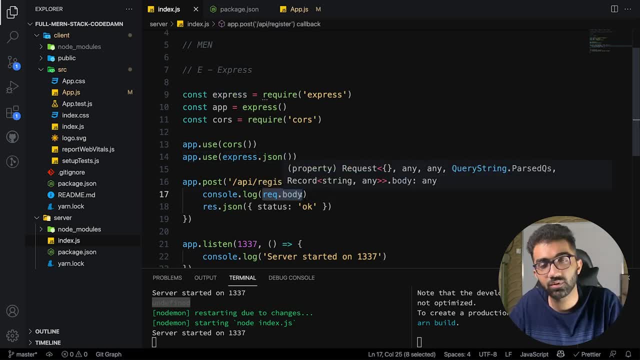 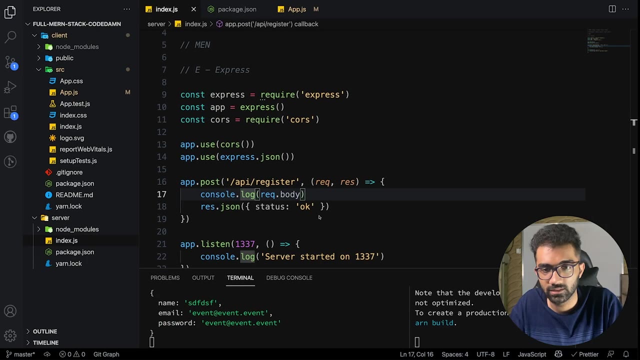 and you should be going ahead and parse anything which comes as body into json- right, that's, that's all it does- and also, like you know, populate the body in the first place, because if it does not, it's just undefined anyway. so once we do that, hit on register. now you can see, we get status. okay, as. 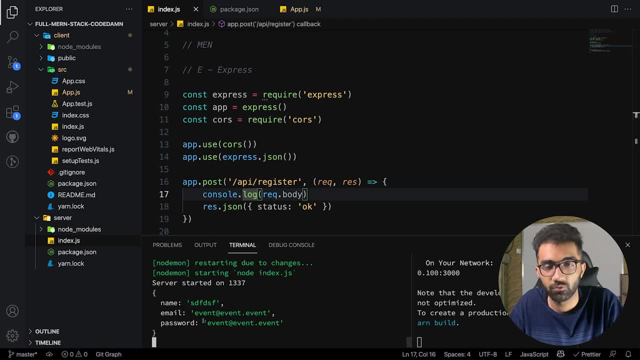 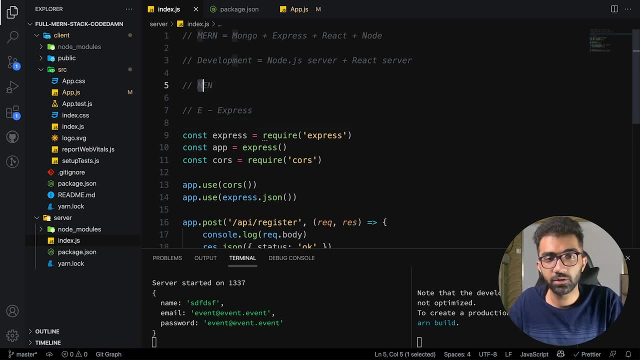 the response, as well as this data which we got from the front end, right, so that is cool. okay, so we are basically done with the, with express and node here, and the only thing we need to do is link mongo now, right, so the way we're going to be doing that is by actually installing another package called mongoose. 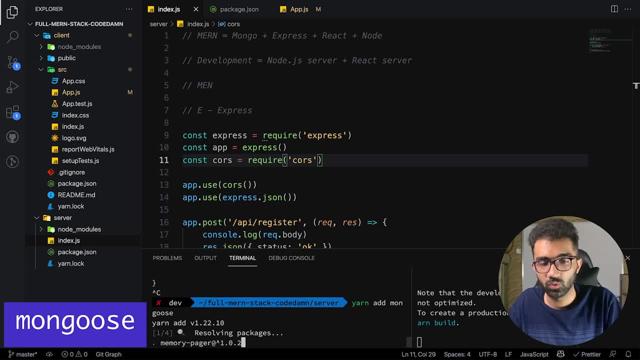 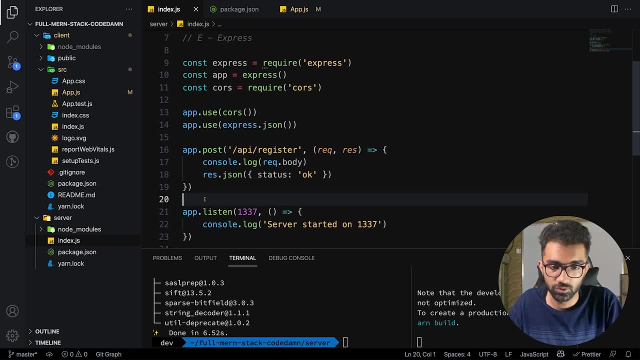 and mongoose allows us to define models and work with mongo db as well through it, right? so mongoose can be as a? you know it's. it's an orm which allows you to connect to mongo db, but it can be a bit useful for data validation and just schema validation as well. 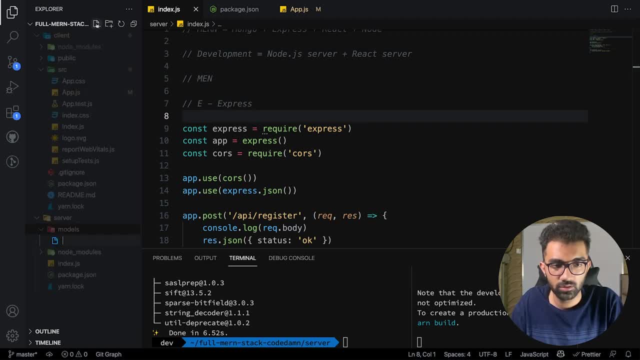 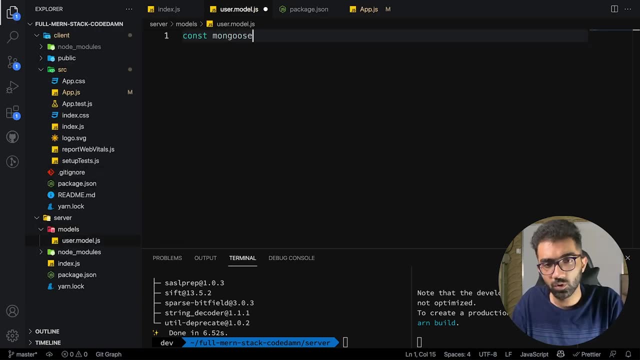 i'm going to be creating a folder here called models and i'm going to be starting with user dot modeljs or, you know, userjs, whatever you want to do. so what you want to do is you want to get mongoose first by saying, require mongoose like this, and you want to define a model. so you 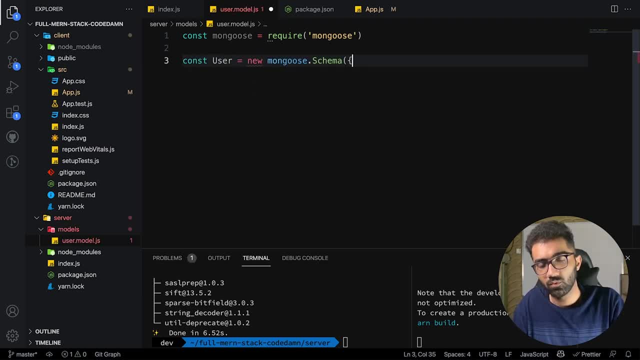 want to say my user model is something like new mongoose, not schema, and it should be having a property called name, which is of type string, and this is required property as well required, true, you can say email type string required to and password required. you know, github, copilot, just. 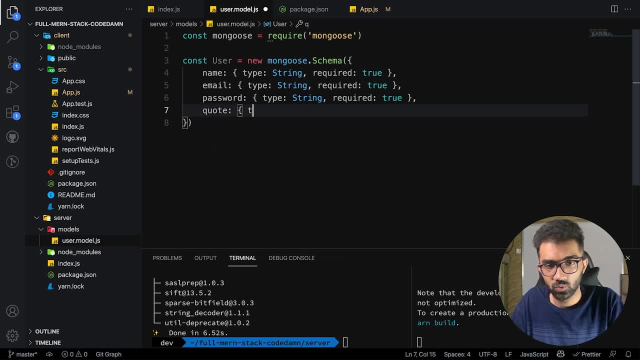 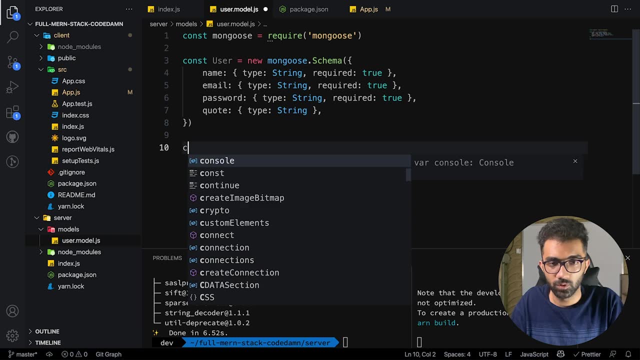 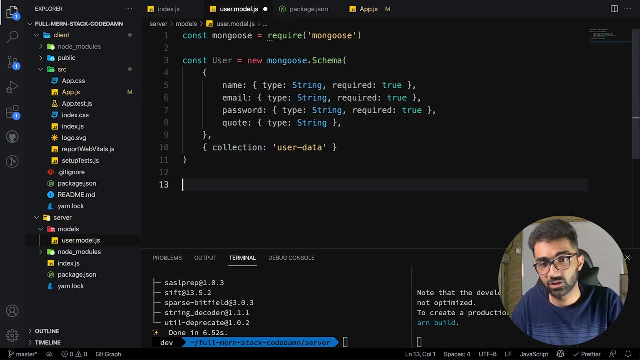 taking over the world. we don't want to create an ad, we just want a quote. let's say: this is of type string and it's probably not required, right? and all we need to do is we want to say that the collection of this model is user data. for example, this is the name of the collection in the mongo. 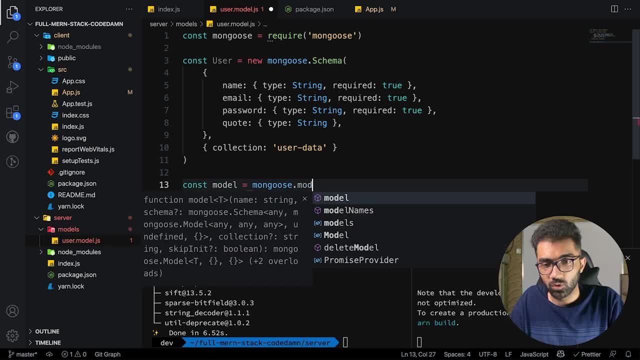 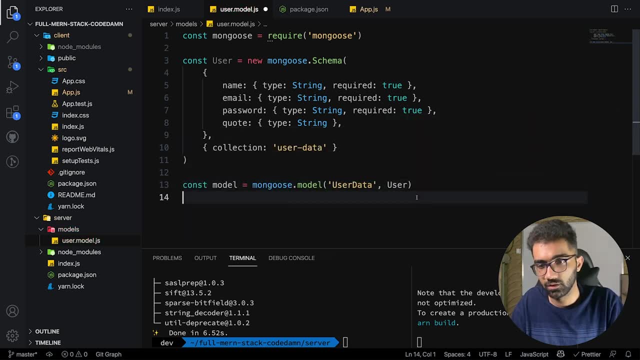 db database which you're creating. next, we create a model by saying mongoose dot model, give it a like user data or something, and which is the schema associated with it? that is the user. and then finally you just say export, not for default, but module dot exports because we are in, still in. 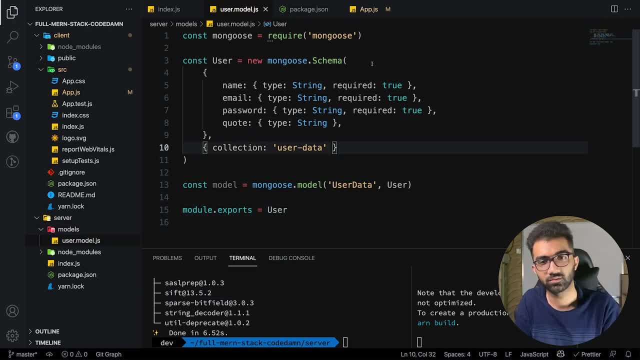 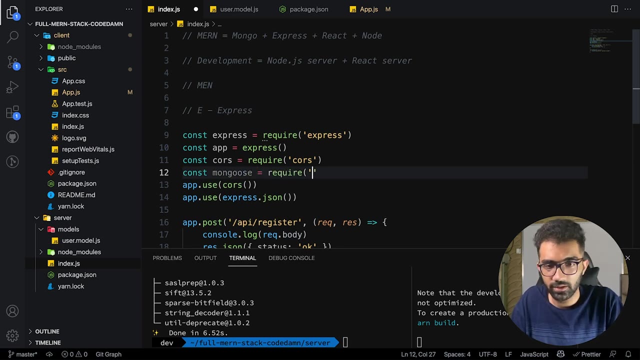 common js world. i should have probably done this in es6 modules, but anyway, we'll probably do it sometime later. mongoose this model right here. so this model just allows us to directly access and interact with mongoose. the next thing which you want to do is also import mongoose right here with 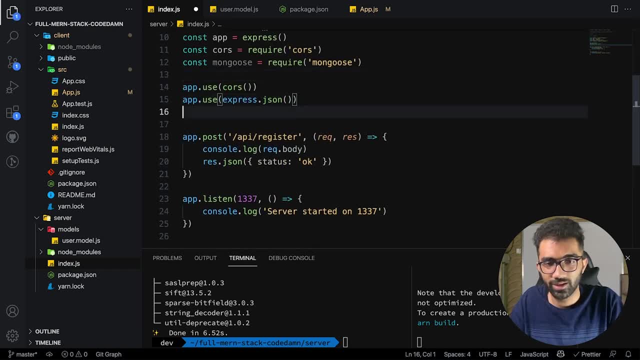 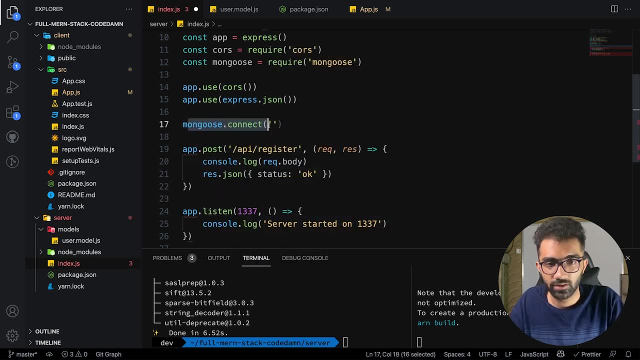 us and the reason for this is because you want to connect to mongoose before anything happens right. and the good thing with mongoose is, although this mongoose dot connect returns us a promise, but mongoose internally queues, that is, it puts it in a queue of things to do if the connection is. 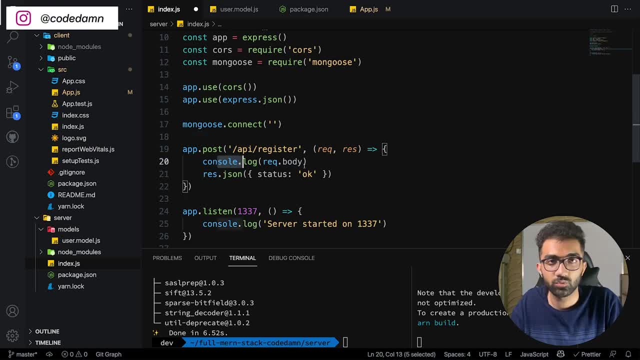 not ready yet. so you can technically just connect it in a synchronous way and, just you know, start using it anywhere you like. so what you want to do is specify a function, specify a string here, connection string. in my case, i'm just running a local host, mongo db. let me just see if my mongo db is running, not. 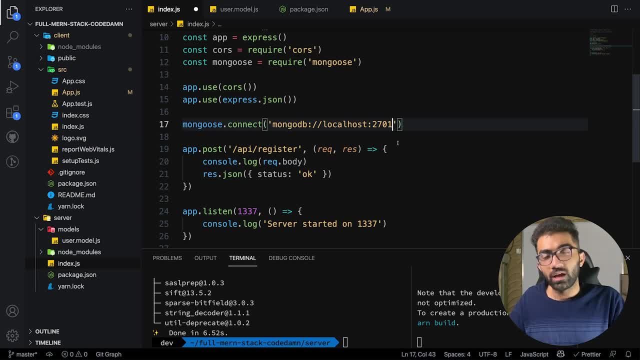 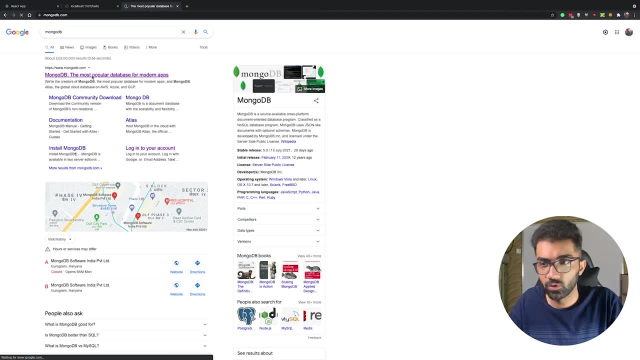 really so i'm just going to start my docker for you. you would have to install mongo db on your system again. it is pretty straightforward: just go to google, write mongo db, go to this mongo db website, download the start do or start free, or download the community server edition, and just 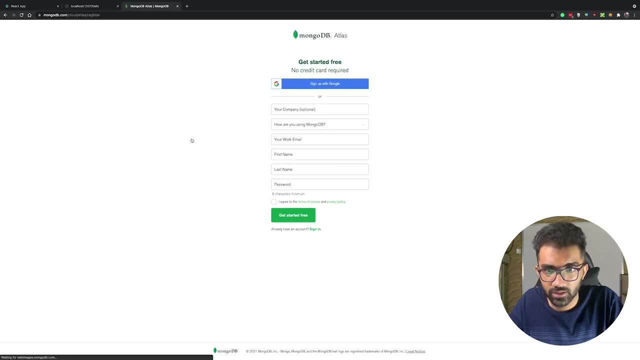 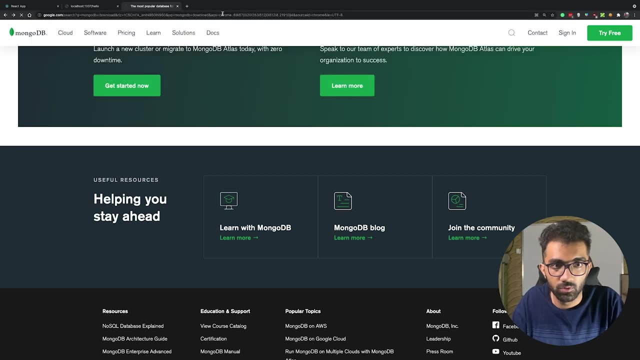 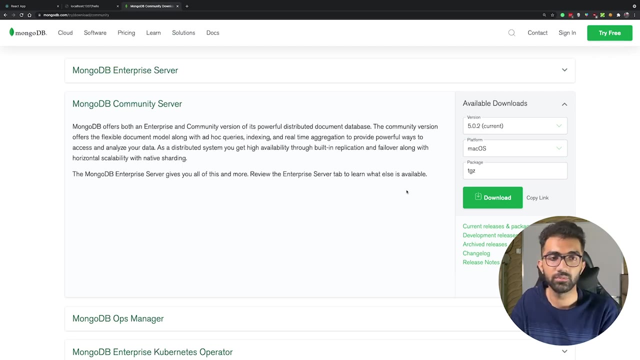 start it by yourself. i think if you do go to get started here now, you don't need to probably create an account. let's see mongo db download. yeah, you want the community download version and once you download it it'll install it, open it, it'll automatically be started on port 27017. okay, so once that is done, 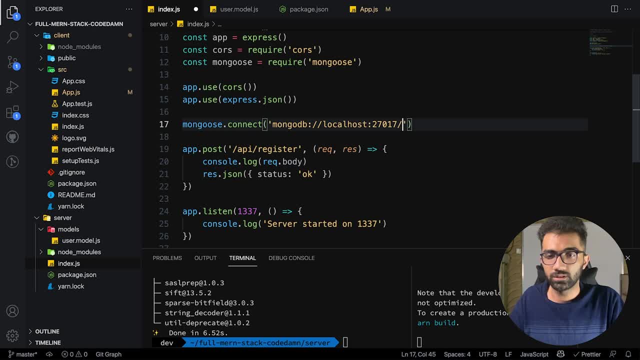 you should be able to write something like mongo db 27017 and the name of the database, and the good thing about mongo db is- or bad thing, depending on how you see it- that you can pretty much specify the database name and collections right away inside the code and it'll automatically create it. 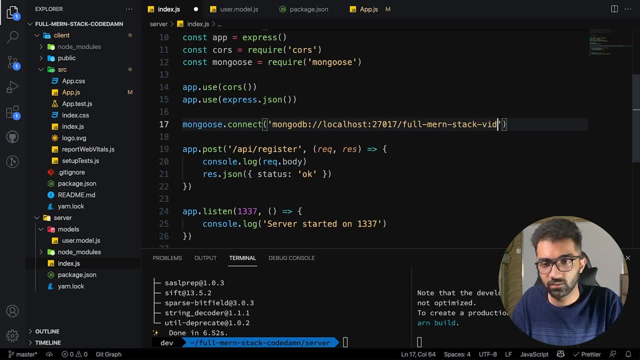 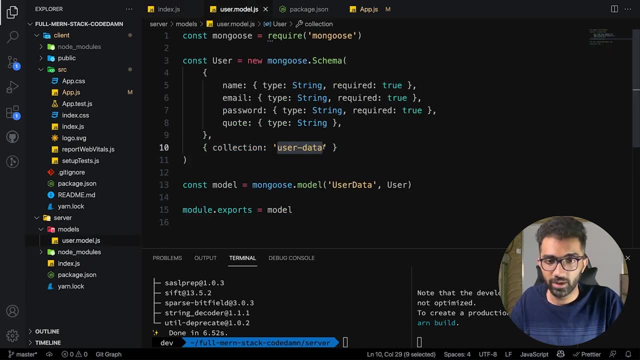 if not present, i can just say this- as full mon stack video, for example, and that's it. it'll automatically create this database and then, when we use this user model, it will automatically create this user data collection. all right, so once we have this, all we need to do is actually we can. 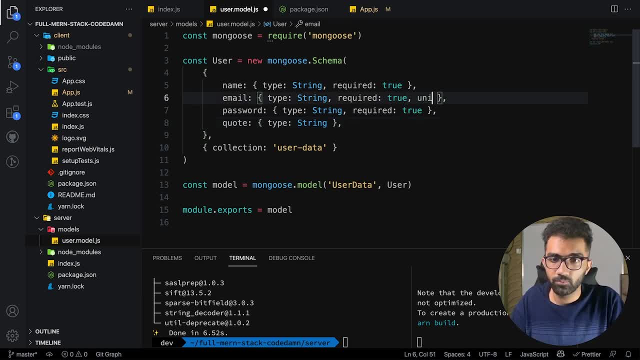 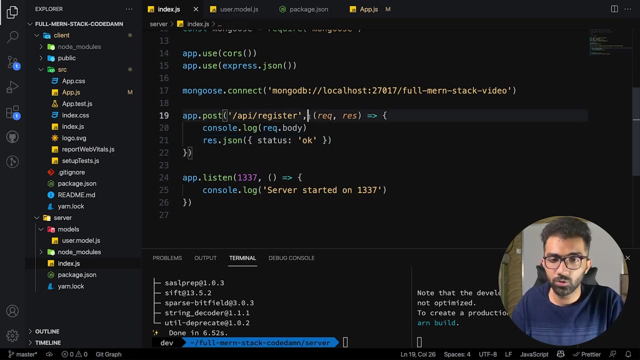 actually go ahead in the model and do one more thing. we can say: the email address is also unique. so what this would do is this will create an index in mongo db which will be on uniqueness, that is, there would not be a duplicate value for email or it will just throw us an error right. so what we want to do is we want to convert. 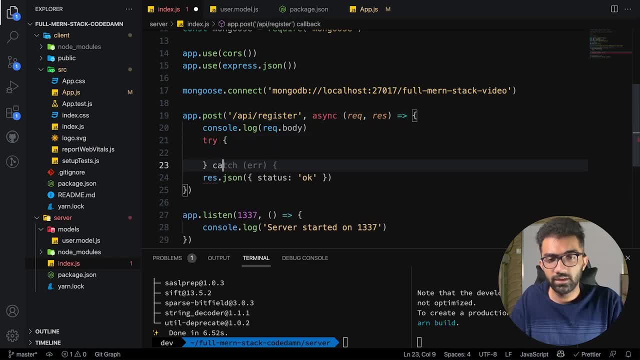 this into an async function and throw it inside a try catch. so we want to say, okay, restart json error is fine. but we also want to say, let's see what code pilot has to offer. yep, that is pretty much it. that is pretty much it. that's what we want to do. but it's always a good practice to 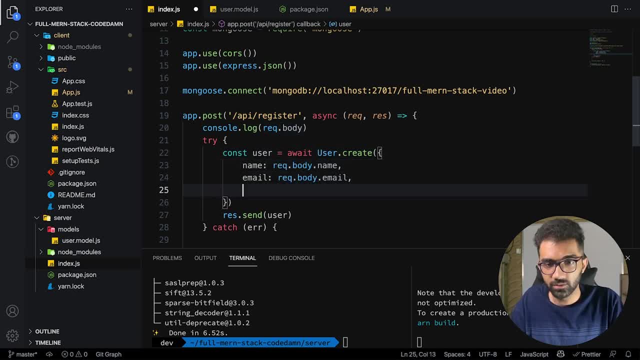 not just arbitrary use user data, but instead do something like this. right, because now i know that, hey, i'm in control. right, what goes into the database? and, yep, i think that's all we are getting from the user side, right? uh, name, email password, yep, that is true. 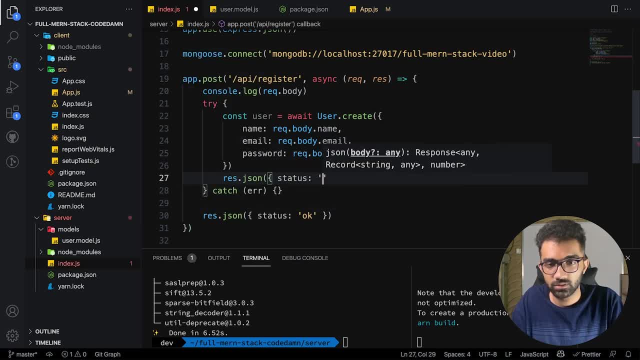 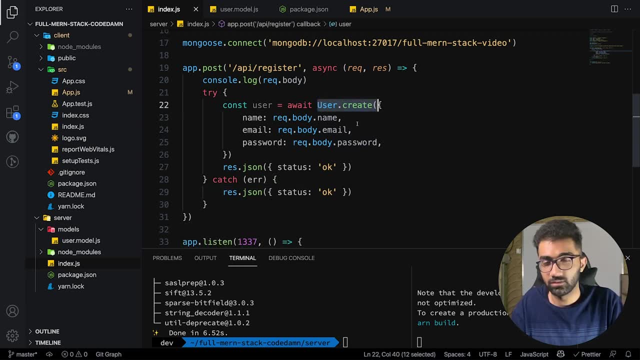 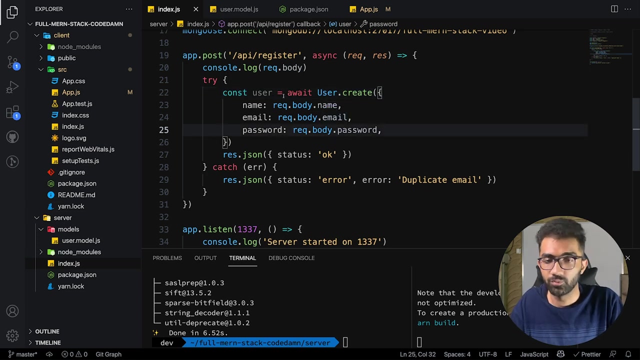 and then we finally say restjson status: okay, right, otherwise inside catch, if we are arriving, we know that the record is already found. it is duplicate. so we can just say status error and then error is duplicate email. right, something like this. you can perform more validation here depending on maybe, like your name should be certain characters. your email should be: 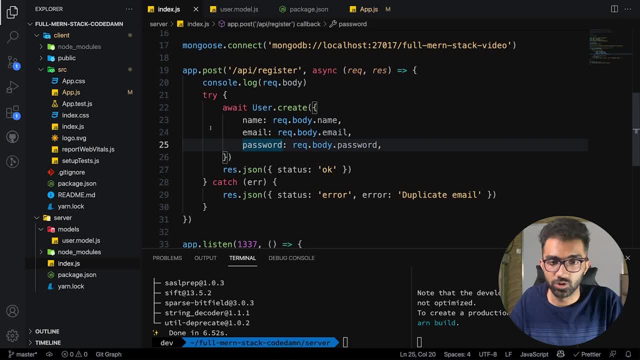 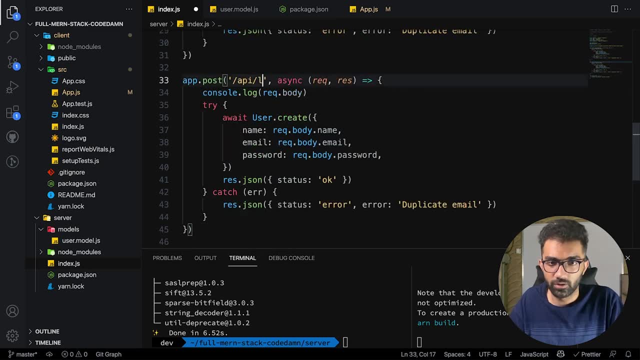 certain characters and so on, but this is like the bare minimum version you should do in order to handle the errors as well. okay, so once that is done with us, let's just quickly go ahead and create a login route as well, and maybe actually let's just say: yeah, i think we can just go ahead. 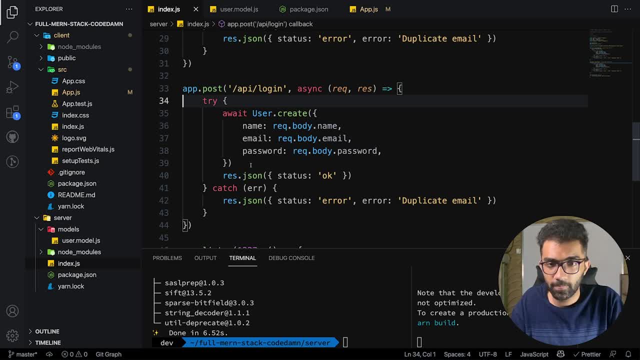 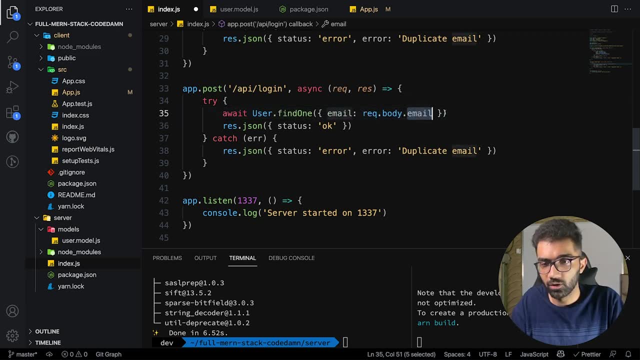 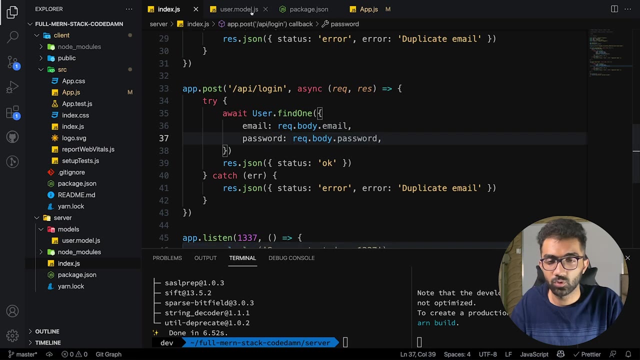 and create a login route right here. what we'll say is: instead of usercreate, we want userfind one with an email of requestbodyemail and password of requestbodypassword, and this is actually a bad practice to store passwords in plain text, which will shortly cover how we should fix this- but we can just say that if we have a user right here and 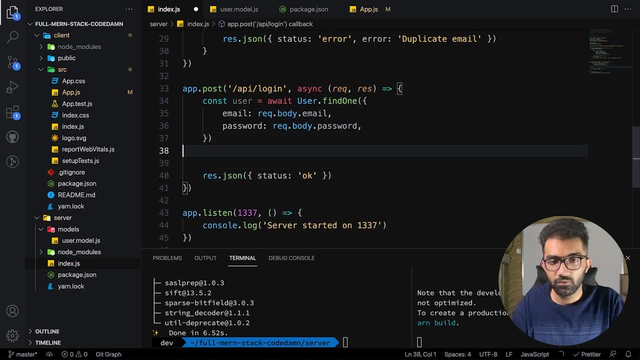 we can just remove try catch from here, because it will not fail if we have a user until nonetheless your mongodb connection itself fails. but yeah, then we just say return restjson status okay, and then user true, for example. we'll return some sort of authentication information here, ideally. 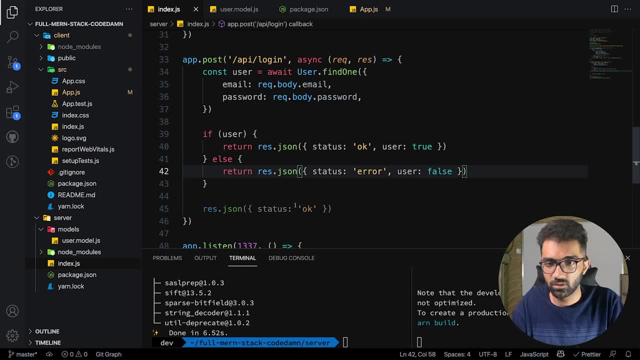 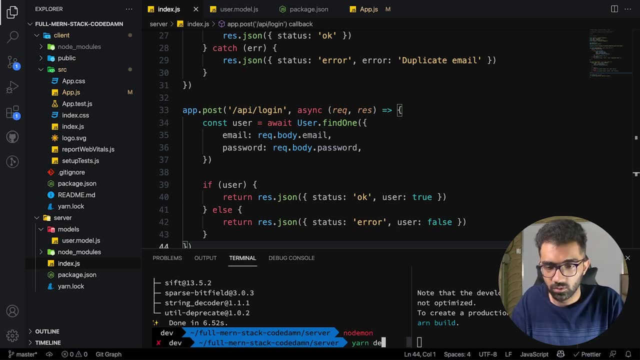 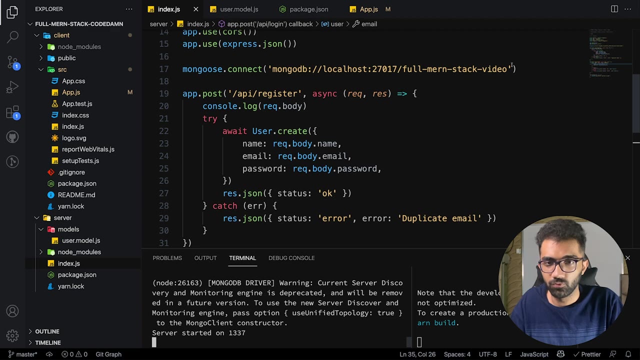 else what you want to do is just return restjson error and user false. that's it all right. i think we have the bare bones code ready with us. we can start it with nodemon no yarn div and once we do that, you can see we get some mongodb warnings. it needs some new flags here, which. 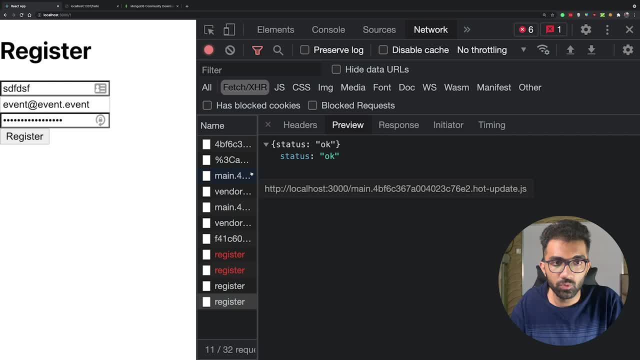 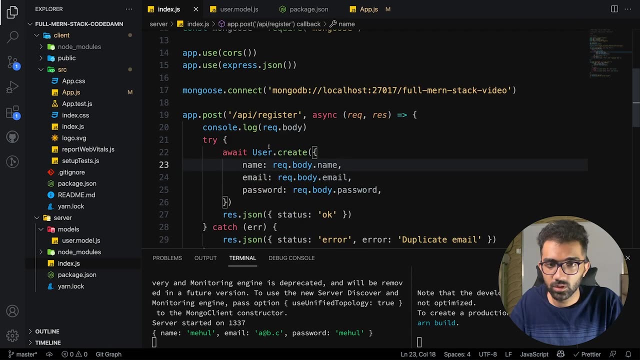 is fine. i mean, they're just warnings at the moment, but what you can do now is go back right here and you can start with, let's say, a at the rate, b, dot, c, right and mayhole, let's say, is the name and the password. so when i register now, you can see that we get a duplicate email, which 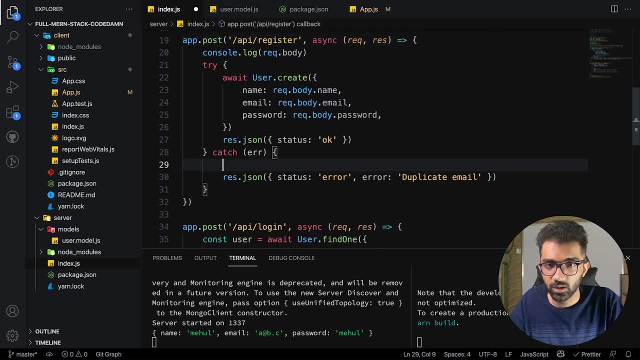 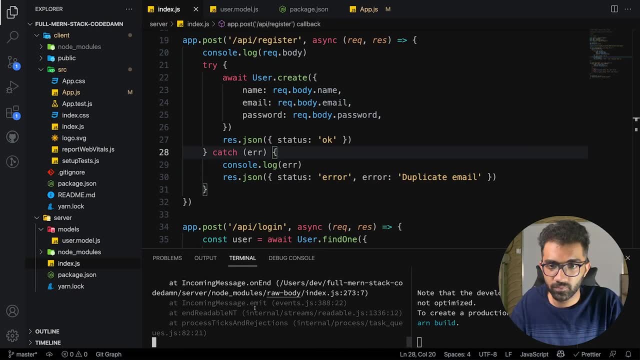 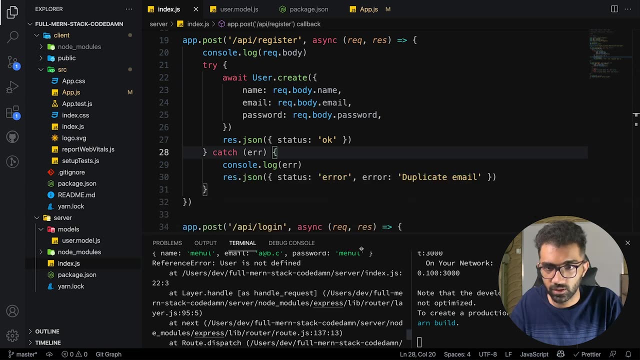 is probably not we were expecting. so let's just debug what is going wrong by also console logging the error right. so now if we register, go to the console, you can see that we have an error saying: not defined very well, because we probably did not import this model. so what we want to do is also: 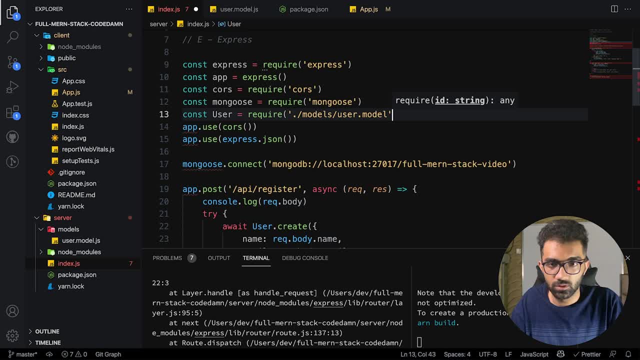 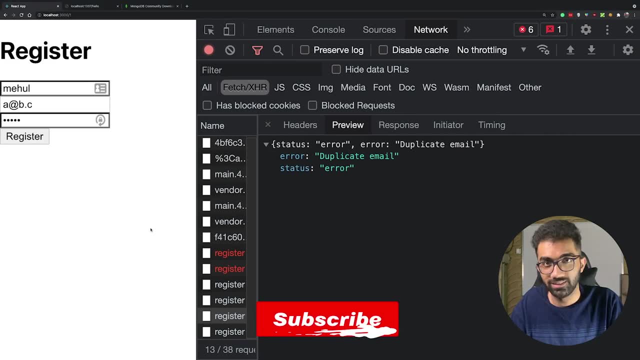 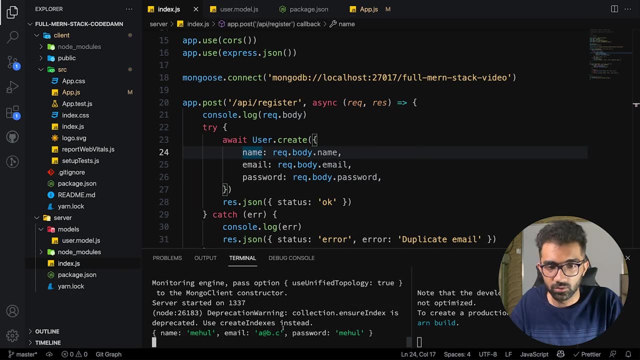 import it from models, user dot, model right. and of course this would be screaming loud if you were using typescript. that is one of the reasons i like typescript, of one of the many reasons i should rather say: yeah, you can see, now we get status, okay, and here also we get the console log. if i try to 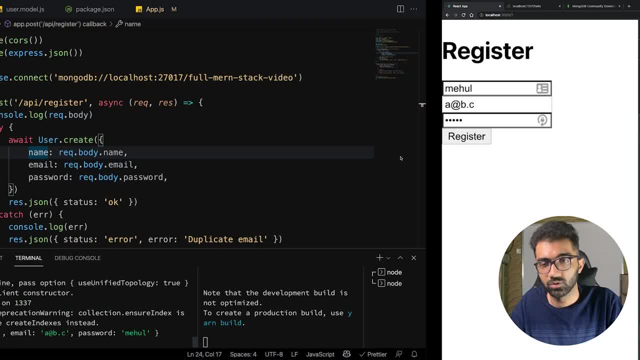 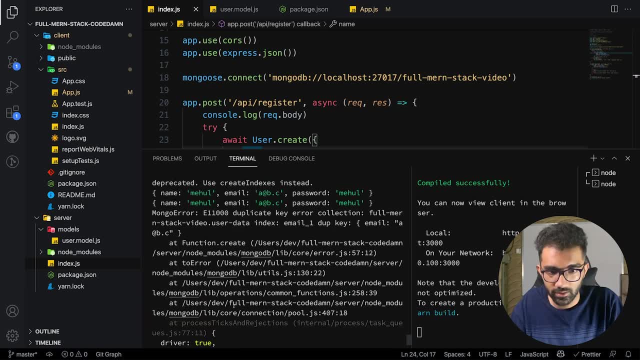 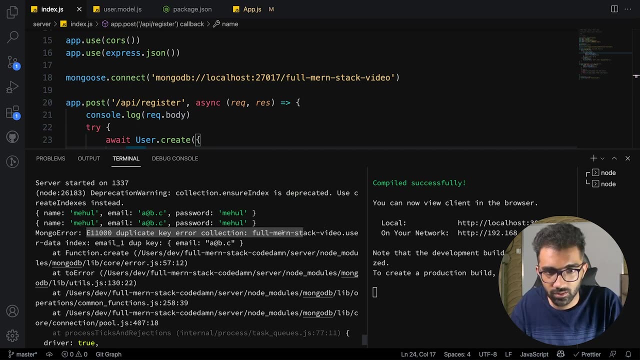 create this user again. then we will actually get a status error right, which is now correct in this. in this case you can see the error which we get from mongodb is right. here you can. you cannot actually see it very well because the error dot message is kind of hidden here. 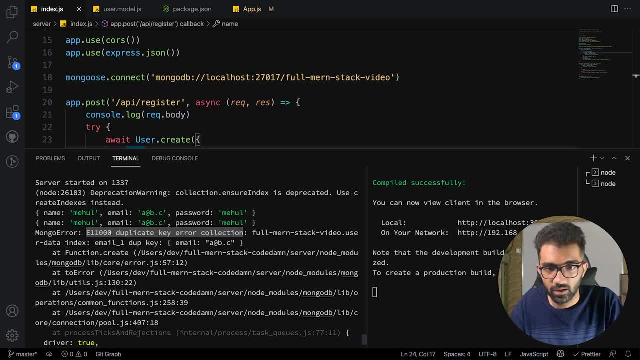 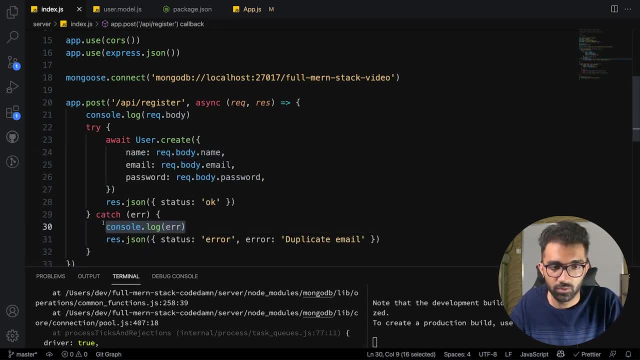 which is like: this is the error message, right. but yeah, i mean you can technically just take out this error message and detect if this is truly an error of duplicate key or not, because just use just like you saw. in any other case it will return you this error. so it's not very tight. but 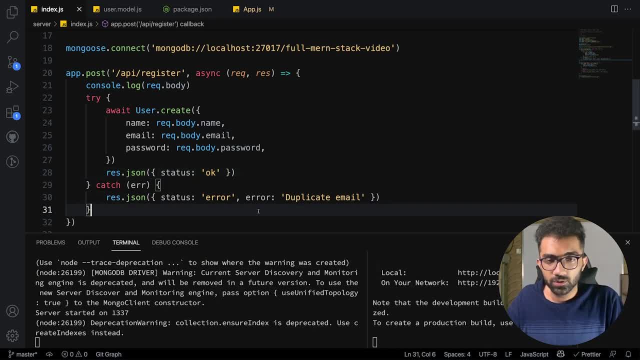 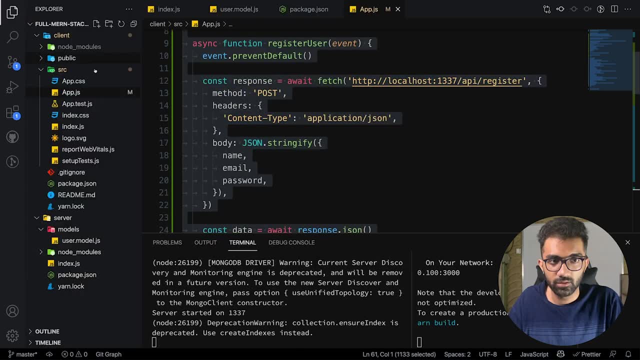 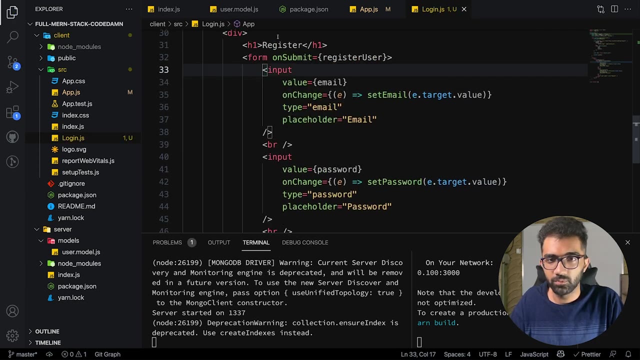 anyway, that's fine. that's fine to start. okay, so we are very close to creating our basic full stack application. here we have a registered user. let's just go ahead and create a simple login page as well. so i'm going to say loginjs, and it's not going to contain name, but pretty much everything. 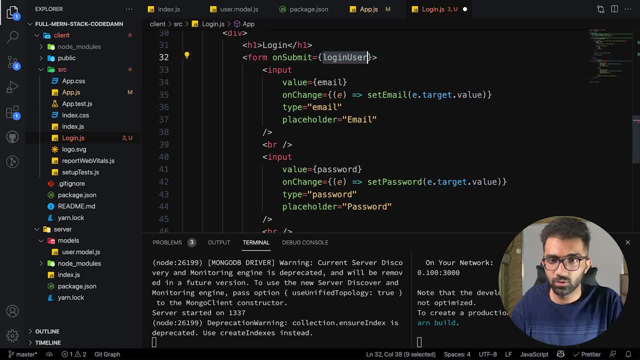 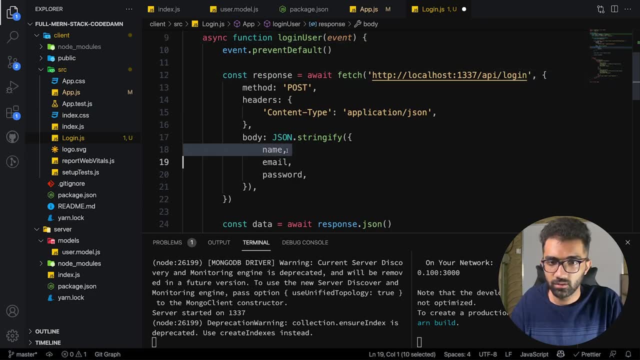 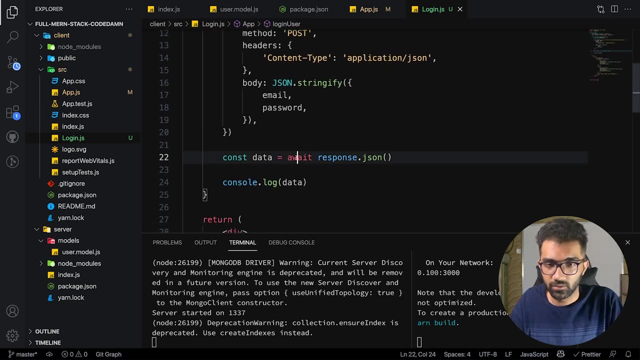 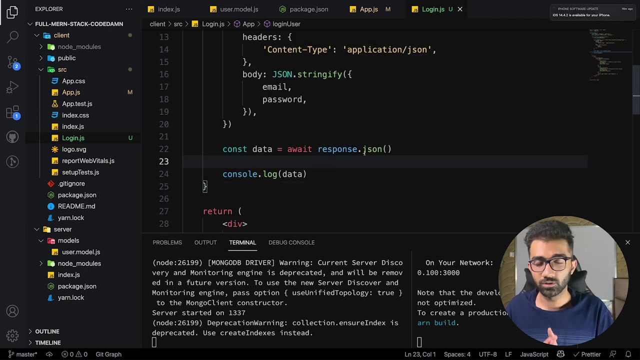 else it will be login, it will be login user, and the only change which we need right here is saying that this is api login name. we only have email and password, and we also don't have this thing right here. right, so you can see. rest of the stuff is pretty much the same. all right, so the next step is once. 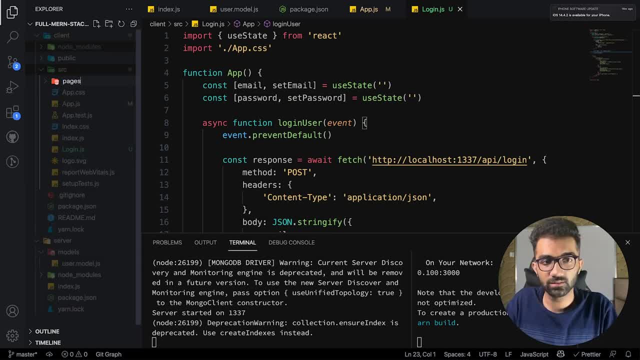 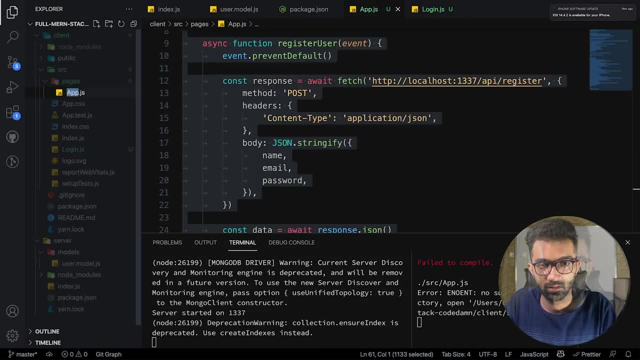 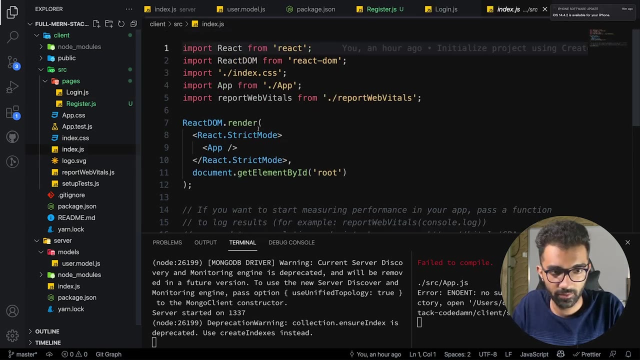 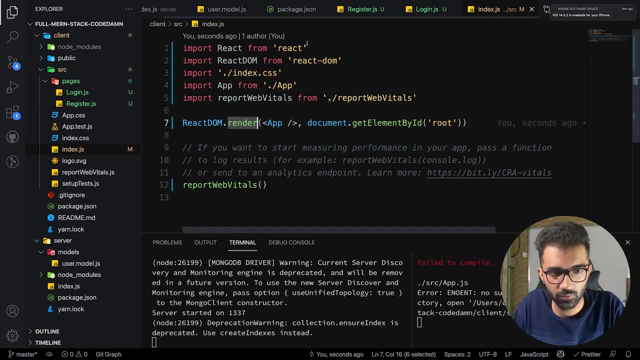 we have this login page actually, let's just go ahead and organize this in a better way. so we're going to be saying this as pages and let's say i move this inside as um register. let's do a little bit of nextjs style thing: login, not exactly, but you know, and we can do create root, but i think we have not installed. 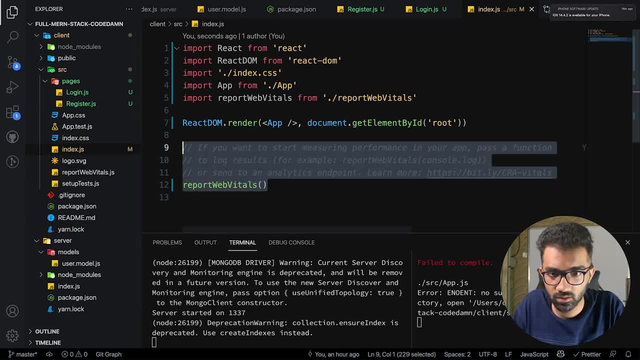 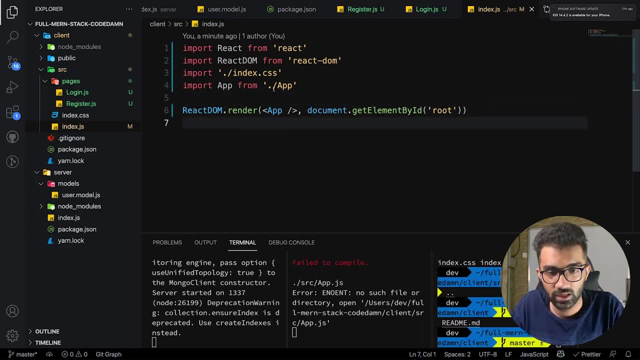 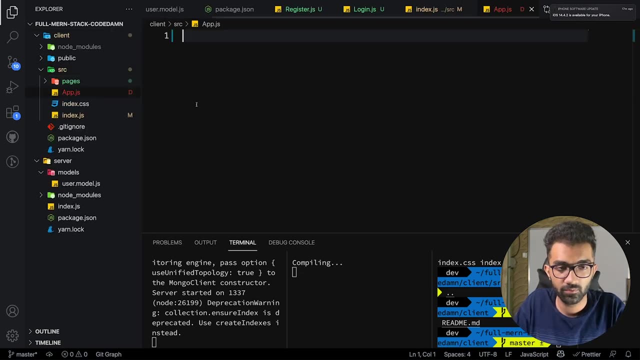 react 18 yet here, so it's fine, we can just keep it up. render: we can remove this, and i have just removed some unnecessary files. it looks a bit cleaner now. you can see we have an app which is being imported from the wrong place, so what i'm going to do is create an app component and we're 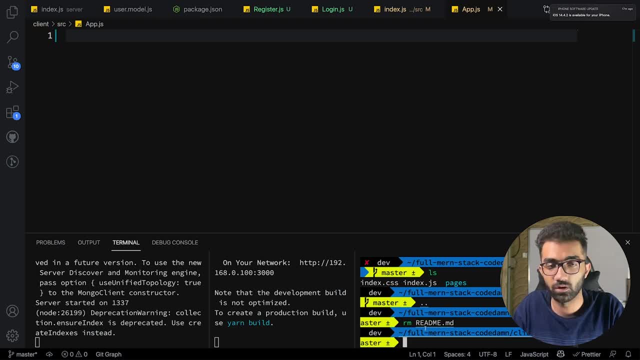 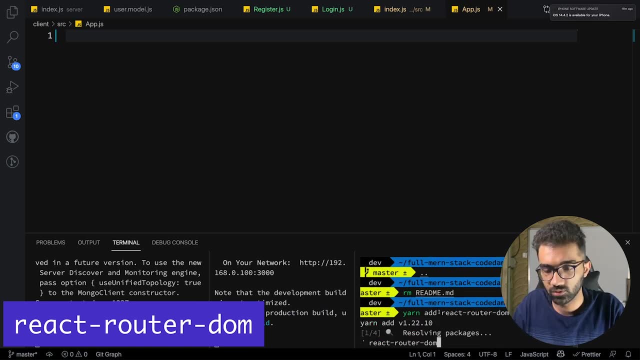 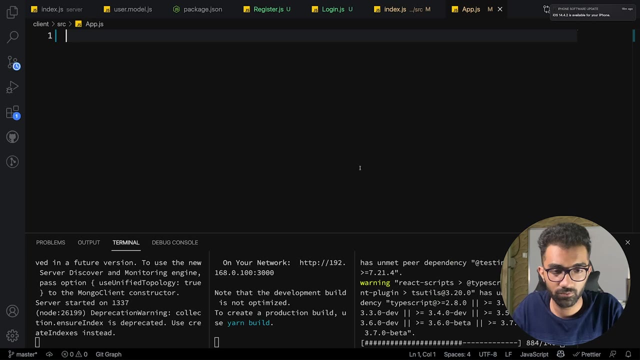 going to also be using react router. now, right, so in order to provide routing on the front end, we'll be doing what i'm going to say as react router dom. so this package right here allows us to perform react routing. that means different, different pages- with the help of client-side routing. and finally, when we deploy. 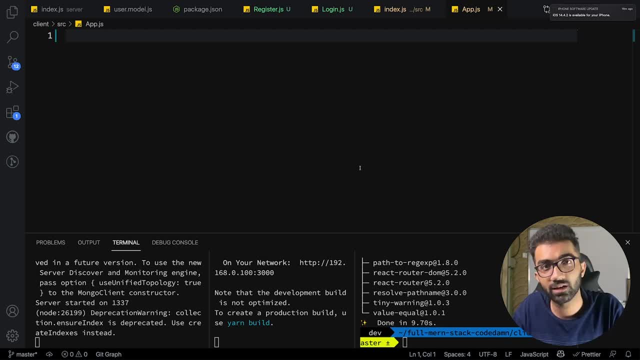 it inside nodejs project as a static files. we will still be doing client-side routing, but that will be also be supported via server side. we'll see when that happens, but anyway, for now let's just import react from react and i'm just going to say: app is a function which returns us. 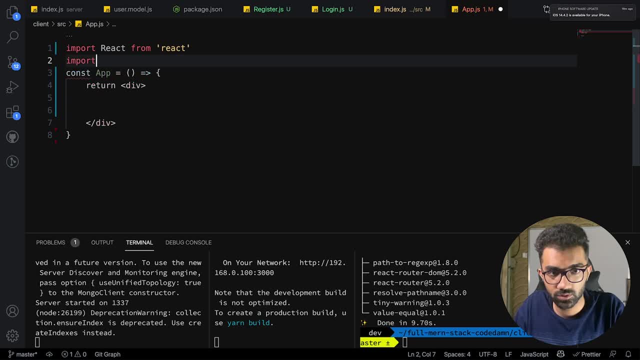 this whole thing, right. so this thing right here is going to be imported from react router dom, which copilot was already able to guess, and this would be browser router, right? so this browser router just provides us with that functionality, which is going to be something like path of this component. this should be actually path login. 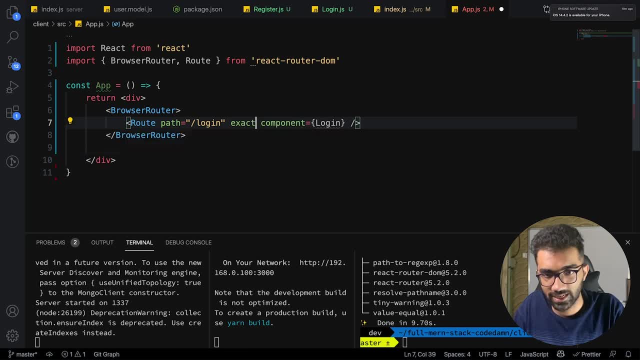 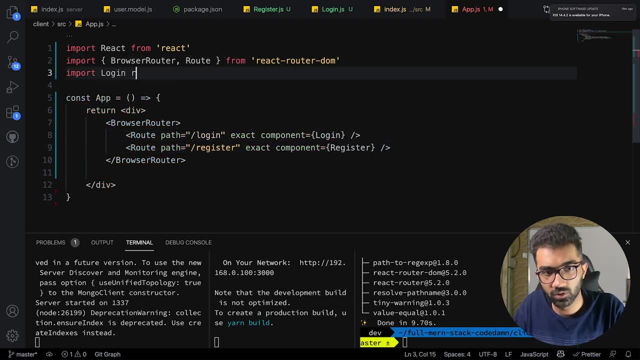 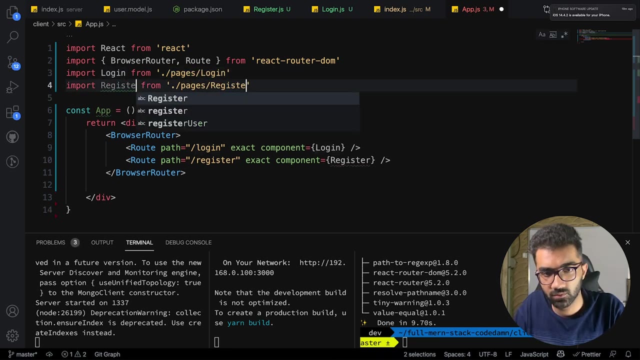 component login, and this should be an exact match and similar thing for register. and finally, we'll also import these two components from pages, and login and register. okay, i think it makes sense so far. so now, if i go ahead and export this, i'm going to get a new page and then i'm going to plug it in, so i will import this and then, if i export this, 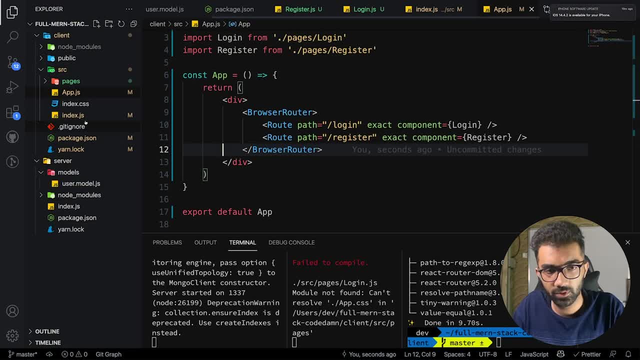 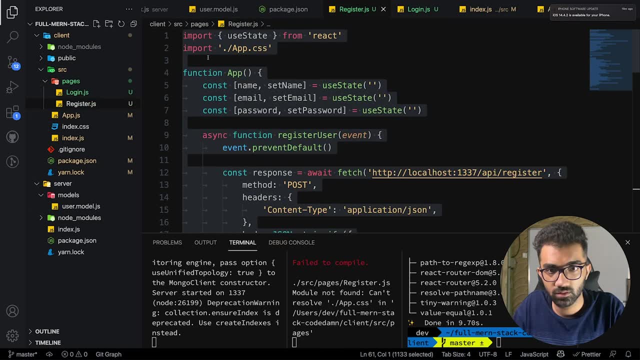 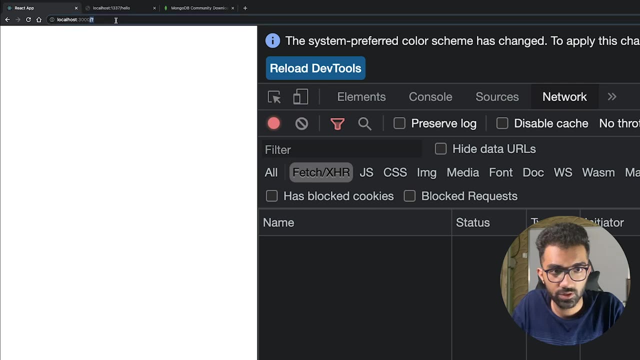 export default app. you're going to be able to see that. let's see, we need to remove the css file imports, i think, and once we do that it should work fine. so now, if i go ahead and take a look right here, if i refresh, nothing happens because we don't have any route. but if i go to login, 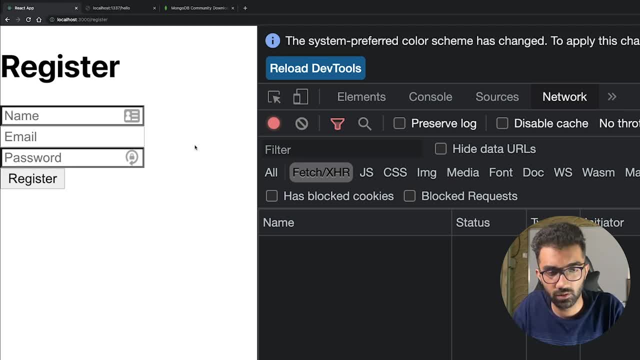 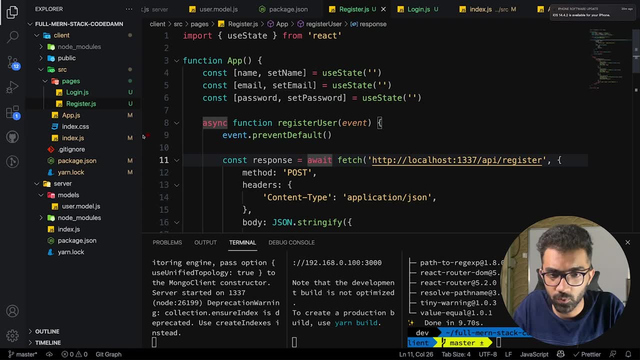 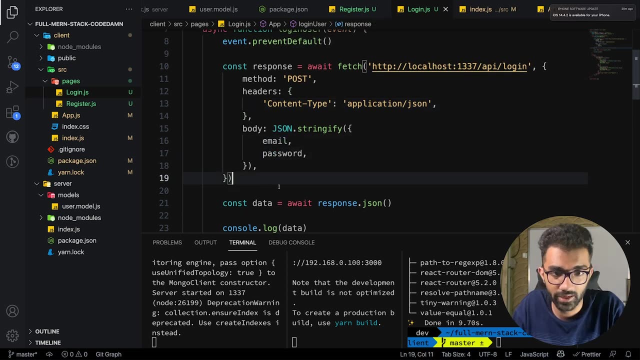 we get the login route and if i go to register, we get the register out. awesome. so now, once again. now let me just refresh this once. what i want to do is inside of login part, we already have done most of the work which needs to be done in order to send the data on the back end inside our indexjs. 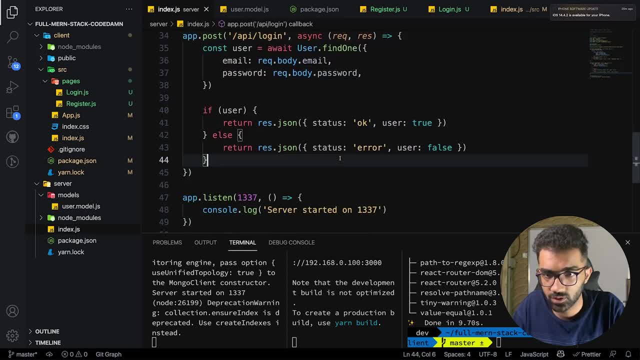 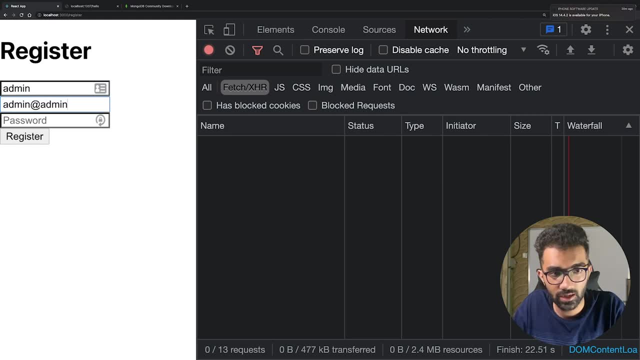 file. inside back end, we will also create a login endpoint. we should do the similar thing, but it pretty much does nothing at the point. so let's just go ahead and create a new user called admin, admin, admincom and the same password. so outside of this this I get in status of okay. if I go to login now, I try this, register this you. 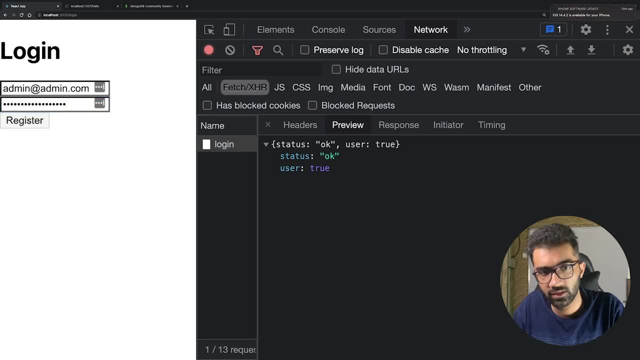 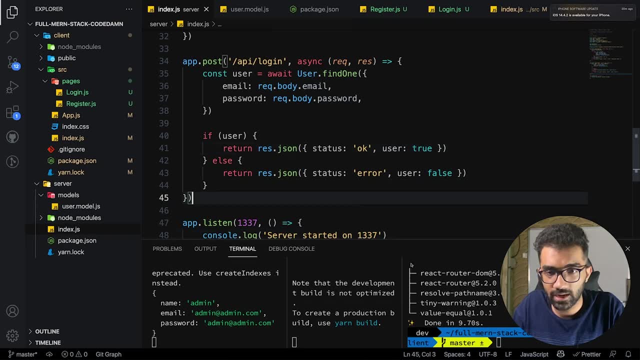 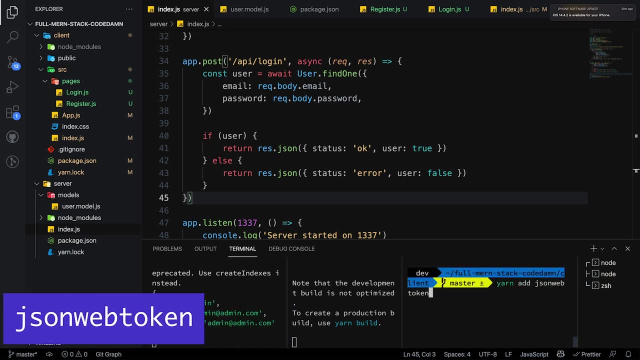 can see we get status okay and user true because my password was fine. if I write 555 here, you see we get user false because my password was wrong. so that is fine. but how do we add authentication to this? in order to add authentication, what I'm gonna do is I'm gonna add another package called JSON web token. and what? 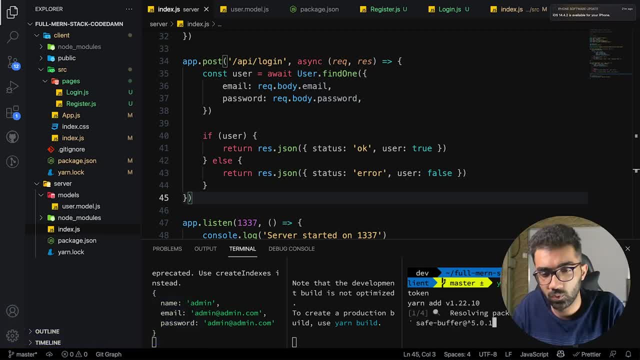 this package would allow us to do is it will allow us to sign JWT tokens and retrieve them and basically work with them. and I have installed this on the client side, but actually it makes more sense to install it on the server side. so I'm gonna say: yarn, add JSON web token on the server directory as well. so what? 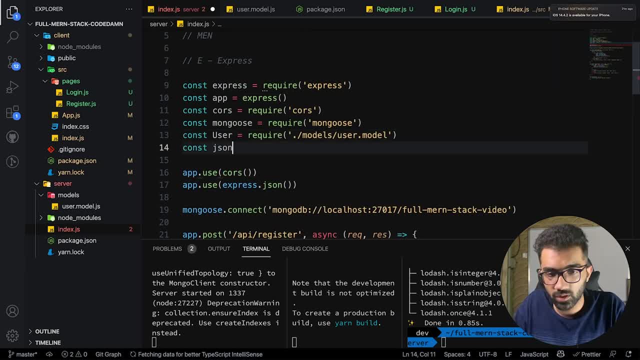 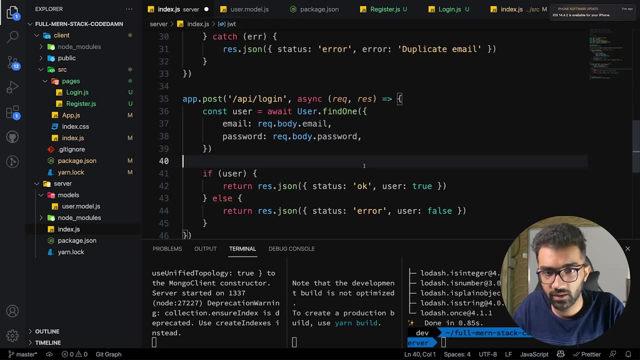 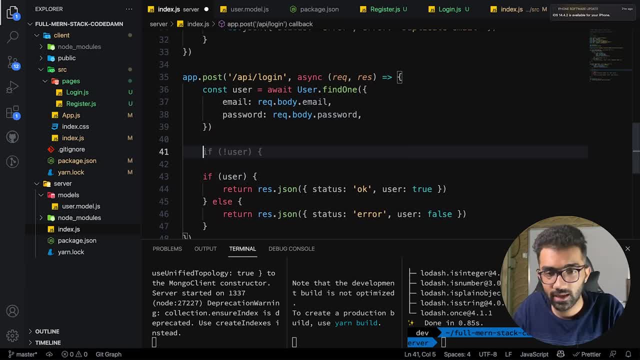 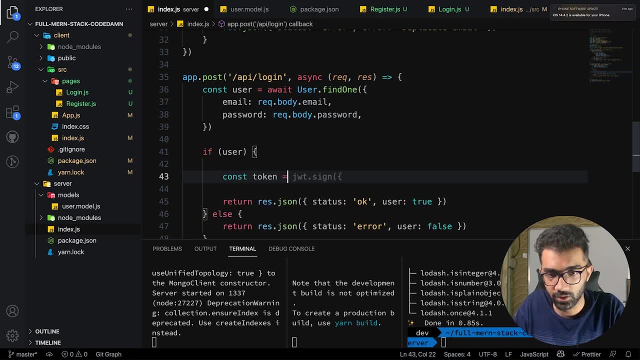 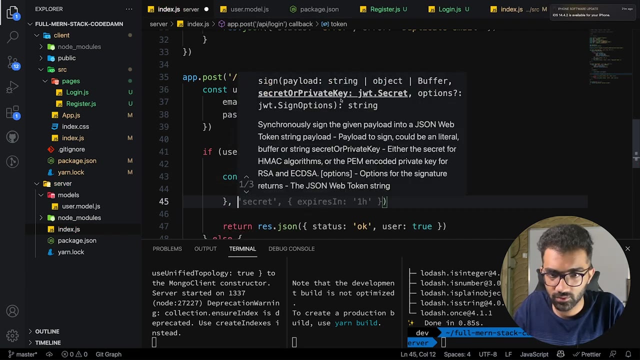 and can allow us to determine that, hey, this user is legit, right? so you know that if the user account exists, we can send the user a JWT token. so we can say: token is JWT, dot sign and what. this is, as far as I remember, the yeah secret of. 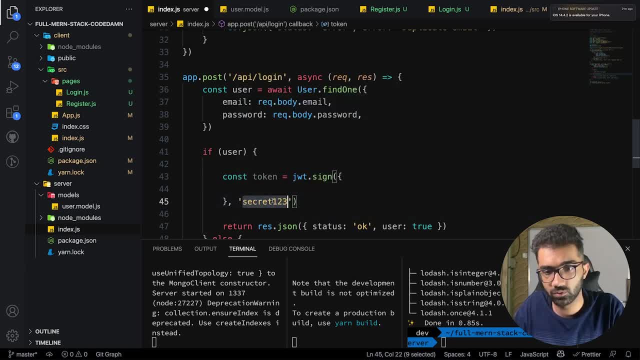 the private key is the second thing. so we are secret, a secret 1, 2, 3, but ideally secret should be way, way way secure and the sign thing right here is just the payload which you want to sign, right in this case. I just want to have an email. 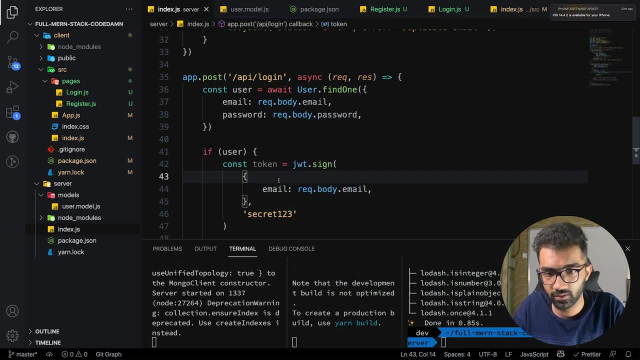 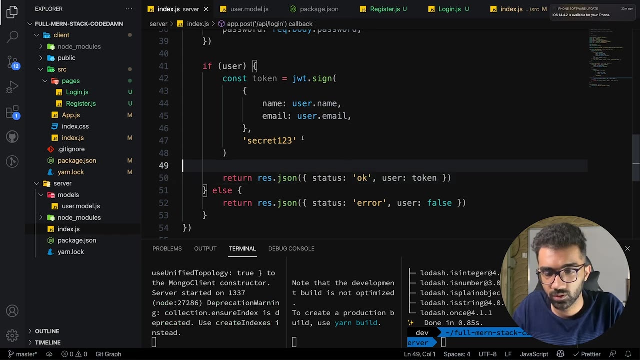 request or body email right here, and probably their name as well. if you would want user dot name, for example, and for the sake of consistency you can also stick with user dot email, and what you finally do is you just send this token down the wire. now what will happen is that when you 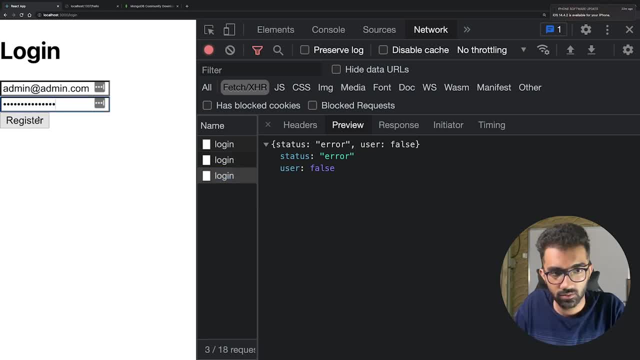 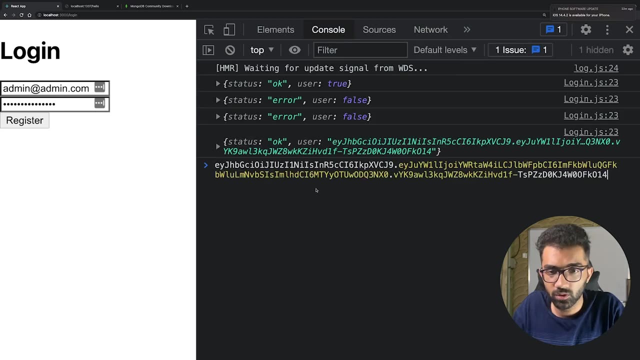 login. if you go ahead and actually move the pipes, if you go ahead, you will see that you receive a token like this. now, what this token is? pretty much it's nothing. it's just a base64 encoded variant of your payload with certain security embedded, and the way you know it is that you see these two full stops. 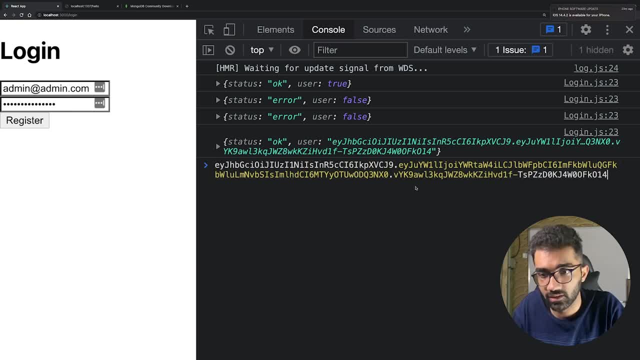 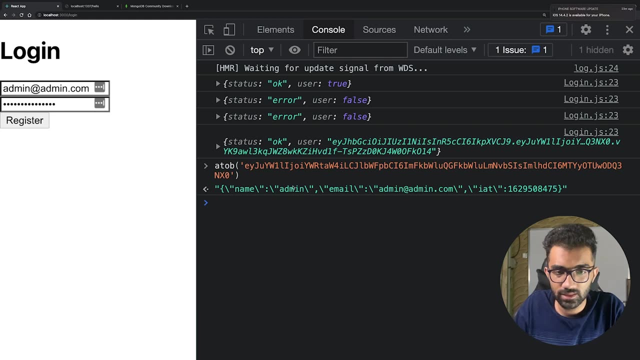 right here and I'm just telling you about JWT right now. this is a standard example of JWT token. this JWT token has the space payload which is in between of these two dots, and this thing right here is base64 encoding, and if I try to decode this with A to B, what you will see is that 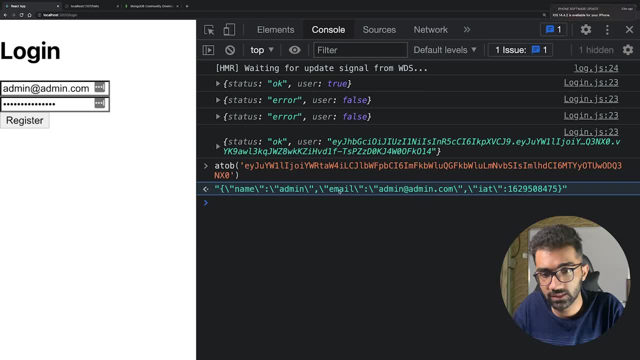 this is a JSON payload, right, with the fields which we pass: name, admin, email, this and also, you know, a creation time of the token specified by the JWT library itself, right, if you just go ahead and try to do it, you will see that you have a, that this is actually the time of creation of this token. okay, anyway, once we have this, pretty much, 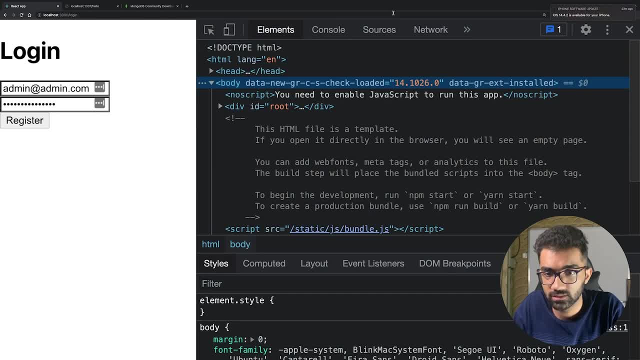 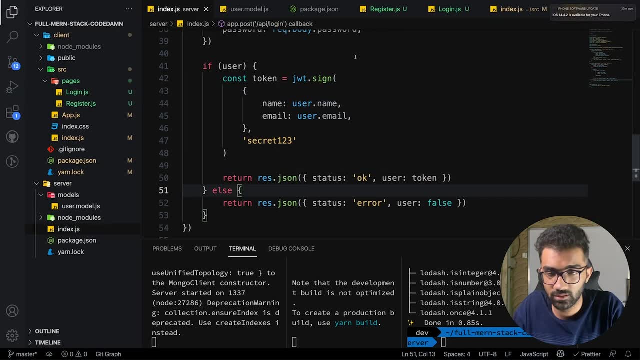 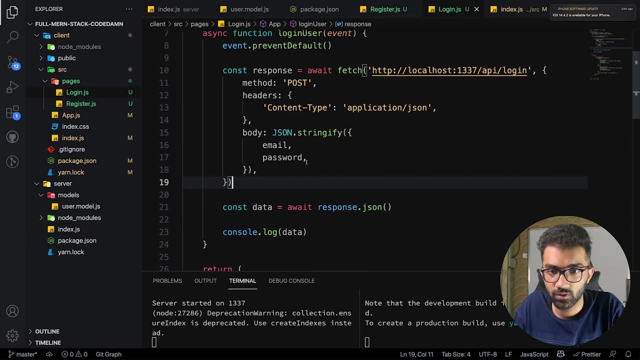 no one can modify this information because if they do, that token gets distorted. you know it will not pass the server side check. so it's fine. i mean we can just go ahead and use it right right there. so what we can do once we have done that is we can go ahead and inside of our login app we can say: 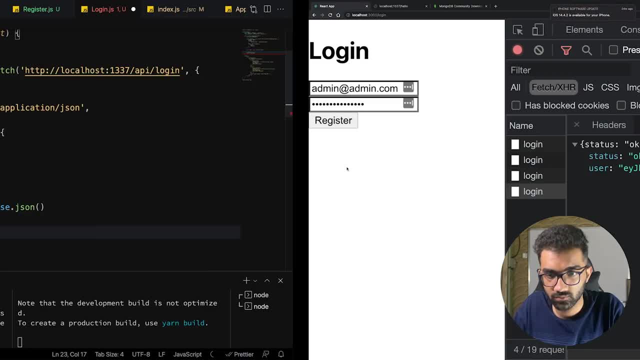 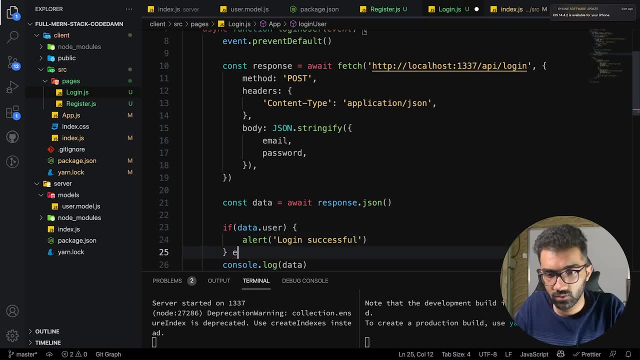 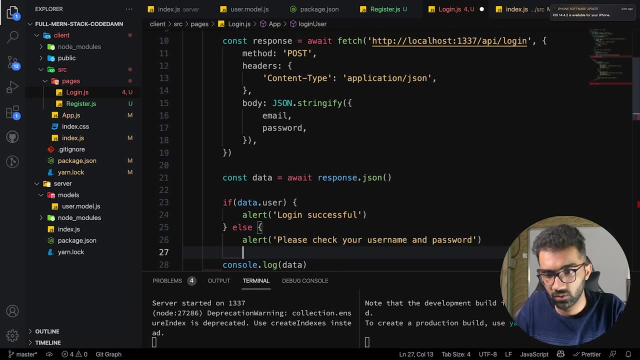 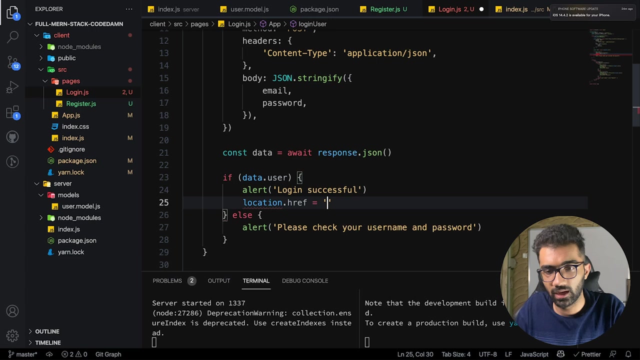 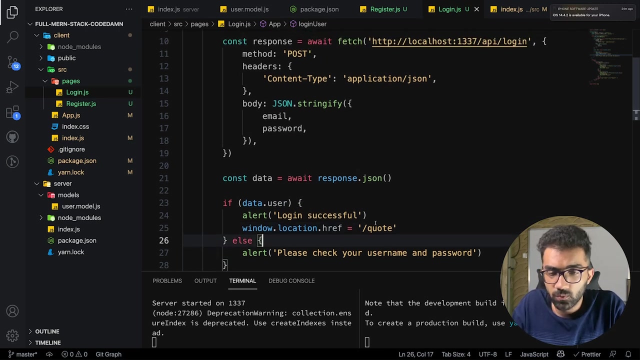 if data dot user exists, then we can say: alert, login successful, else alert. please check your username and password right. once the login is successful, you may very well just send them at a code page right window dot location. so what this will do is it will allow us to create another route here. 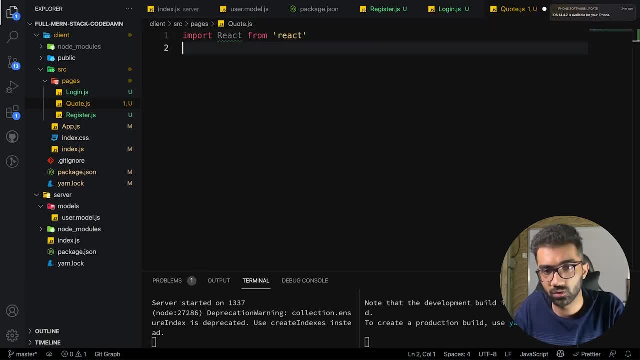 codejs, where we can just show the code of the user, which they have, right. so i'm gonna have a quote page here saying something like hello world, for example, and what we want to do is we want to have the user code being shown here, right? or let's just name this dashboard instead of code. 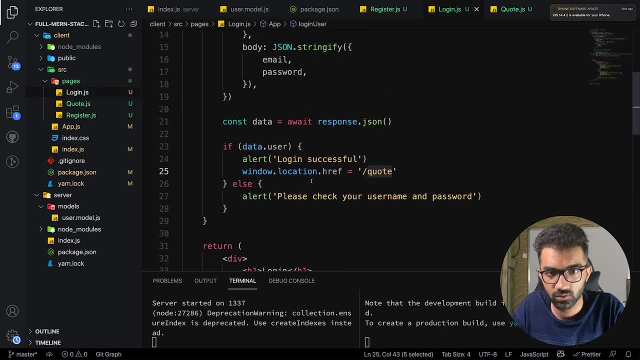 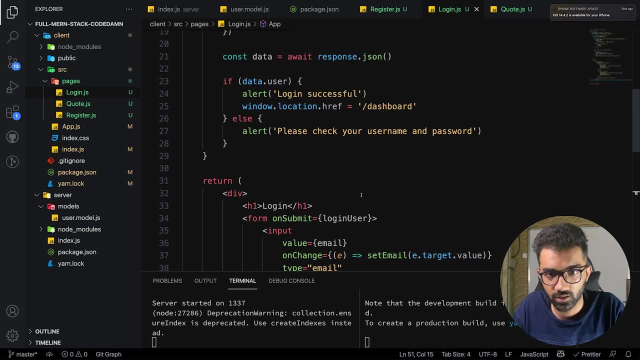 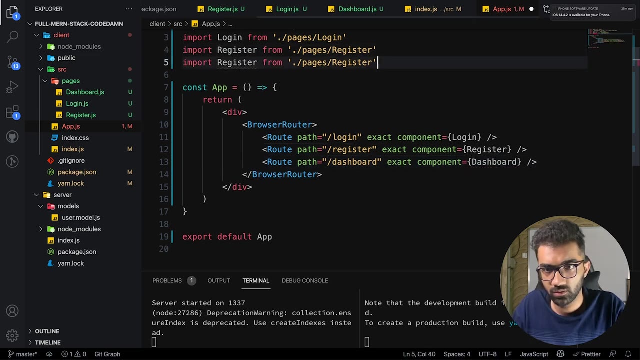 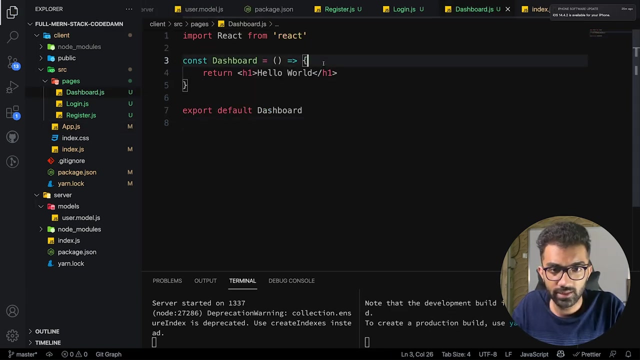 and this should also be. this should also be dashboard. and one more thing, which is we can just name this as login, okay, also, let's just go ahead and define the route for this real quick. so dashboard, dashboard and import dashboard like this. and one more thing that you can do is inside. 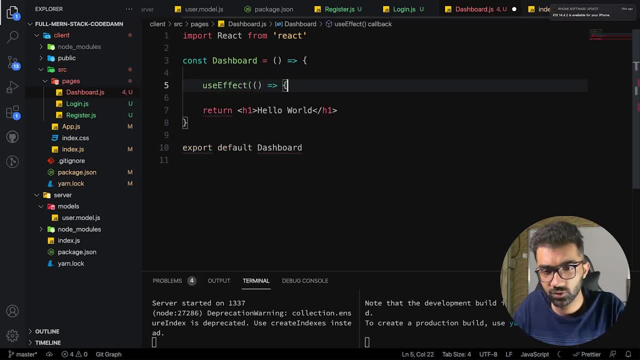 dashboard we need to verify the user is logged in, right? so we're going to be writing a use effect and we're going to be saying that, hey, if we are not able to find that jwt token with us- so i'm just going to say jwt from json token, because we also installed it here- i can say, uh, my token is: 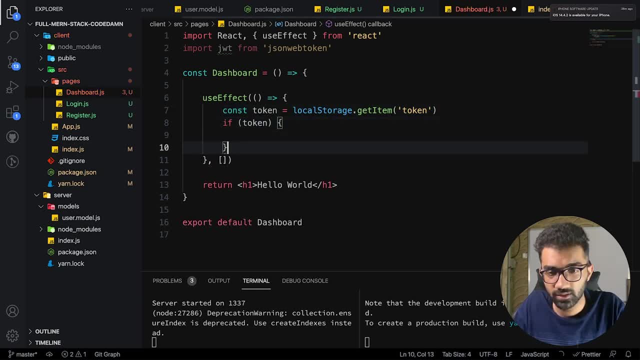 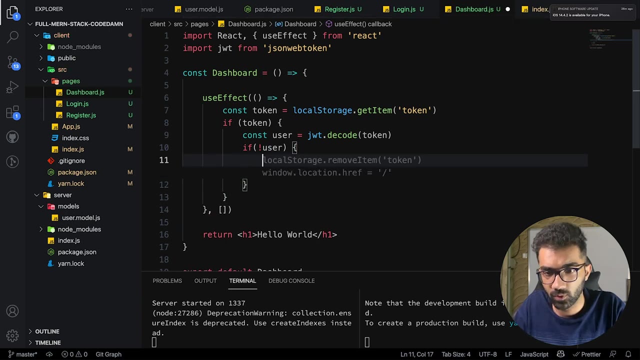 first of all, we get it from local storage, which again something we have to see. if we have token, then user is jwtdecode token, which is like copilot is doing all this stuff, and we can say: if user does not exist, that means something went wrong. uh, yeah, i mean this kind of works right, which? 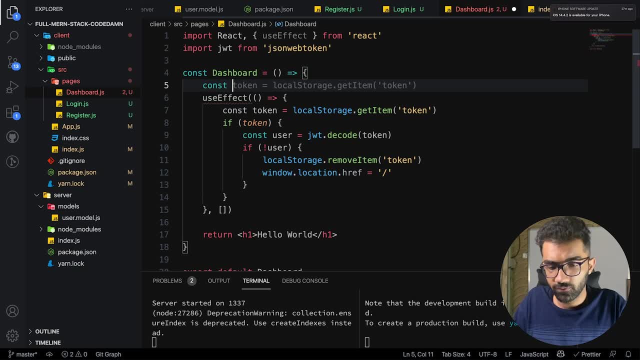 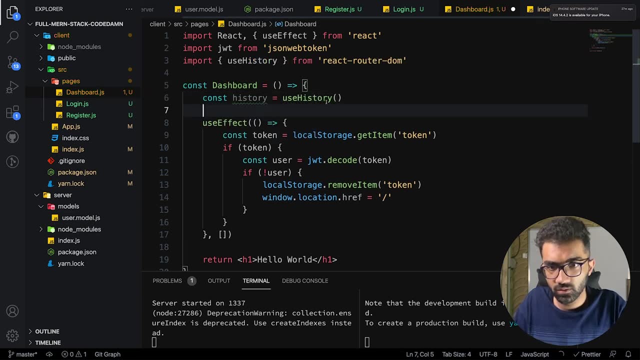 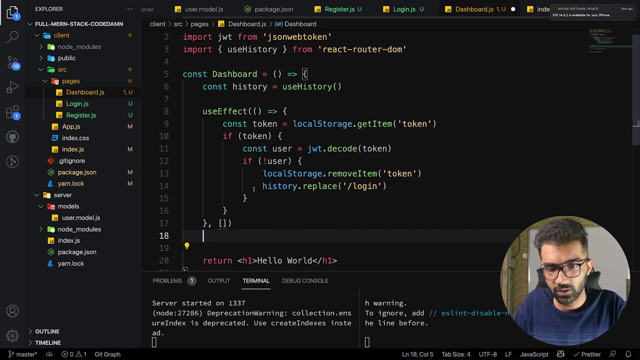 copilot is writing. instead, what we can do is make use of use history hook from react router, use history, and once we do that, you will be able to see that we can just say history dot he place and login right here. so this performs a check. and another check which we need to do, in fact, is that if user does not exist, if user does exist, 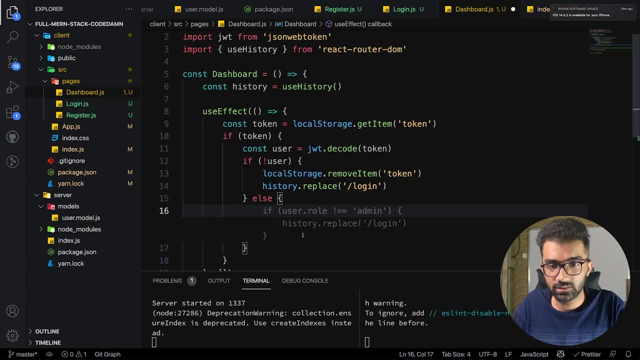 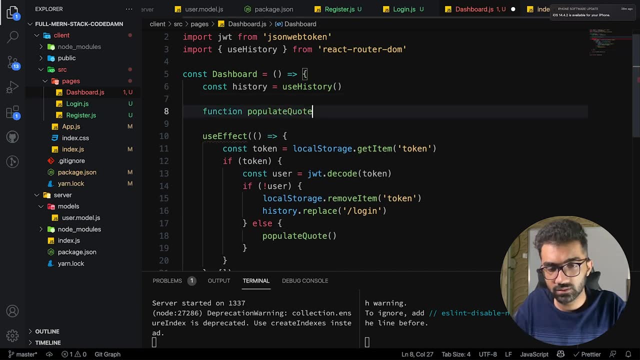 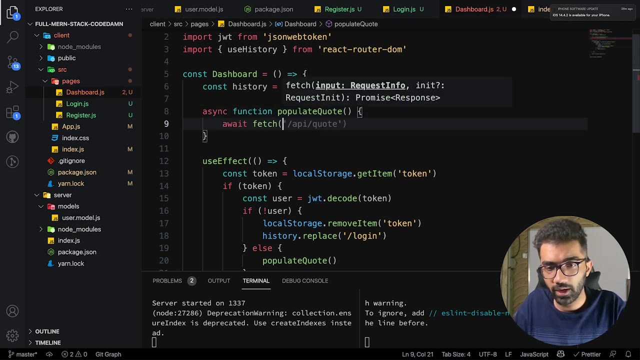 what we want to do is perform this request to the backend and see if we can populate the code, so we can just say: populate quote right here now. what this will do is that this will be a function like this, which could be async, and what we can do is just say: await fetch api slash code. 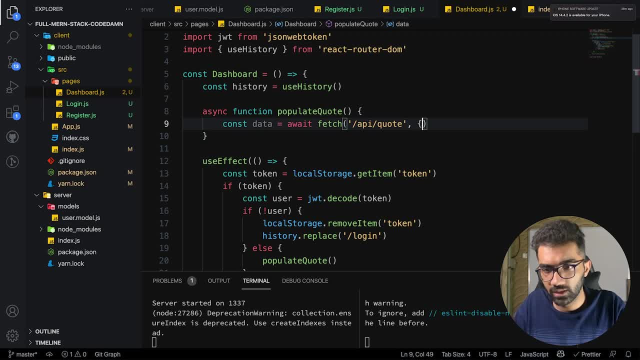 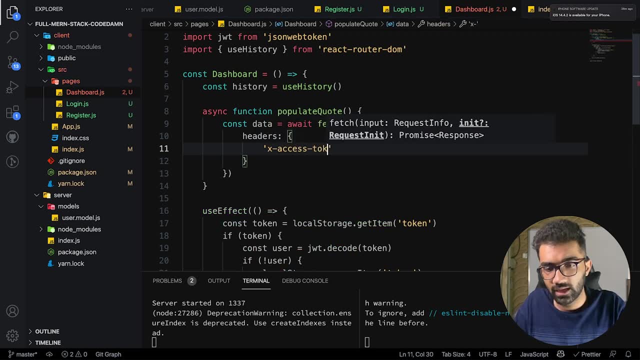 is data is equal to APS slash code and we can just say: headers: we are just including this in the headers X- access token instead of cookies, and we can just say: you know what we did here: local storage dot get item of token. now a quick recap of what we are doing here is that before, after, just after this? 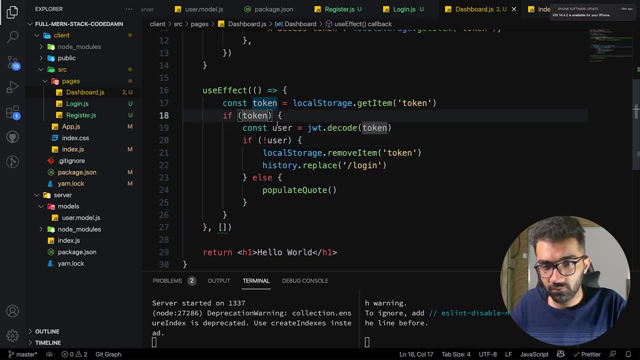 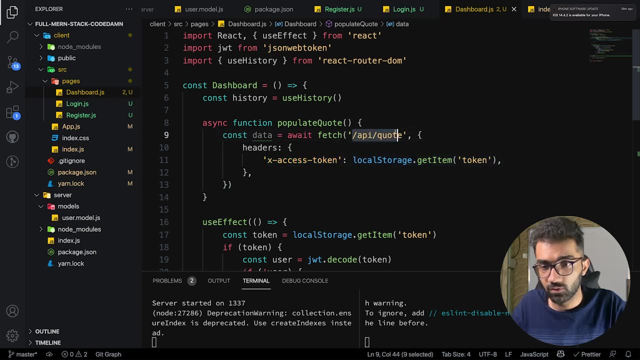 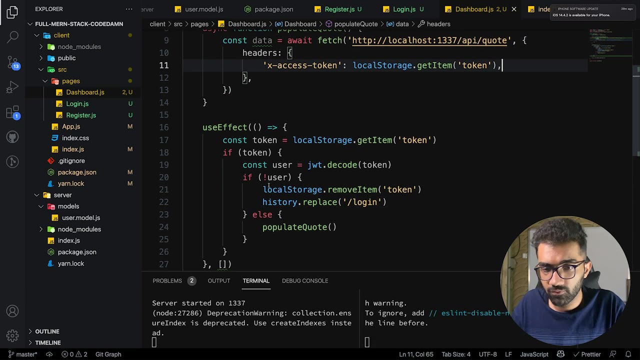 component mounts. we run this use effect only once. if we found the token, that's well and good. you know, that's well and good. we just populate the code by giving an HTTP request to slash API slash code, which should be actually localhost 1337 slash API slash code. if not, then we redirect the user to the history dot. 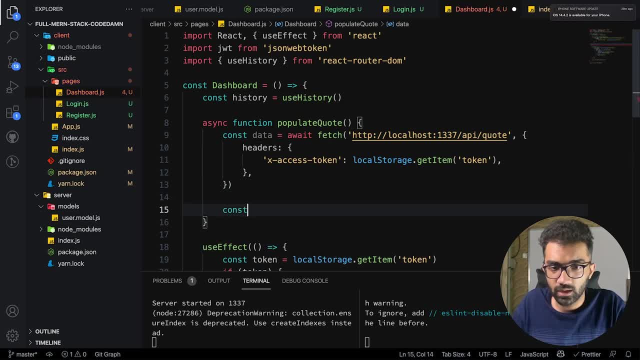 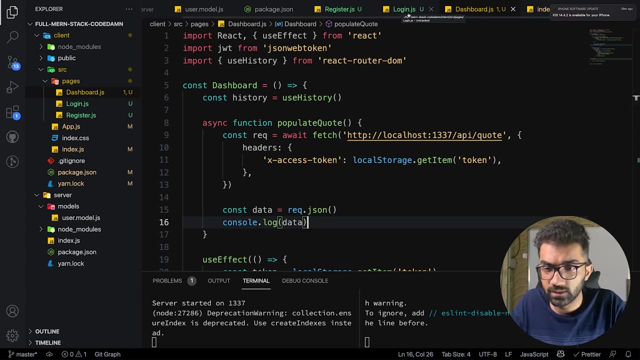 replace thing of login, right, okay. so once we have the code with us, what we can say this could be just request, and data is request dot JSON. we can just say console log of data right now and just to see what we are getting right. so the next thing we should want to do is 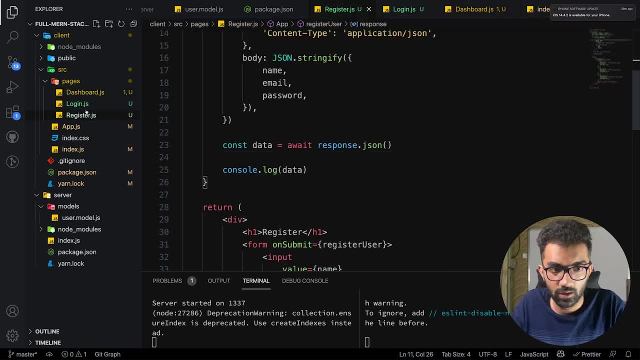 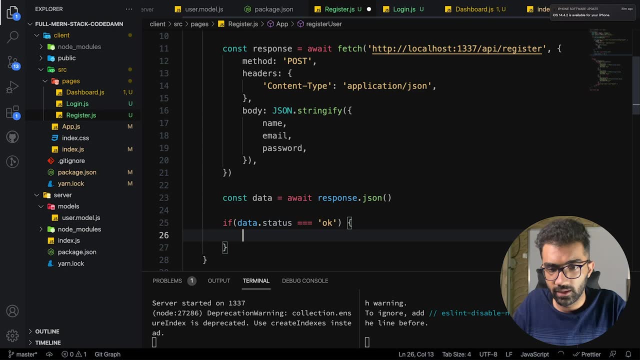 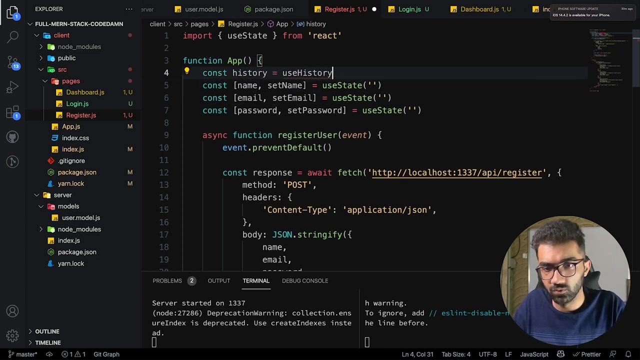 right inside of our register page. we also want to say: if data dot status is okay, then I just navigate it to the login page. right, so I can just say history dot push login, not push state, but actually push. and this history right here is again a hook which is provided by use. 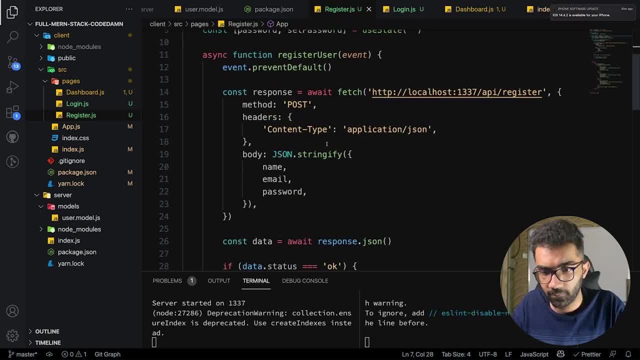 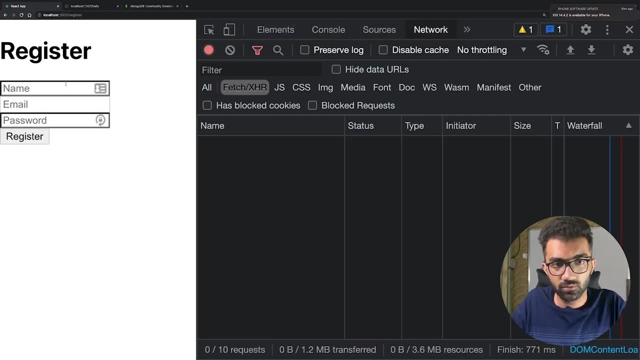 react router down library right, all right. so so far what we have is: if I go ahead and create another account, let's say mayhole, mayhole at the rate code downcom and the same password, we get redirected to the login page and if I have this as the login thing, you can see I get login successful. click on ok and I. 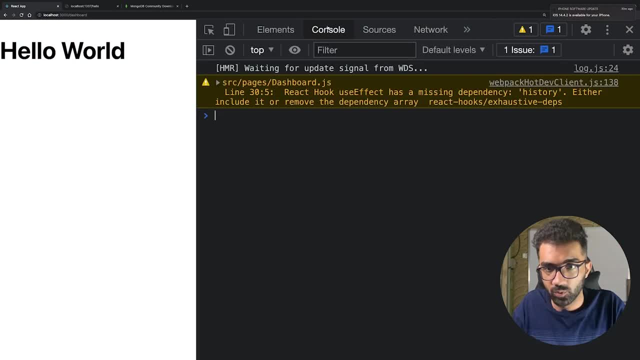 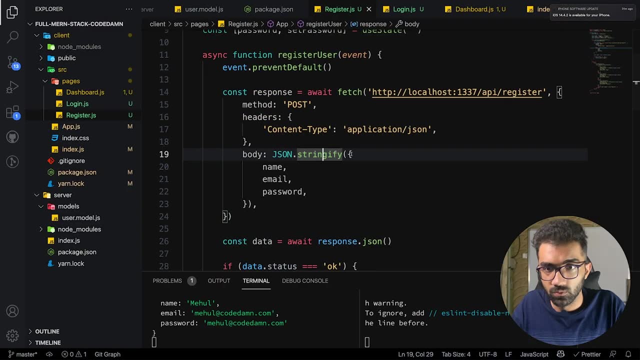 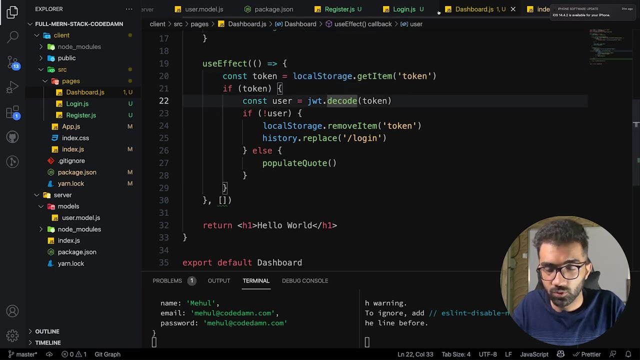 get redirected to slash dashboard, which just saves me hello world. at the moment, right and inside of console, we see nothing happening instead of Netflix also nothing happening. so that is that is probably not good, because, yeah, that nothing happens because we don't have the token store. so what we want to do at 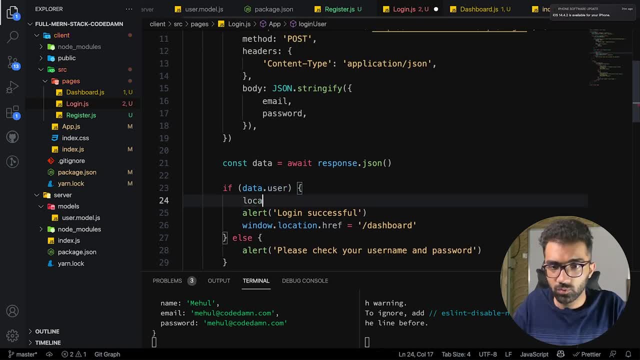 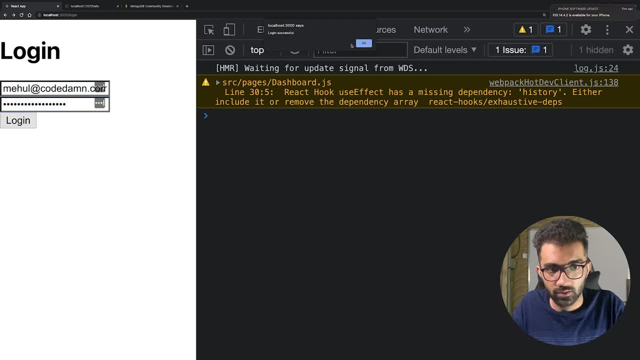 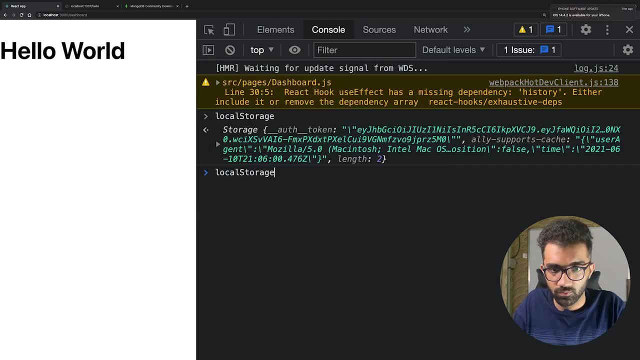 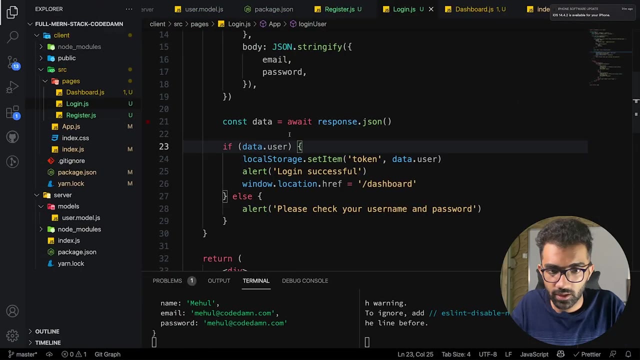 again. so let's just perform the login one more time and click login, and now you would be able to see that our local storage includes not this one. actually this is from some other project, but if i do a locals, let's just go ahead and do it one more time and let's say login. 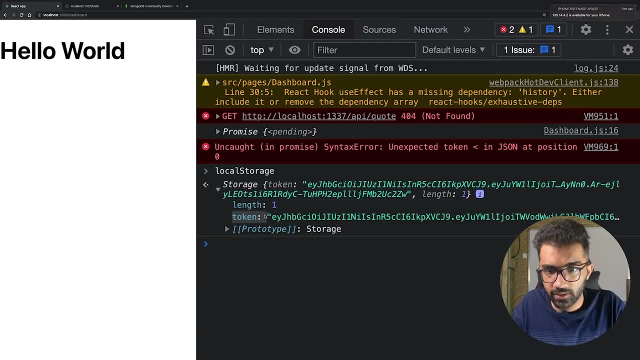 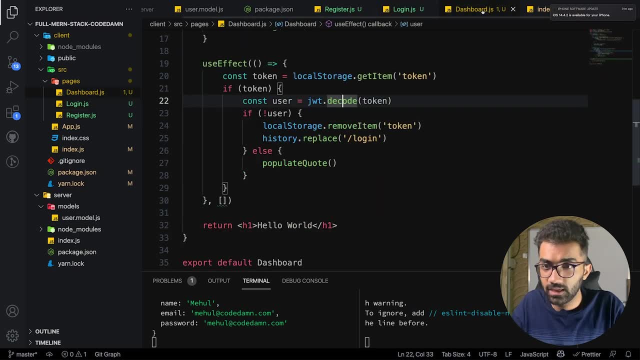 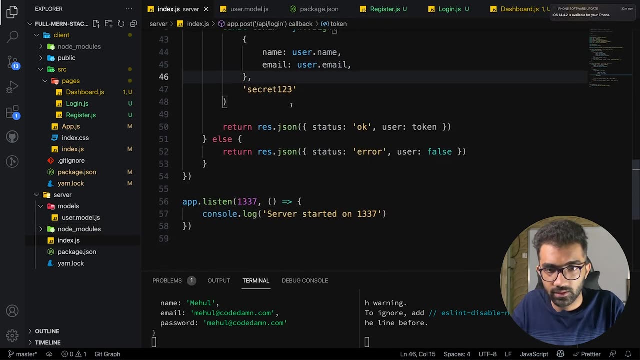 login successful and you can see right here we have our token in place right, and you can also see we get an error that 404 not found. so let's just go ahead and create this api now at the back end. so what i'm going to do is go to my indexjs again and create a new endpoint and remember this. 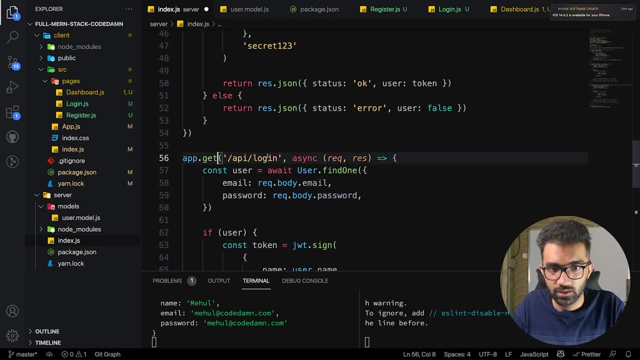 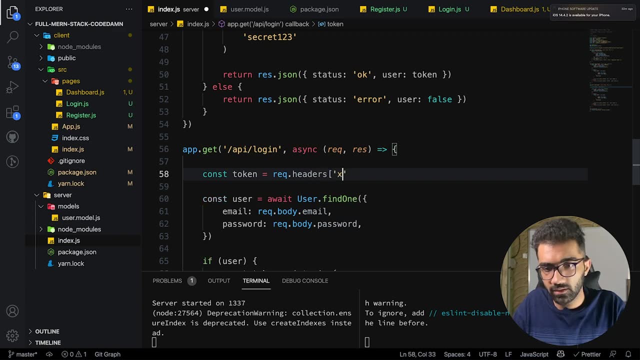 endpoint was get, it was not post, so we will just keep it get like this. but what i'll do is i'll say my token first of all, is requestheaders x- access token right, because we want to perform authentication first. so i'm gonna say const decoded is jwtverify, and then token, and then secret one, two, three which 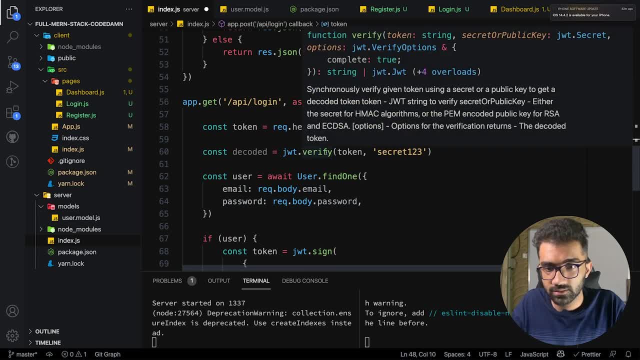 was the actual secret which i wrote right. this just verifies synchronously. you can also pass this as a callback if you would like. uh, synchronously this verifies if your token is correct or not right, and i think this throws you an error. i'm not sure if this throws an error or 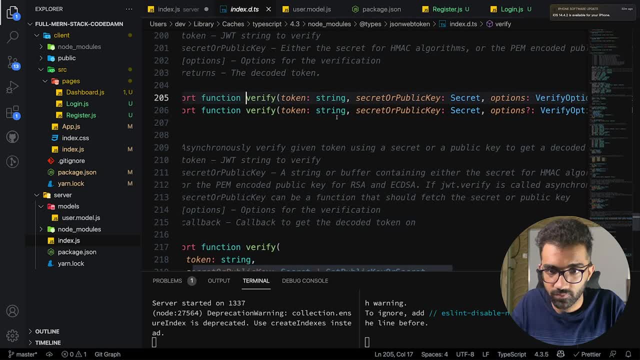 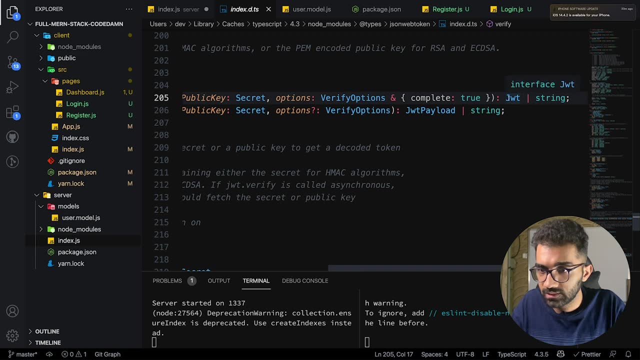 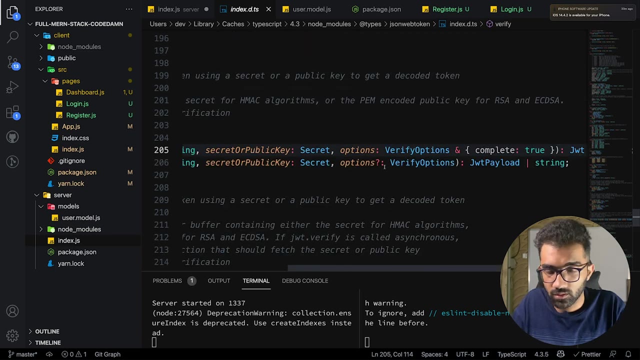 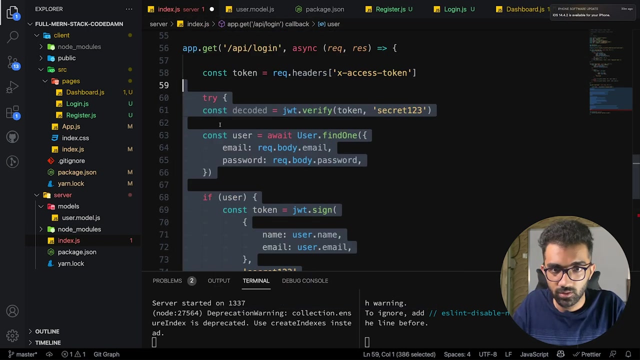 just returns a. you know returns undefined, so it just it says that it returns you jwt or string, so it does not return you a null value. yeah, so i'm hoping that this throws you an error anyway. so if this does throw you an error, what you want to do is try catch this block. and if we have a decoded token, what? 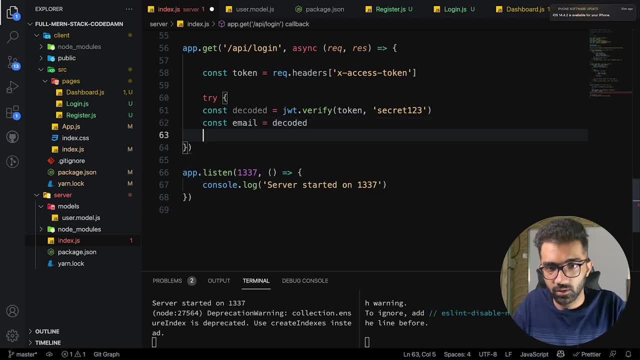 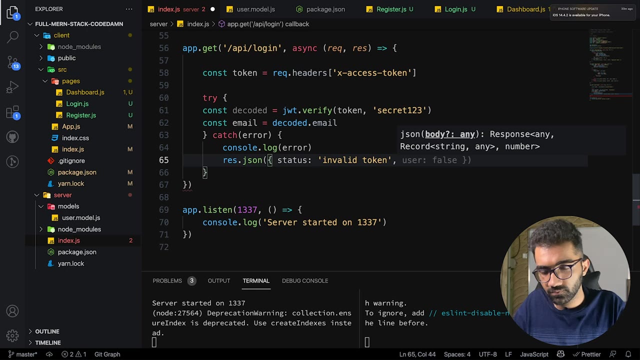 i want to do is the email should be decodedemail right, and what i want to do inside catch. i want to say that you know consolelog error first and then riskchason status invalid token. or you know status basically error. let's keep the format. same error is invalid token. 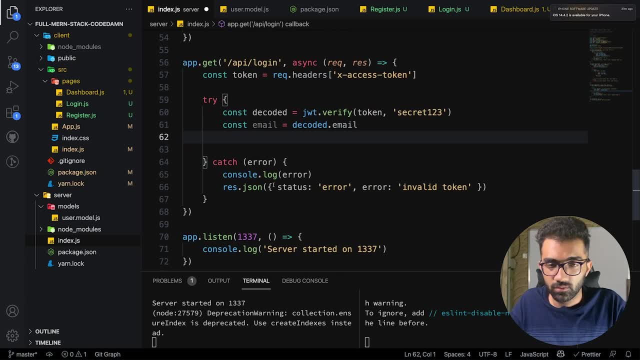 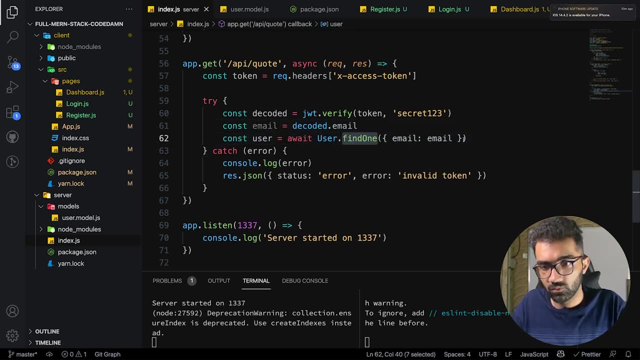 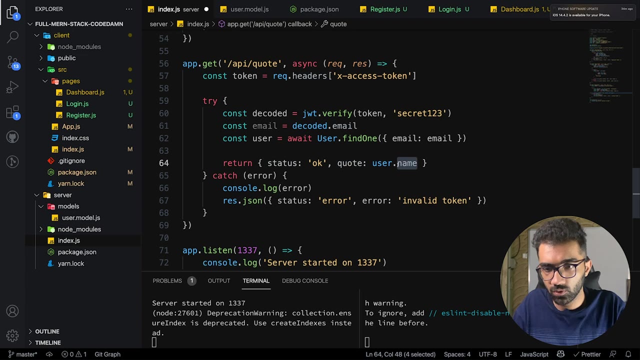 right, but right here. okay, yeah, but right here inside api code. once we have the email, we can get the user and once we have the user, we can get the code. can say: return status: okay, user, not user, but code. could be usercode right here which is inside our 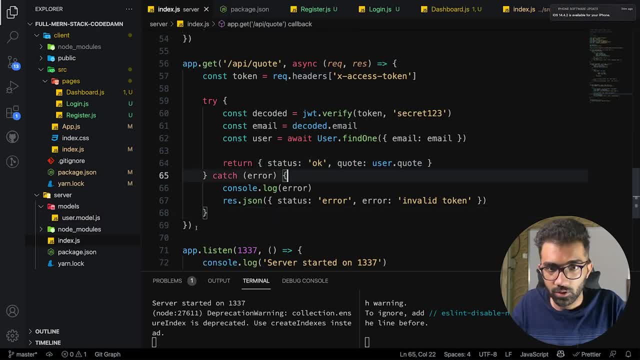 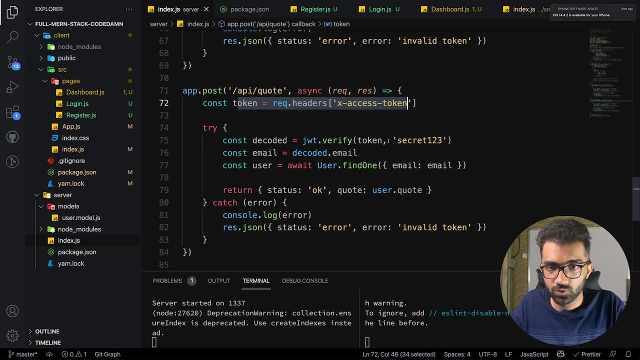 model right. so that's fine, that will work. but you will see that we also need to create the code right or add the code. so what we can do is also create a post route which, pretty much again, is authenticated. we verify the token, we get the email, but the only thing which we say here is update one. 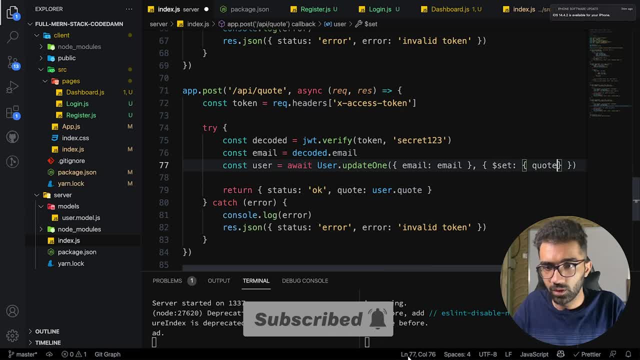 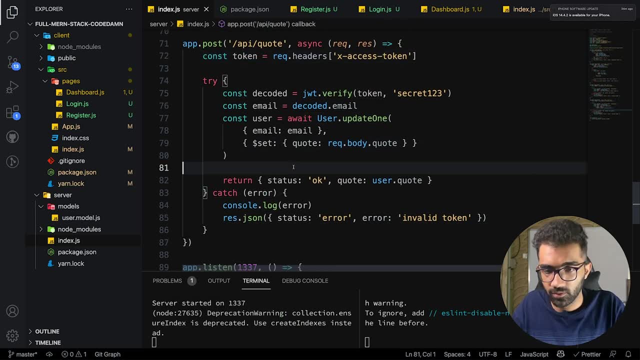 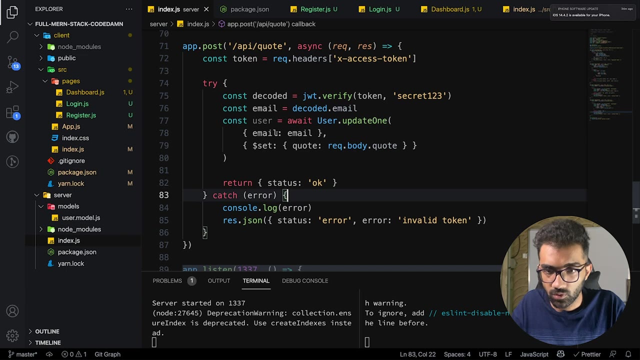 email this and set the code to be whatever we passed, right, so requestbodycode, which will destruct from here um status sake. okay, and data is invalid in other case. awesome. so i think that is pretty much all we need from the back end part. yeah, it should be. 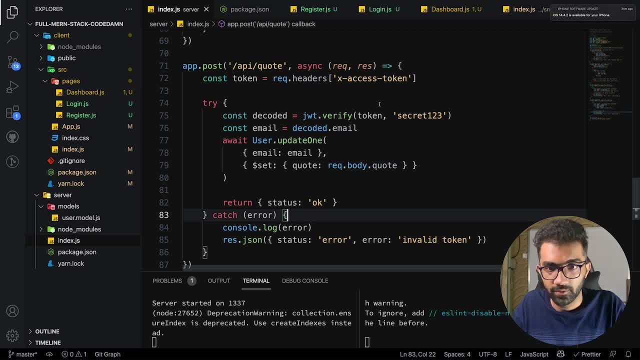 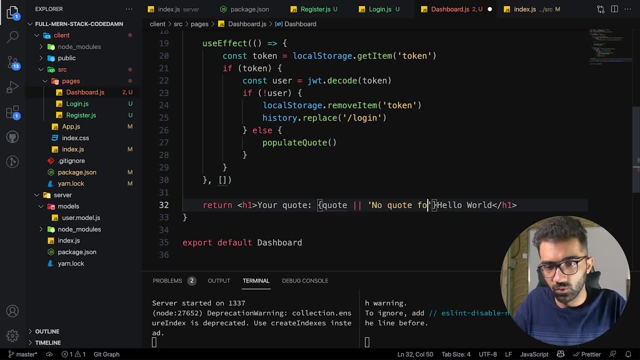 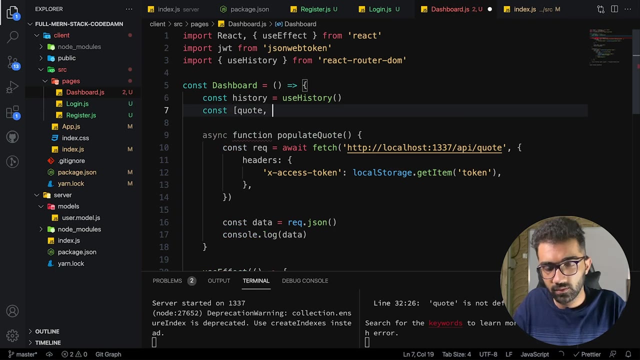 probably working just fine. let's see it how we can implement this on front end. okay, so the first thing we want to do is you want to say this is your code and let's say this is your code, this code or no code found something like this right, and what i can do is make this code as a 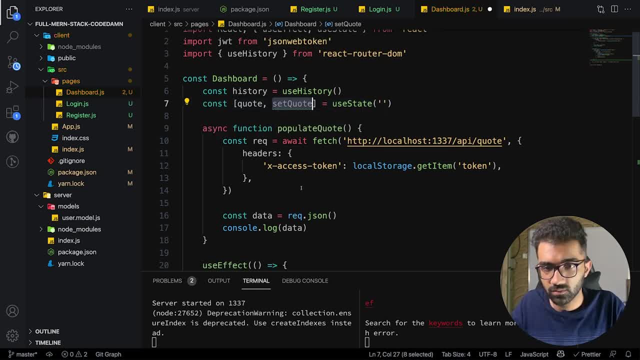 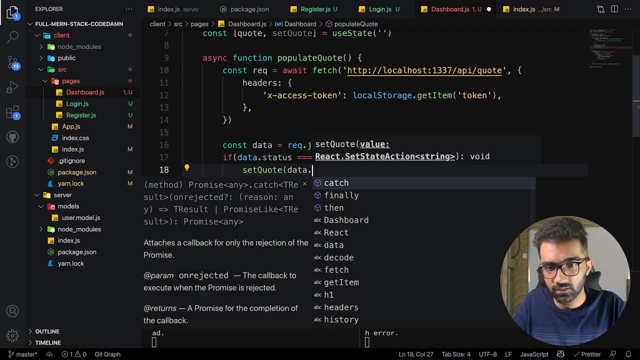 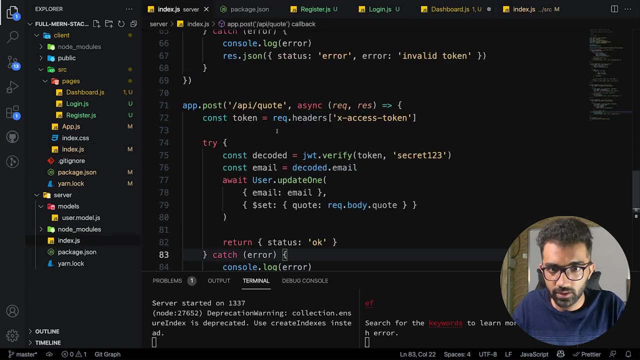 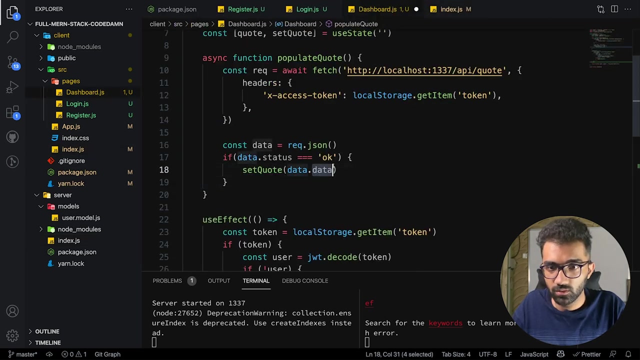 state variable which will help us set this dynamically. so once we have the data, i can save. datastatus is okay. then i just want to set the code to datadata. i guess i think that's what we return, right? let's go to index. we can see slash api, slash code hit, ok and then the code okay. so datacode, not datadata. 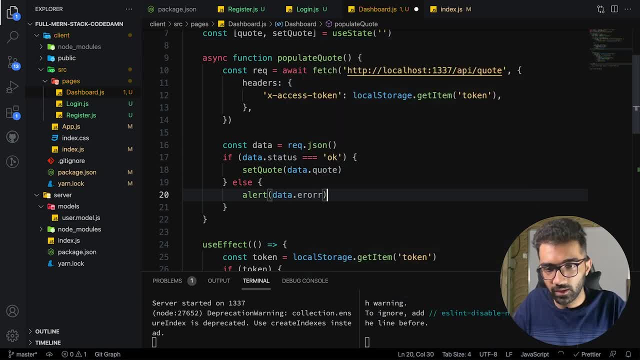 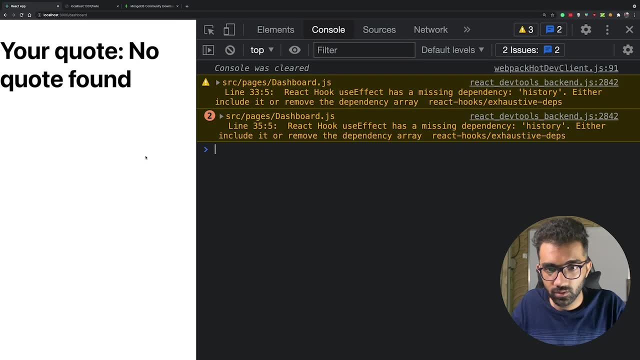 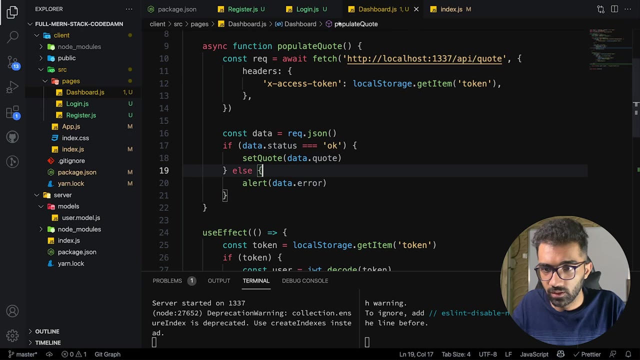 else. i just want to say: alert dataerror. right, all right. so here we have the basic setup for at least displaying the code, and right here you can see the moment i refresh it. we get no code found, because, fair enough. um, okay, actually we are not returning anything and the 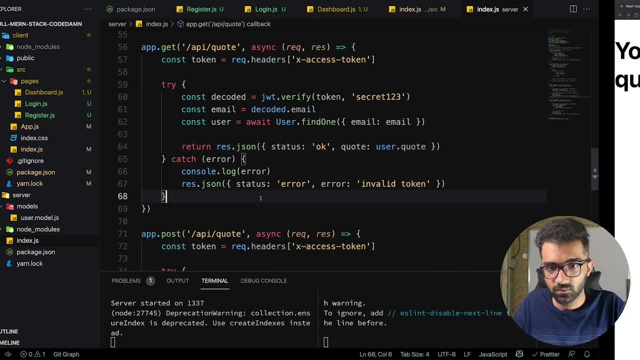 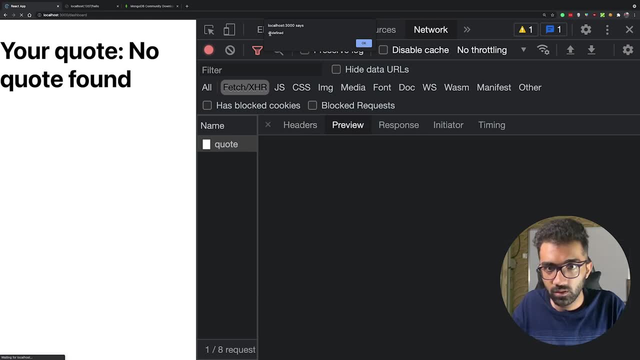 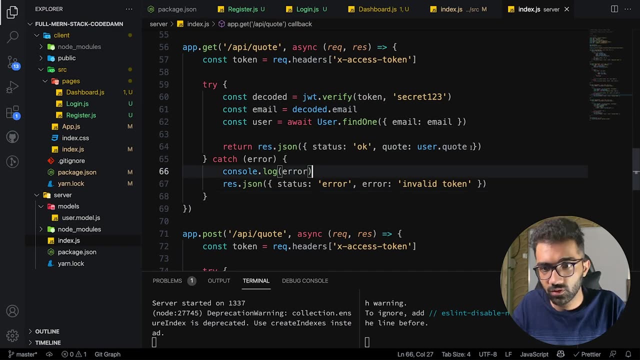 reason for that is probably we missed restjson. okay, now if i refresh this, you're gonna see that again we get no code found because, okay, it saves me undefined as the alert. if i alert, you can say: see, we just get status. okay. the reason for that is because usercode is undefined and undefined. 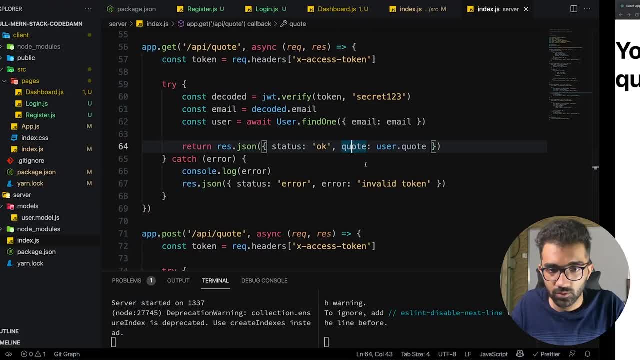 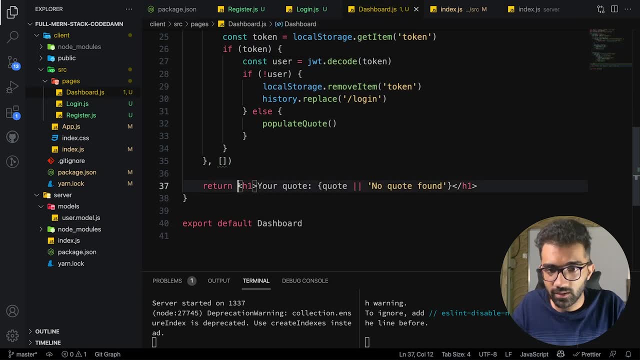 is not json serializable, so json just removes this. so what we want to do is actually provide the user an interface to set the code as well. the way we can do that is we can wrap this whole thing inside of a div and create an input field, or rather a form. let's say input type, text place. 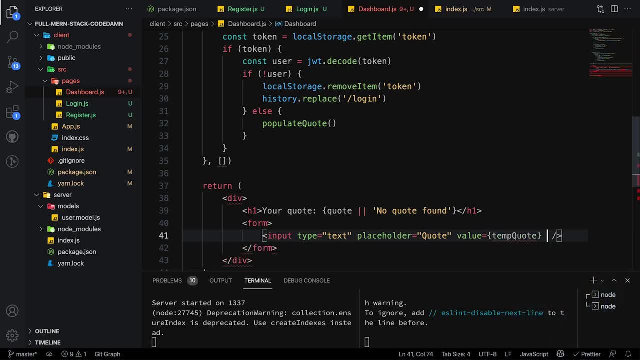 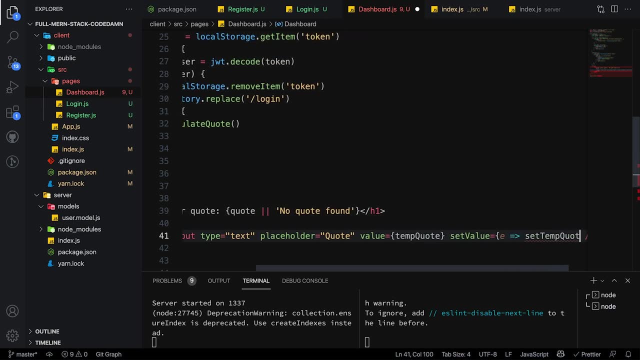 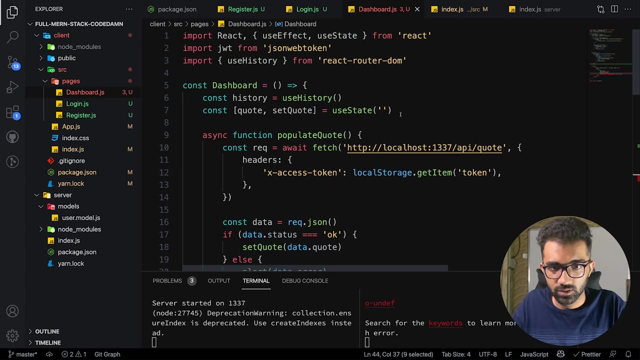 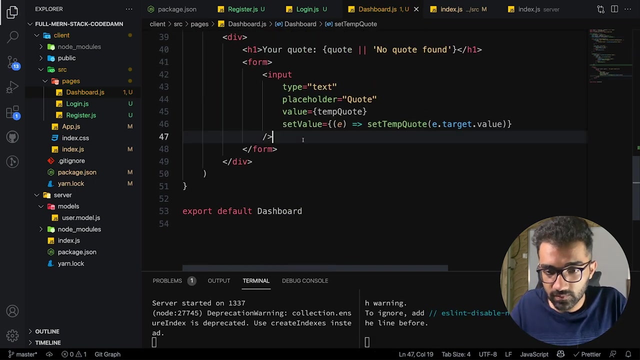 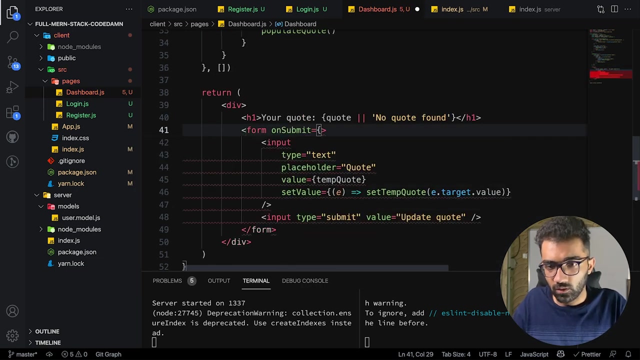 on the code value is empty. report set value is, you know, e set m code, v dot, target dot value, basic state management stuff, and you can just go ahead and create this like this. i also added a submit button and i also am adding a handler to this which is update. 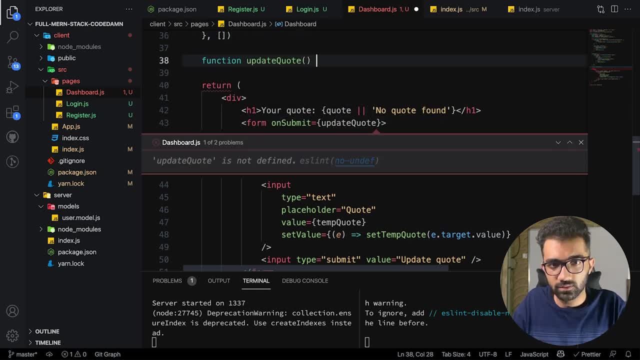 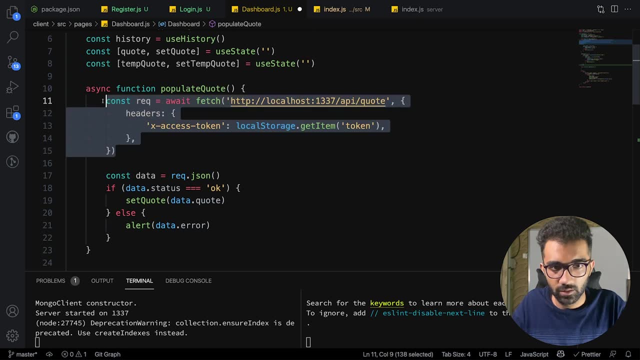 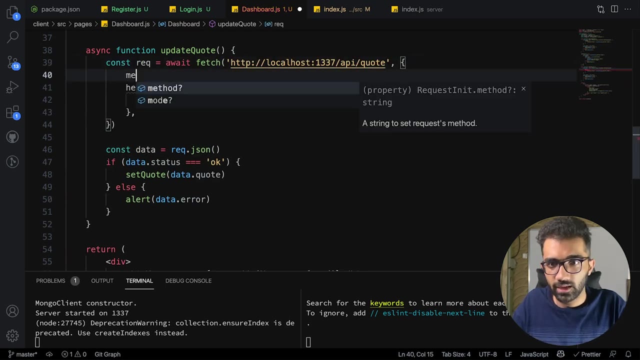 code. what this function will do is it will just send the same update call, but this time to update the backend, right? so i'm just gonna say the same thing right here as populate, but instead of the get request, we're going to be performing post request and headers. 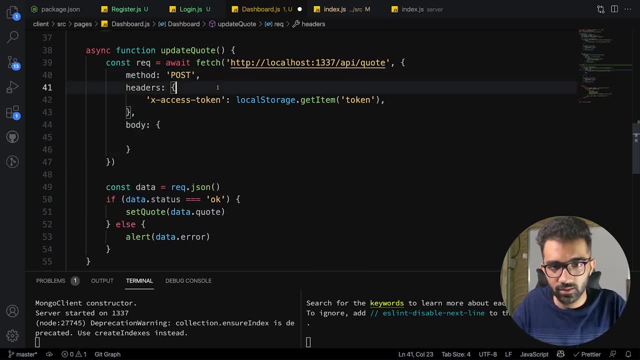 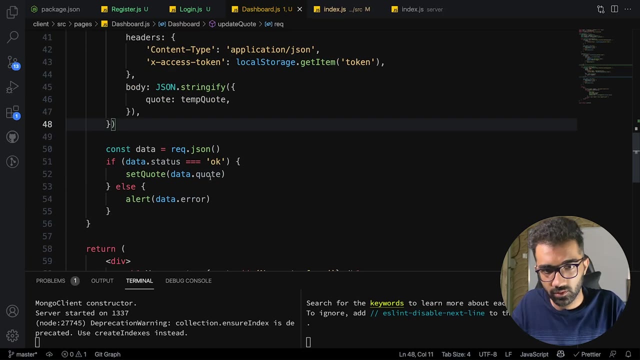 would be same. there would be one more body thing right here and there would be a content type header here as well, application json, and the body would be jsonstringify- the following thing, which is code as m code right there. and the final thing which we can do is, i mean, we already have the 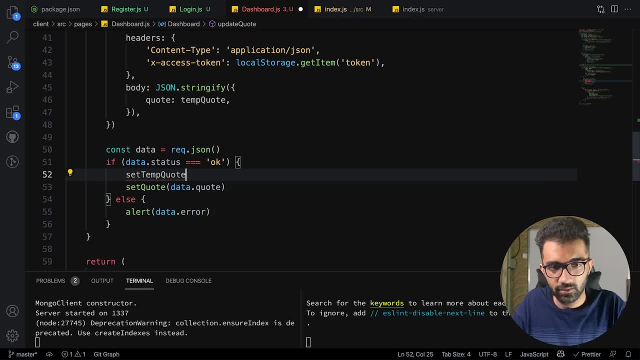 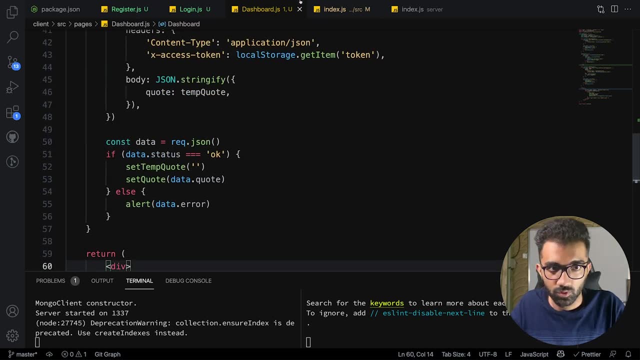 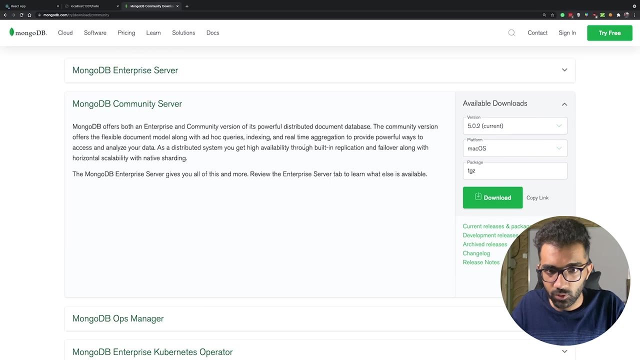 set code thing. we can also say set m code as md and that will be it, i guess, because we already have the back end ready on the server side. all right. so if everything is fine, i do believe this application should just work out of the box now. so 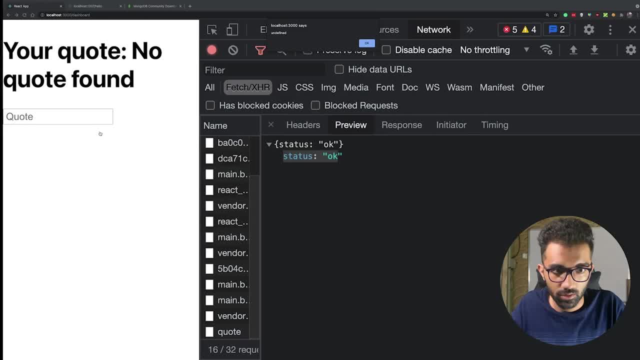 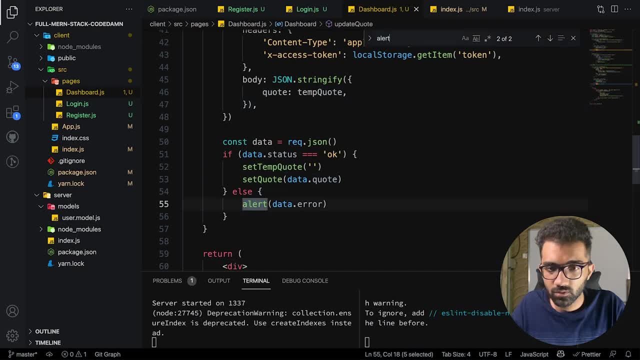 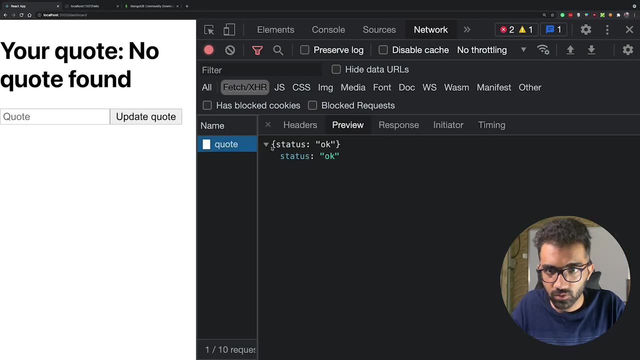 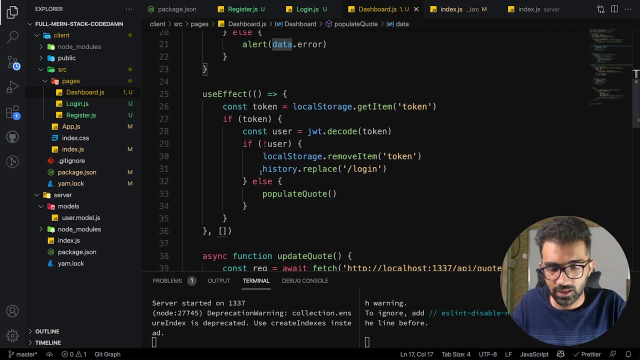 or maybe not, because we are missing uh input button, i guess, or was it just a refresh away? yeah, we have an alert of some sorts, not sure why, so it's of populate code for some reason. yeah, and that is because we are not using await on requestjson, so we just have a promise here and that should not. 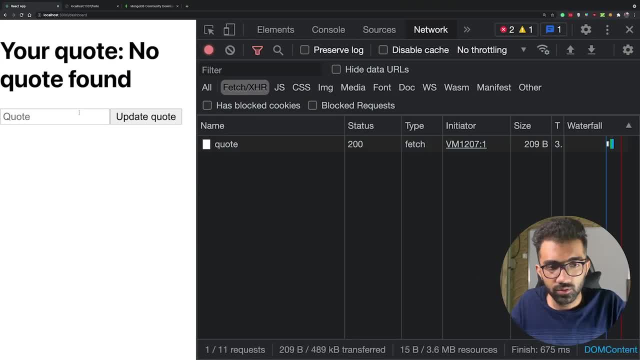 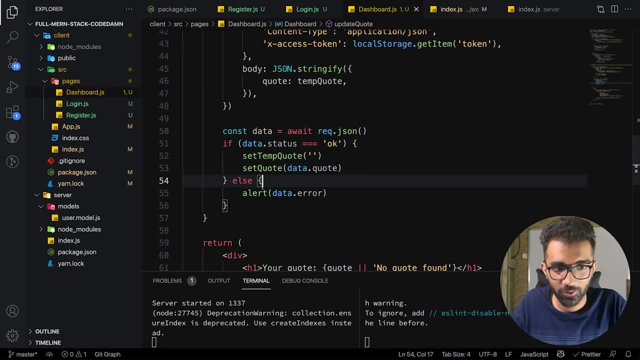 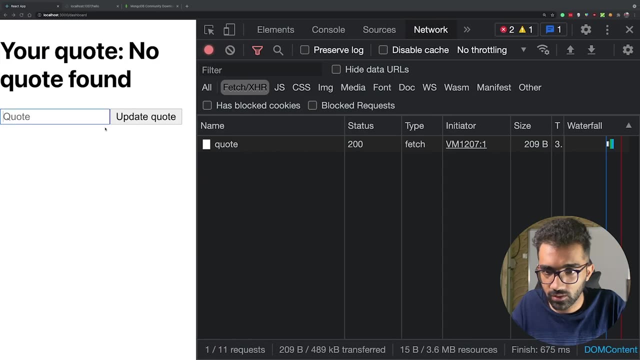 be here as well. there we go, all right. so now it should work. fine if i go ahead and write a quote, something like: work today or yeah, okay, so our code is not even working. m code and set m code, p dot, target, dot value. not sure if it was not working, or oh, this is not set. 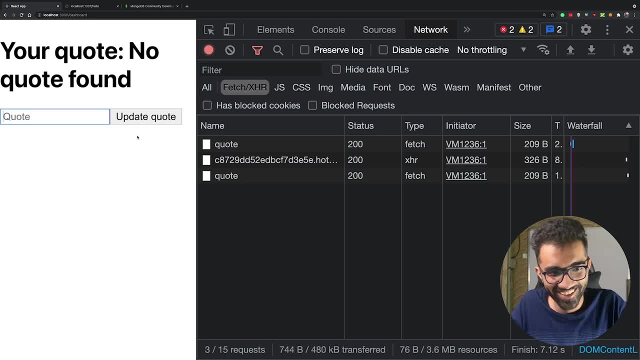 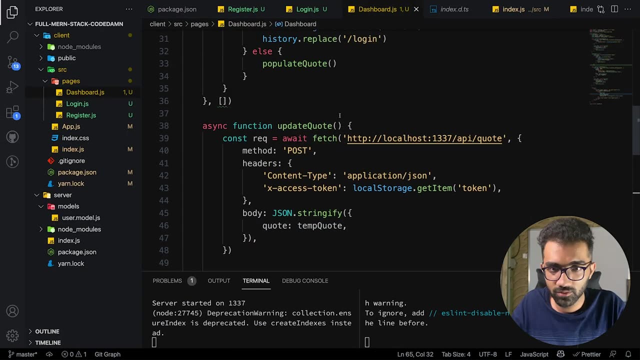 value on change. i think i should really go to bed. but anyway, let's complete this video work today, party later. i don't know like i just randomly created this and if i click on update code, nothing happens, because we need another final thing, which is to prevent this event from refreshing. 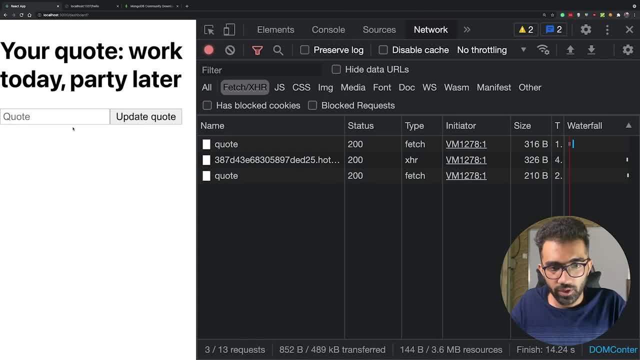 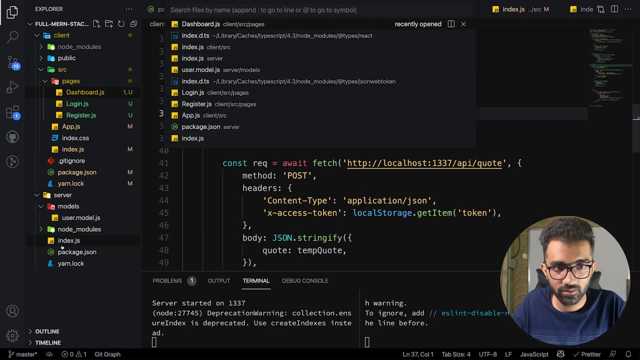 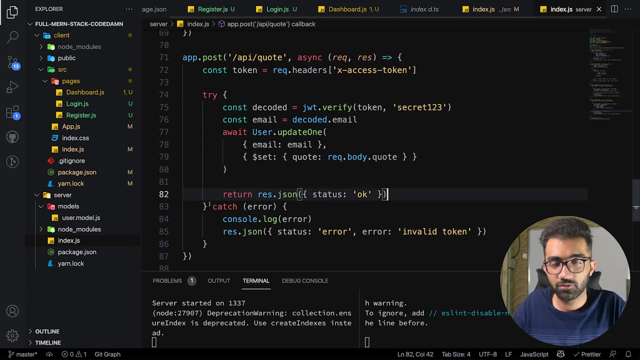 the page. all right, let's hope this works now. work today party later update: we send a code request and we have another problem on this page, problem on backend, I guess, because I think we are still. yeah, I mean, I'm always in the GraphQL based mode, right, where you just return the response and 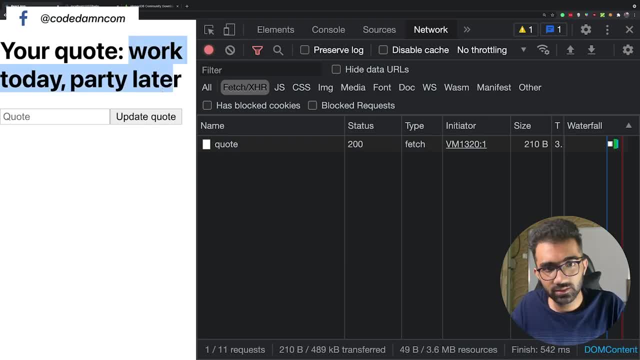 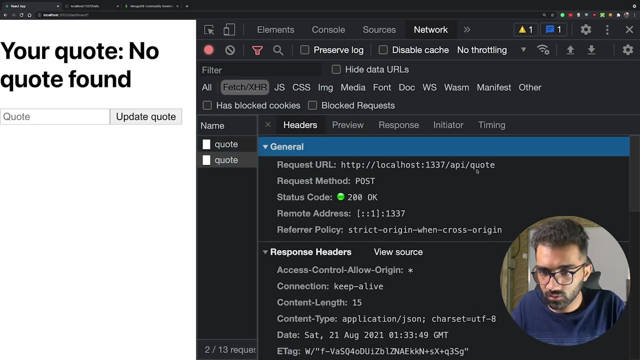 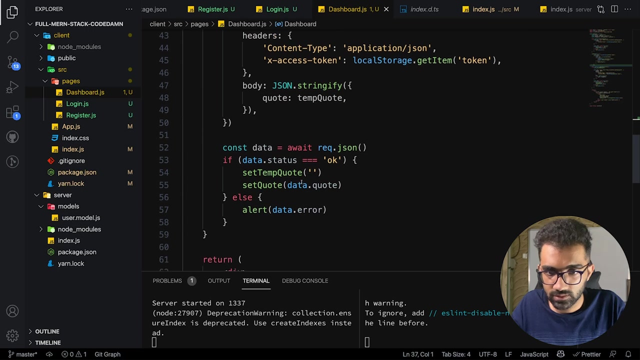 it sends us JSON anyway, so I refresh. now you can see our code is updated. I mean, we know that it works, but if I try to add new code here, updated code, okay, we get no code found. that is because of why is that? because of: let's see inside. 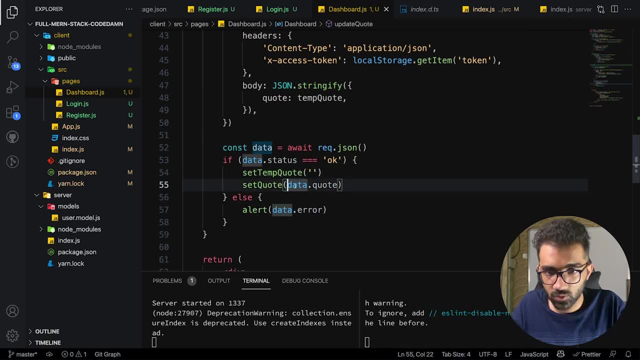 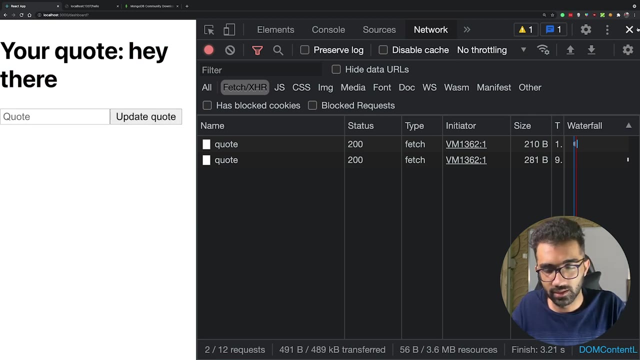 update code. we set temp code as that and set code as no. this could be just temp code, right? because we just sent the temp code, so we know that this will be the updated code. so refresh, hey there, update code. and you see that we get, hey there. 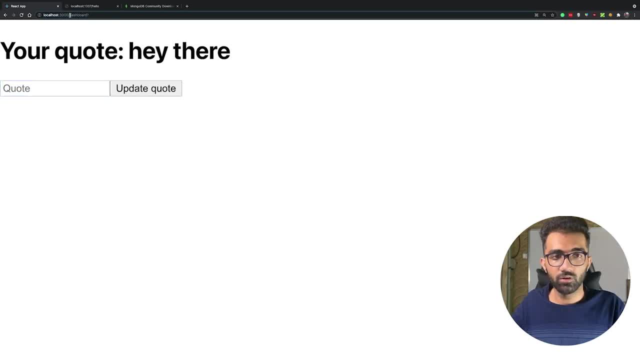 as the code. so I mean I think this will work fine now if I go ahead and create a new account, if I go to register mehul2 mehul2 at the ratecodedowncom and use the same password, register and login again. login successful- hey, I am mehul2. 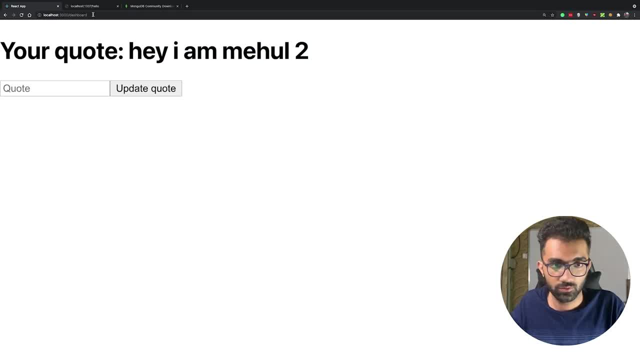 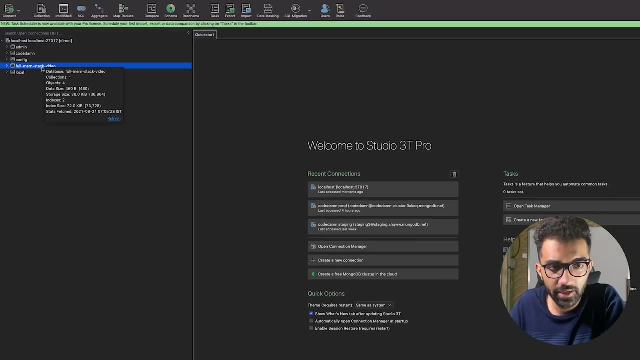 update the code and we get: hey, I am mehul2. that's awesome now if I go ahead and login again, but with my original username and password, hit login, login, login successful. we still have. hey, there code right and inside of the database. when we see and the database, you can see that we have a full mall. 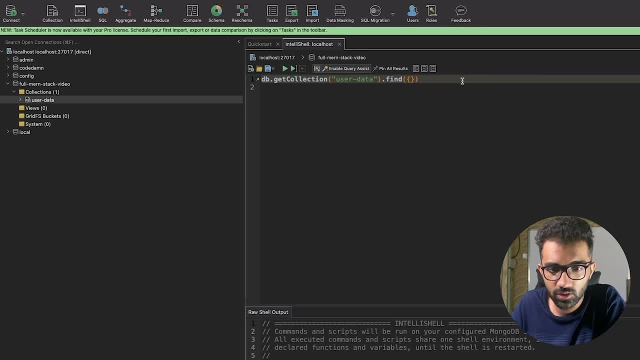 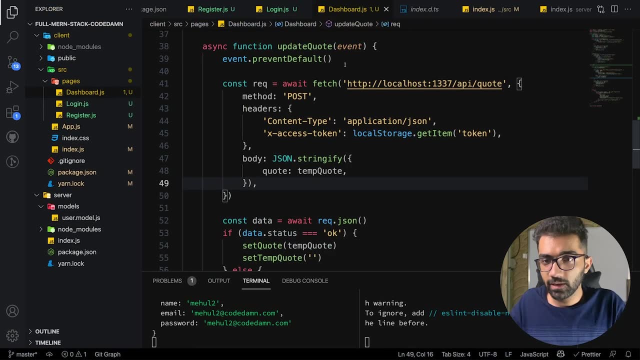 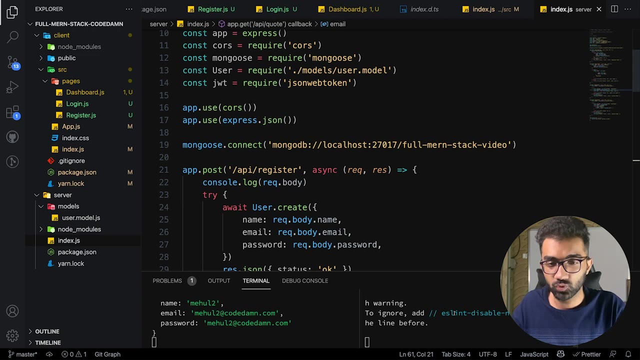 stack database and inside that we have a user data collection where we have all these records which we have created, right with the code values. one final thing I want to just tell you before going from here is how you should store passwords, because that is, I think, a super important thing and usually people miss. 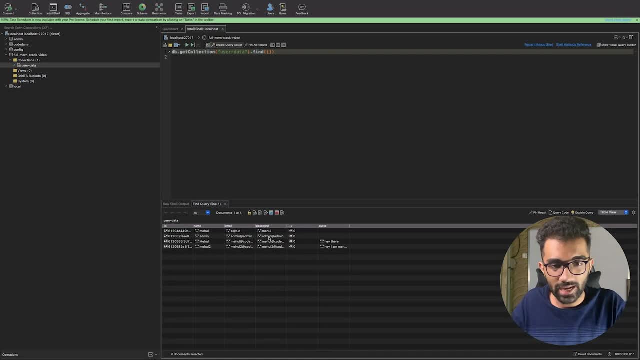 out on videos like these. Well, that's all for today, and I'm gonna sign out of this recording video today and have a great rest of my first 4 serpents next week. bye for now. So I don't want to do that. You should absolutely not store passwords in plain text like this. 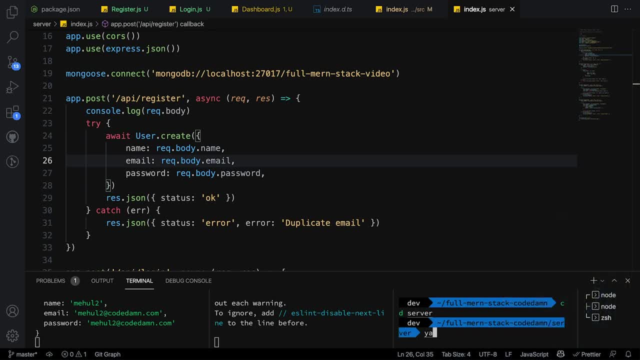 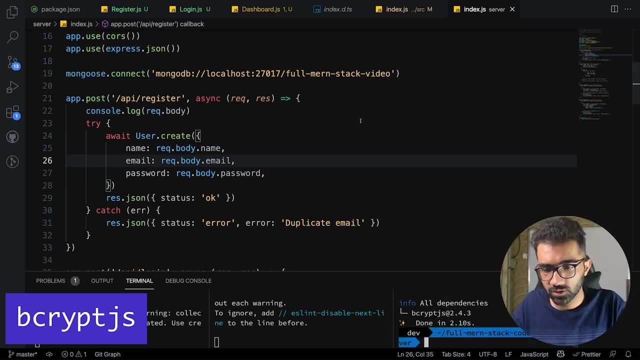 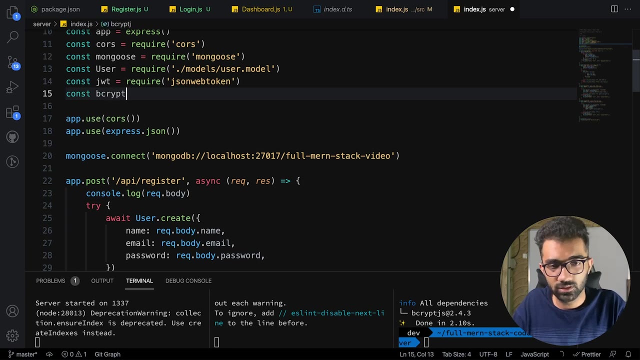 The way to store passwords is the following: go to your server folder and install a package called yarn, add bcryptjs. It could be bcrypt as well. I'm just using bcryptjs because it is. it does not install binary binaries of bcrypt, Which are native binaries, and although it's a little slower, It just works like that. 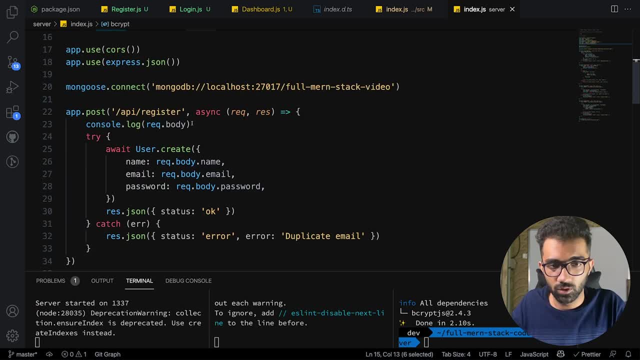 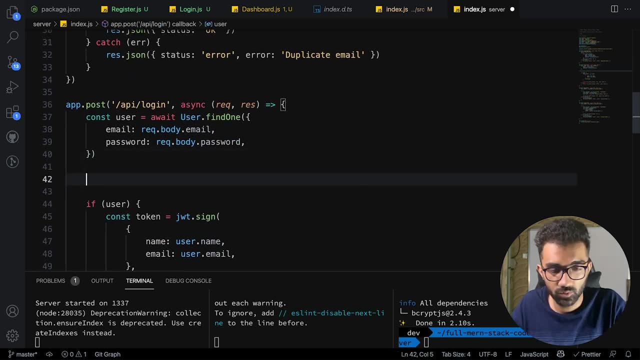 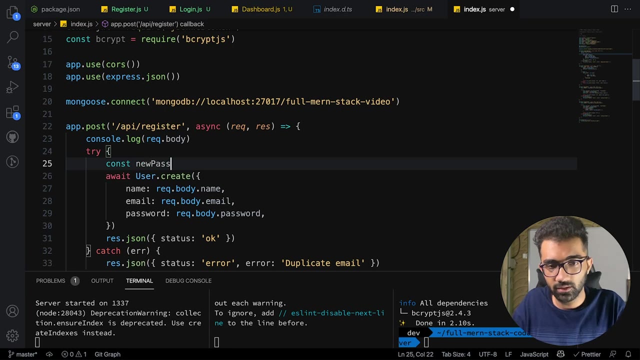 But if you're writing it for the prod, it's probably better to also consider bcrypt as the package. So bcrypt is a hashing algorithm, a hashing mechanism which can Secure your passwords by making a one-way hash of them. So what do you want to do when somebody's trying to register? is you try to create a new password? 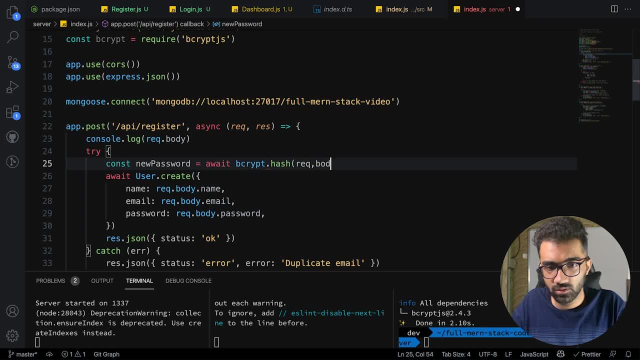 By saying: await bcrypthash requestbodypassword and give it some cycles- and usually 10 cycles are enough- and you Store the hashed password instead of the regular logged in password. right? So this is the first step. now The second step is: how do you verify this? because the moment somebody now tries to register on your app, 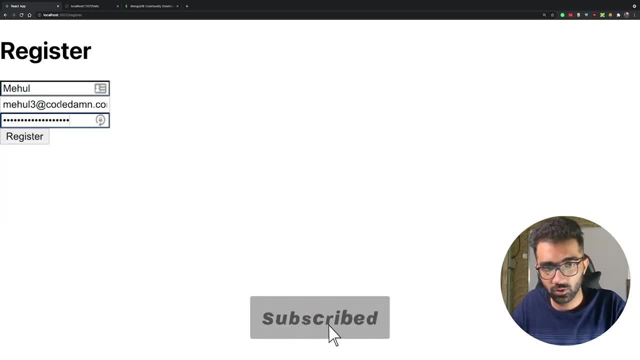 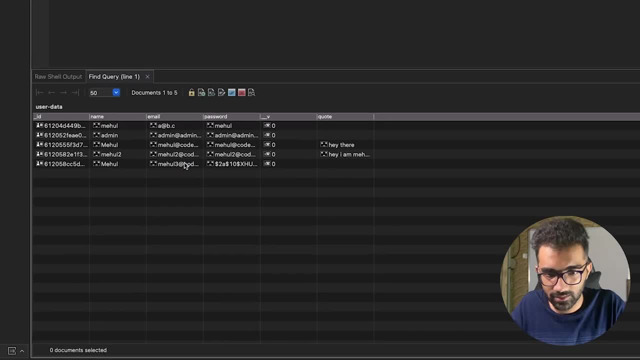 Let's say, if I try to create a mayhole- mayhole3 at the rate code downcom- And do the same thing, what you're going to see inside of database is that mayhole3 Right here Has a weird password, right, And this is a hashed version of that password.